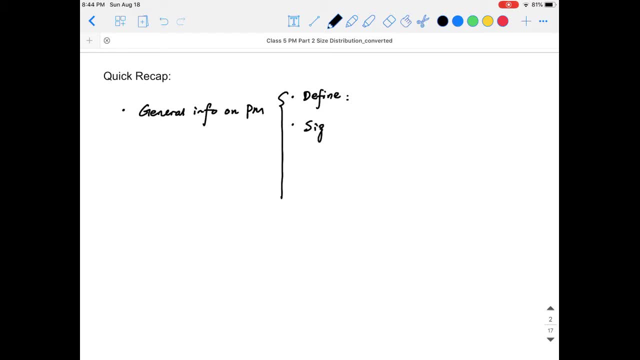 right. We also talked about the significance of PM, which includes the impact on human health, include the impact on the climate, but by both direct and indirect effect of the particles on the climate And also it could pose an impact through the formation of functional nanoparticles. 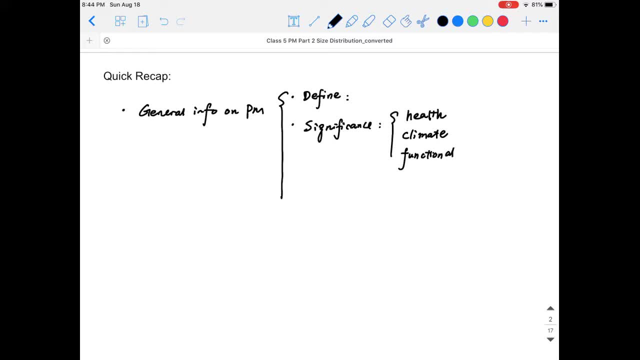 or nanomaterials. Okay, so we also talked about the source of the PM, mainly about how they're being formed, And there are two ways of the formation. One is top-down, which is generally by separating or disassembling the larger objects into smaller pieces, which is forming the PM, for example. 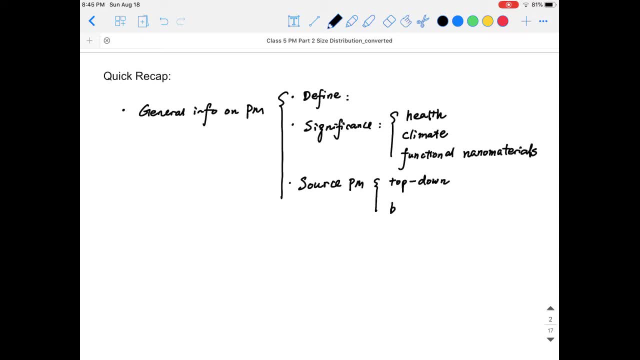 the sawing process, And also they can be generated by the bottom-up method, for example the combustion or some secondary formation of the particles. Then we also discussed about the quantification of the PM. Okay, Okay, Okay, Okay. 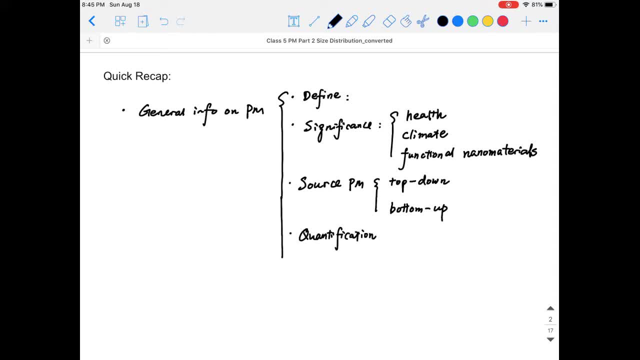 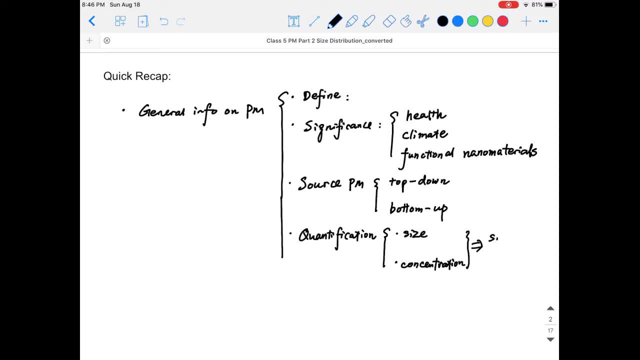 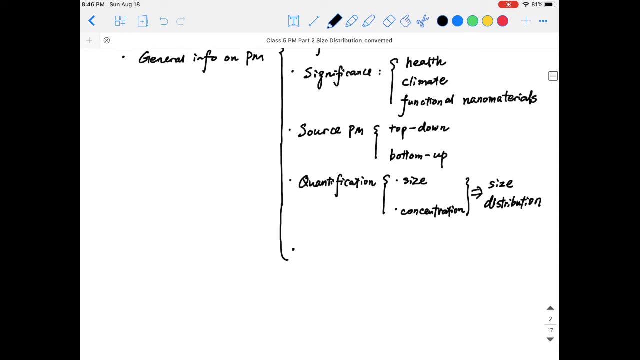 by calling or by using the size distribution system. Okay, Okay, And in this class we're going to focus on more on the size distribution And finally, I would touch a little bit about the measurement of the size distribution. right, And before midterm, we're going to have one week of time to delve more or discuss more about the measurement of the size distribution. 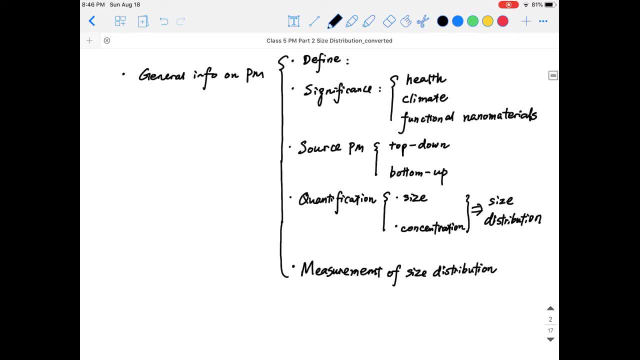 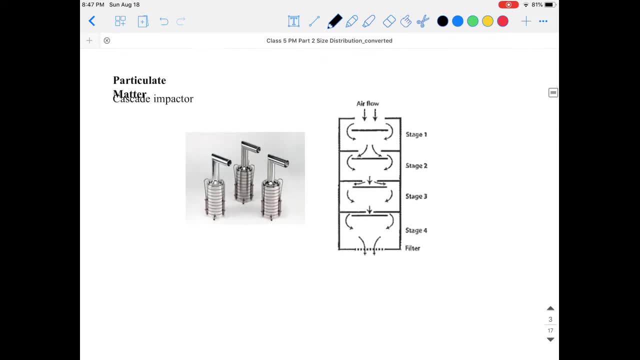 So there can be much more fancier instruments that we can use to look at the size distribution of the particles. So in this class we're going to focus The size distribution. so somehow it's not showing the correct format of the of the contents. 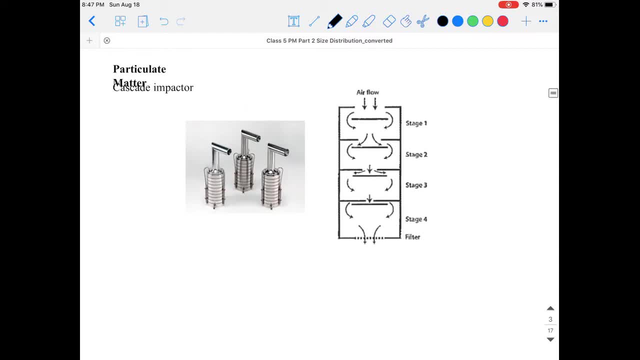 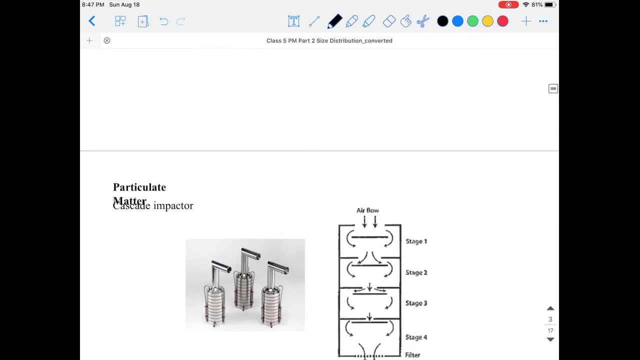 But let's just go through this, because I think I didn't put too much text into the slides. OK, so last class we talked about that. to measure the particle size distribution, or the PM size distribution, we can use a device called- that's called- Cascade Impactor. 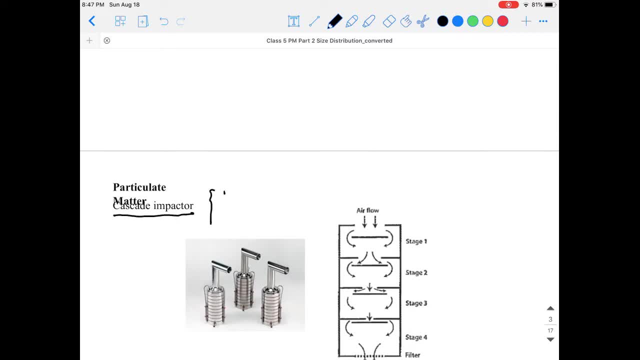 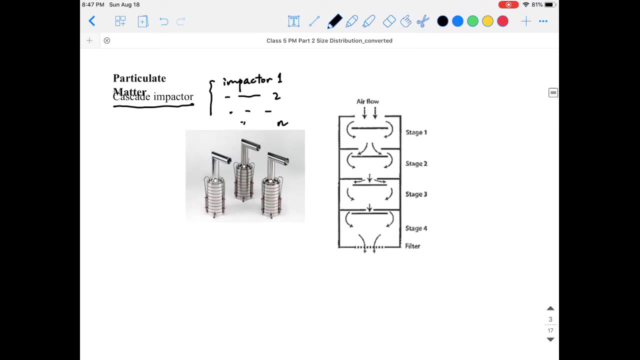 So basically it's composed of a series of impactors. So it's more. make it more clear. Let's say impactor one, impactor two and impactor n. So basically it's showing on this side here, OK, so. 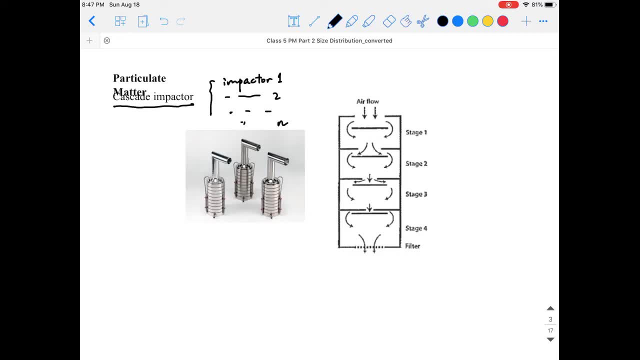 So, as you can see, there are some differences in terms of the geometry and also the configuration for each stage. Let's say the airflow is going through this way And then at the first stage it has a relatively larger opening And also the distance between the stage or the collection stage and the opening is longer. 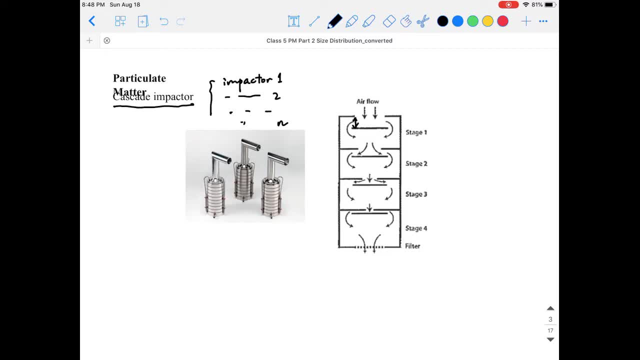 Right. And if we further go downstream, we're seeing that the opening is getting smaller and also the distance is getting smaller. So if we imagine we're putting through a series of particles into the inside airflow and let them pass through different stages, then at the first stage what's being collected? 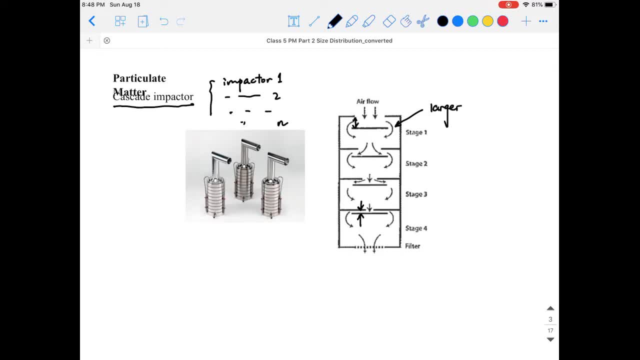 are going to be the larger particles. Particles larger PM. Let's say that right now we start to quantify them as dp, which is the particle size. So dp will be relatively large And as the larger particles are getting collected and the smaller particles are going to get remained, 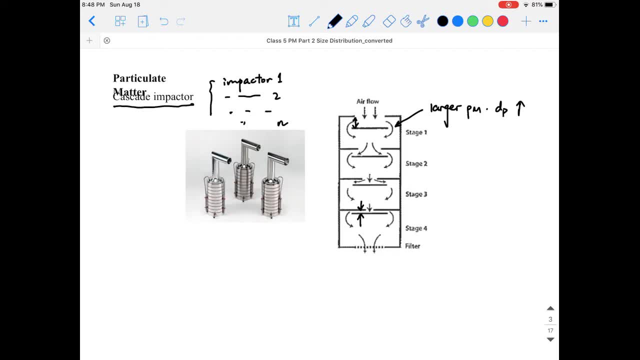 And at the final stage, the particles are becoming really small. So that is the reason why we have to increase the velocity which is a result of the smaller particles, And we have to reduce the velocity of the smaller opening, which will bump up the speed of the particle. 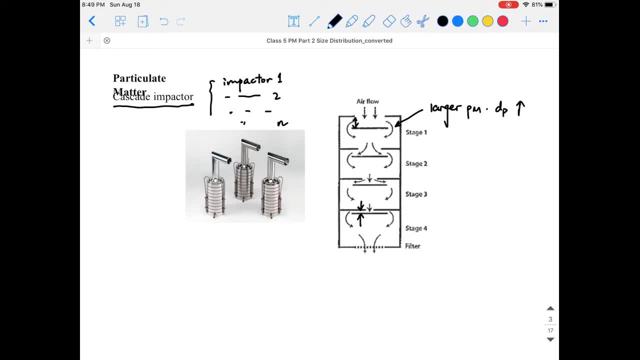 And also by shortening the distance between the opening and the collection stage, we're going to be able to collect the smaller particles. So at the final stages the particle size will be small. We want this configuration for sure, because if we, let's say, switch the stage one and stage four, 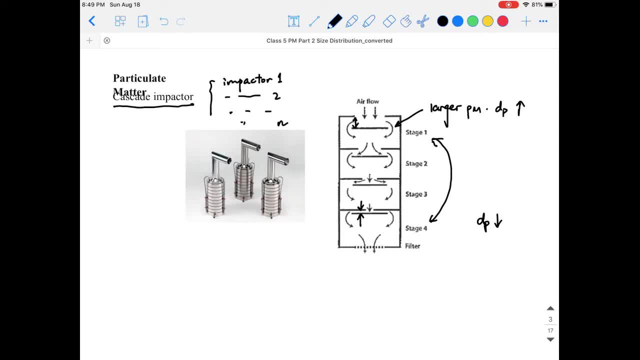 then all the particles with a smaller, with a size larger than this small size are going to get collected, And if the final and then the final stage or the stage one at the end are not going to be able to collect any particles. So that is the reason why we want to arrange so that the particles gradually 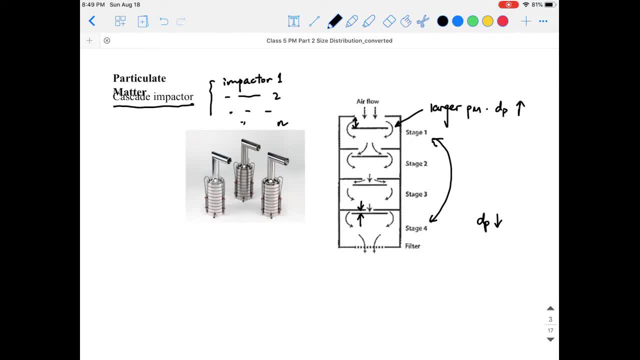 the size corresponding to each stage are gradually decreasing. In this way, we are able to measure particles that are within the size range Or that are between the size cut for the previous stage and the downstream, for the upper stage and the lower stage. 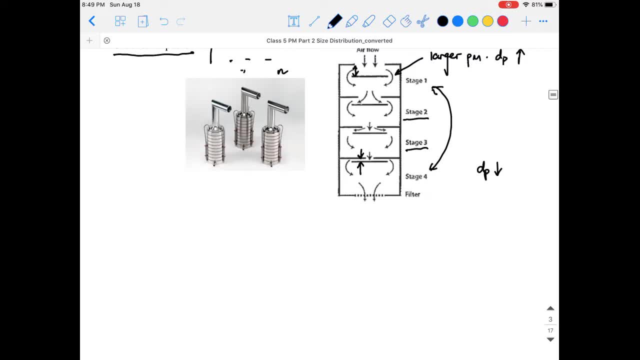 So let's say, for example, that now we have more than four stages. Let's say we have 10 stages. The final, the future, is going to be somewhere at the end. Let's say we have more stages until stage 10.. 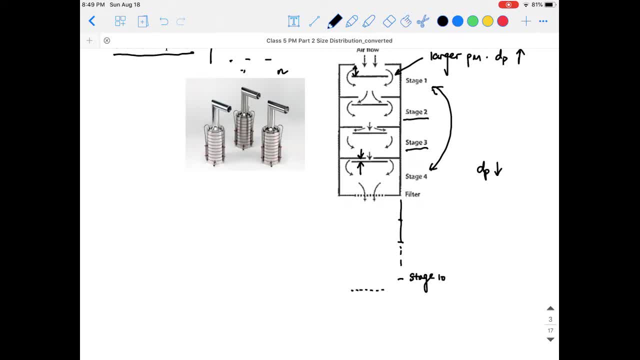 And, finally, it's the future. So what the future does is it's going to collect all the particles that are smaller than the lowest size And in this way we're able to say that part, all the particles larger than zero nanometer, until the size cut of the previous stage, are going to be measured with a future. 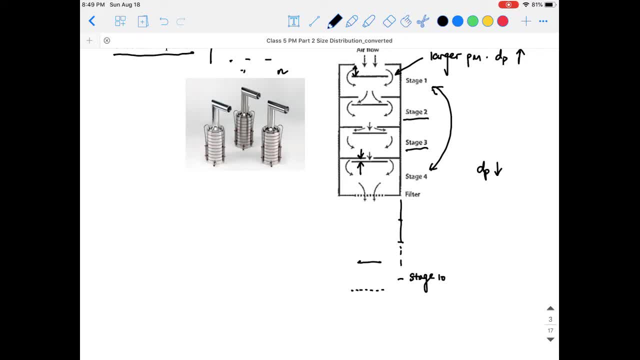 And we can weigh the future to measure the mass of the particles. So let's say further: assume that the particles or the size cut for each stage are going to have a size of 2 micrometer, say 4 micrometer, until there are 10 stages. 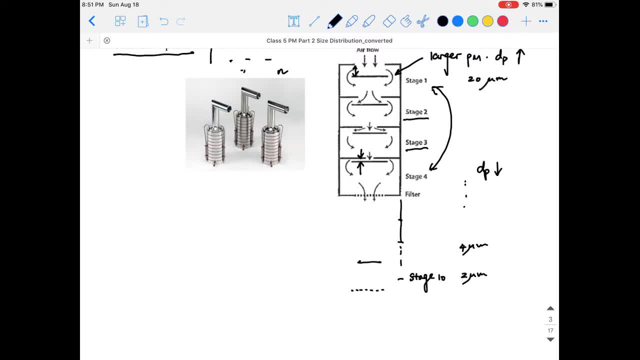 So it's going to be until 20 micrometer. Okay, So by measuring the mass on the second stage, we're going to obtain the mass of the particles that are larger than the delta mass, that are larger than 18 micrometer but smaller than 20 micrometer. 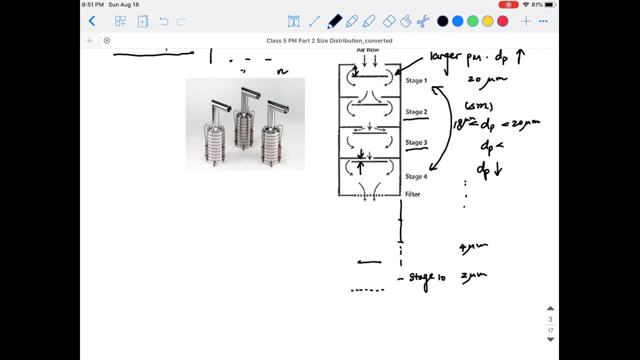 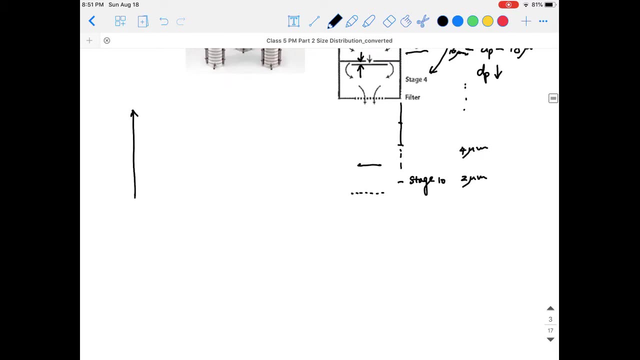 And similarly for the stage 3, the particle size is going to be smaller than 18 micrometer, but larger than 16 micrometer, Right? So in this way we're able to basically create a size distribution. Let's say the x-axis is the particle size. 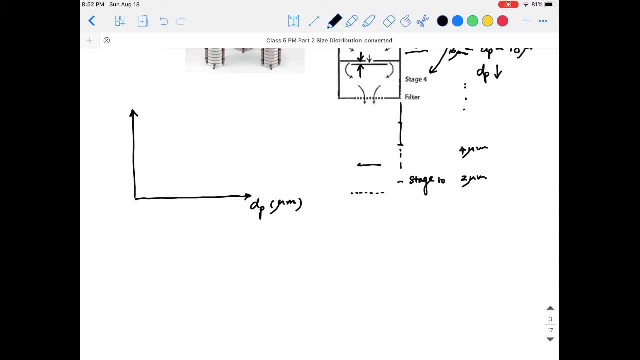 Let's say it's a micrometer, And the y-axis what we're going to use is the delta m divided by delta dp. So basically, the area that we obtain from each of these columns here are going to be the mass or the delta mass. 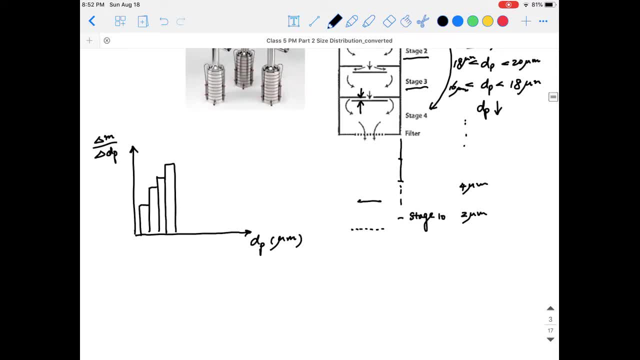 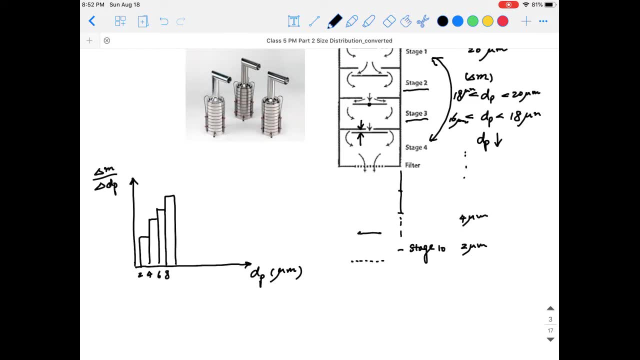 are going to be the mass of the particle that's collected on certain stage here. Okay, So let's say it starts from 2,, 4, 6,, 8,, 10, and then 12 until the end. Okay, 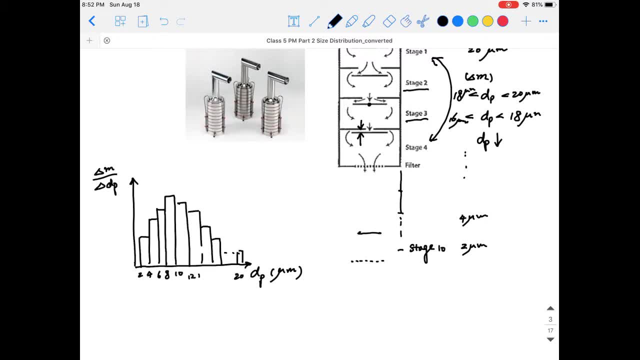 Let's say this is 20,, 12,, 14,, 16,, 18.. So I guess that I don't need to go that far, So this is going to be 20.. Okay, So this basically gives us a size distribution. 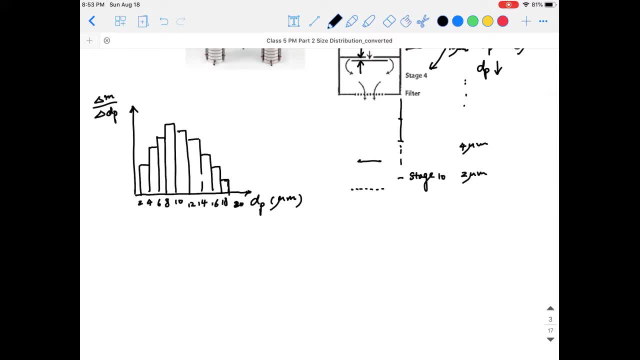 and this is definitely a rough size distribution. We also call this as a size distribution. that's in the discrete form, Because this size distribution cannot represent the actual size distribution The way I mean it is, because let's say, for example, for particles that has a size of 10.5 micrometer. 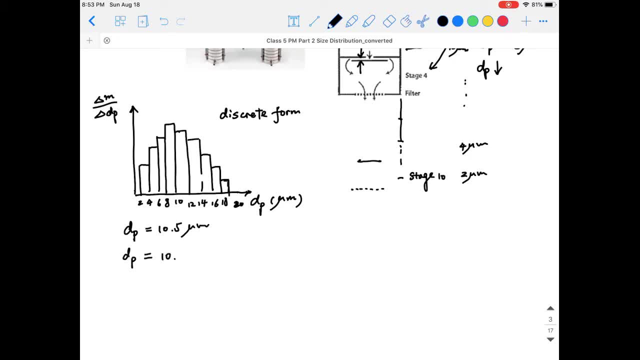 and for particles with a size of 10.8 micrometer. if this is the real size distribution of the particles, then what it means is that the concentration of the particles at this size and at this size are going to be the same Right. 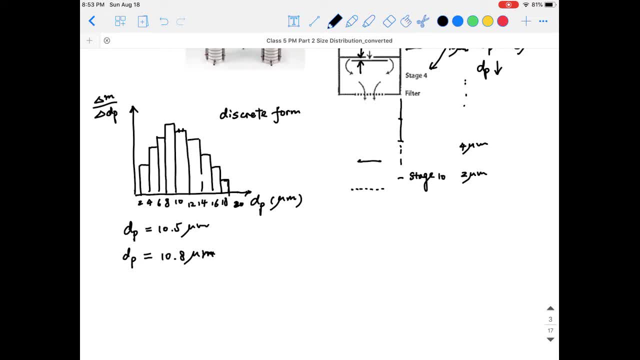 But this is not the case, Because in real situation, it's going to be a continuous form And in very rare situation, the particle concentration will be the same. So it's going to be a continuous form And, due to the resolution of the cascade impactor. 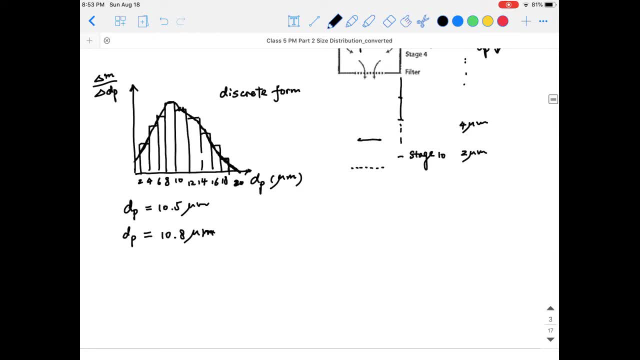 we're not going to be able to measure particles with this continuous form, But still people would prefer to use some mathematical way or to use some equations to describe the particle size distribution. Okay, And this further involves the quantification of the size distribution. 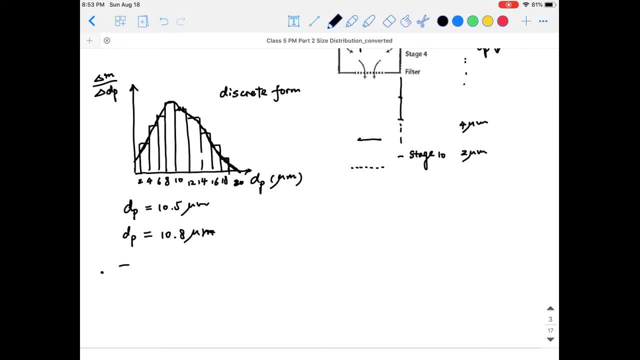 or in constraining the size distribution with equation forms, Let's say equations for size distributions. Okay, So if we directly look at this form, let's maybe try to draw it here. Okay, They're going to be, they're going to have. 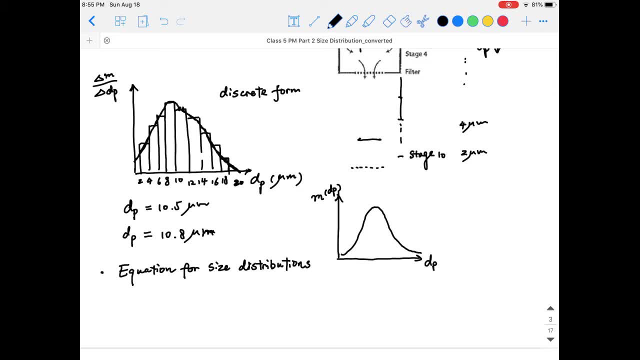 a shape like this. Okay, And interestingly, many ambient size distributions will have these type of shapes And in mathematics we know that there's a term or there's a prescribed distribution called Gaussian distribution to describe this type of distribution. Right. 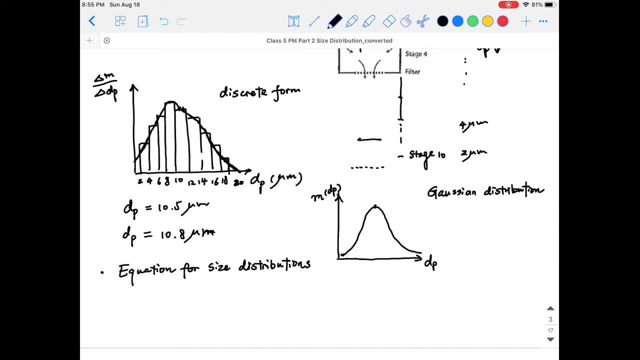 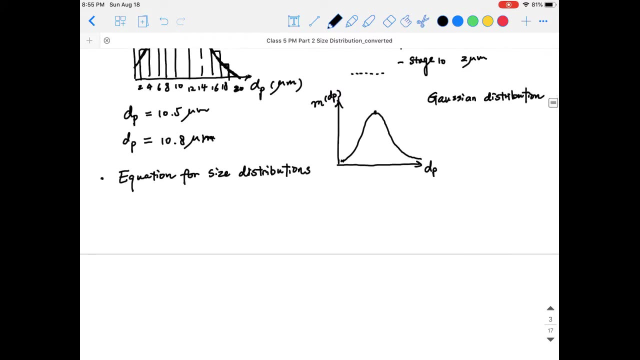 So normally there will be a peak that corresponds to the maximum mass concentration, And normally the slope or the curve before and after the peak are going to be symmetric, And similarly we can use these type of Gaussian distribution to describe the particle size distribution. 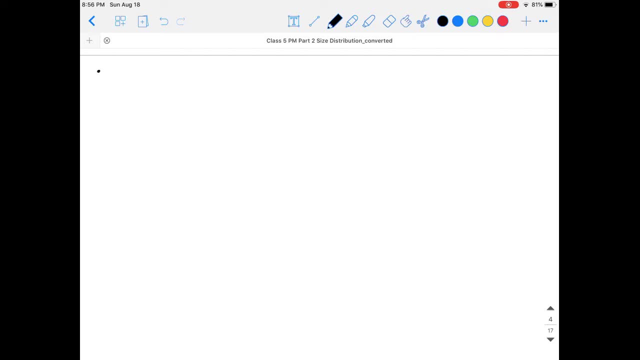 So then it's going to have a form of- let's first write it down again- So it's going to have a form of MDP equal to M total square root of 2 pi sigma exponential minus dp, minus dp average, or the mean of dp. 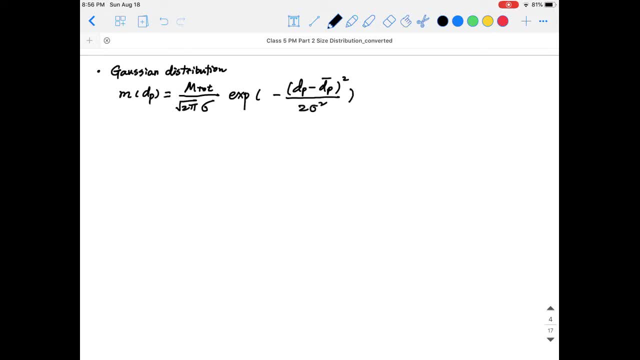 square divided by 2 sigma square. Okay, So in this equation the M total is the total mass concentration. Okay, The sigma here is the standard deviation of the size And the dp min is actually, as we show, is the 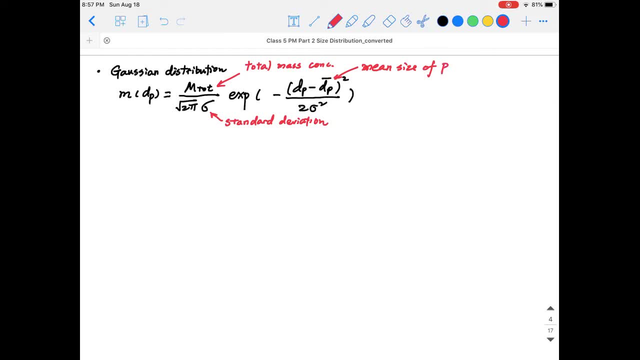 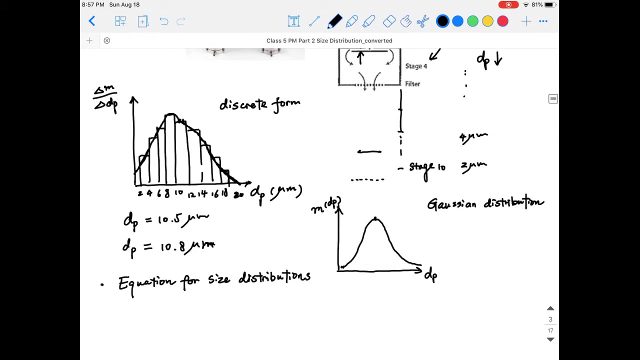 mean size of the PM. Okay, So the reason why we have this type of form is because the integral of the Gaussian distribution is the M total. So, similarly, this actually corresponds to the same situation for the size distribution we show here. So, basically, 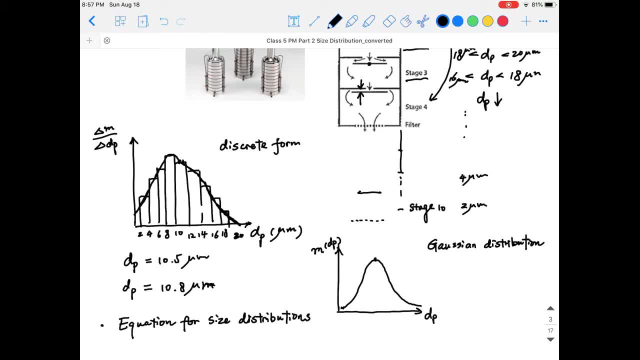 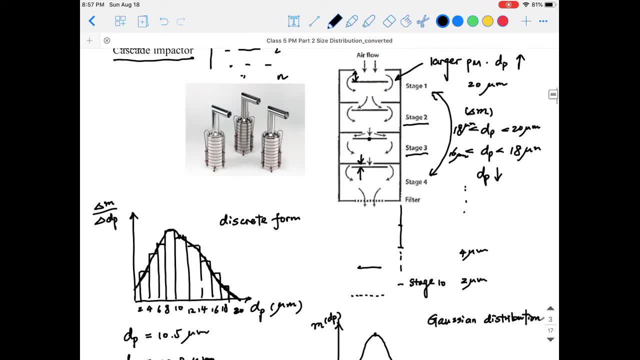 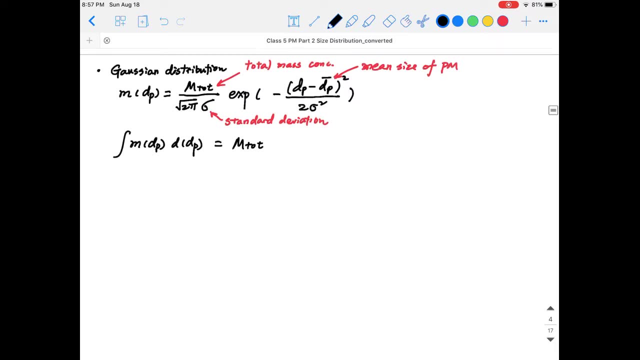 the average, or the the area below each bar, or by summarizing the area of all bars. it's going to be the total mass concentration that's collected on all the stages and the filter. Okay, So for a continuous size distribution, we want it to be defined in the same way. 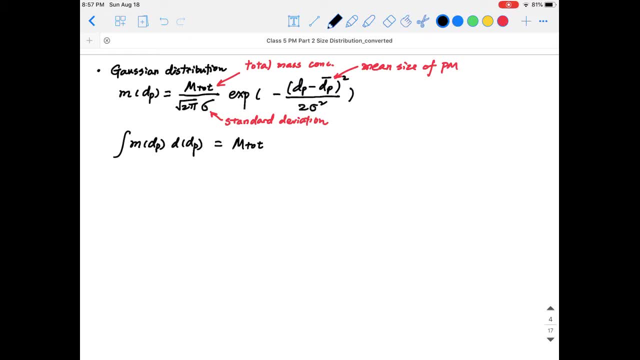 But actually there are some problems if we use such a Gaussian distribution to describe the particles. And there are actually two problems. The first one is if we check the definition or the range of the particle size, we can see that the particle size can actually be smaller than zero. 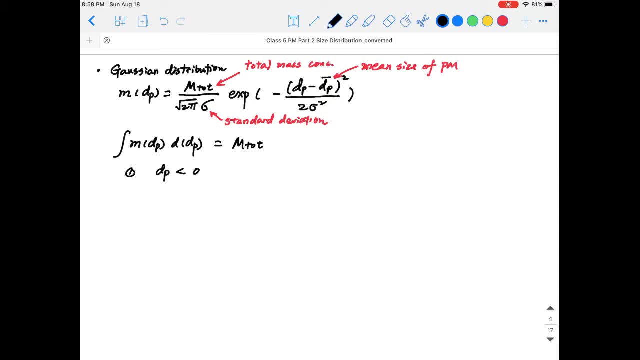 Right. What it means is that if the particle has a size of minus 10 micrometer and if we plug it in, it's still going to give us some distribution, Right? So the Mdp is still larger than zero. But this doesn't make sense. 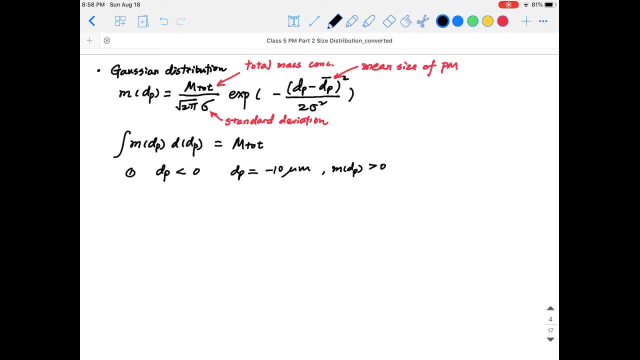 because we know that the particles will not have a negative size. And you may say that why don't we just put a constraint on the particle size? Let's say we still have this type of form, but we have to define that or have to say that the dp is larger than zero. 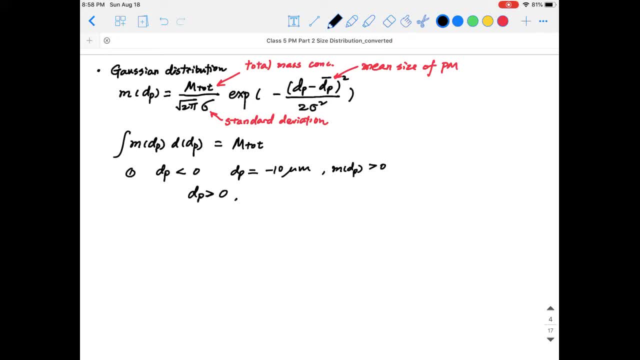 But if we set such a constraint in terms of the particle size, then the integral of the mass concentration, or the size distribution, will be smaller than M total Right. And this is because, again, when this happens, the Mdp is larger than zero. 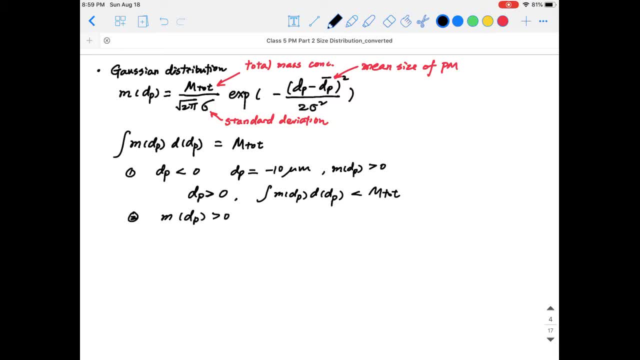 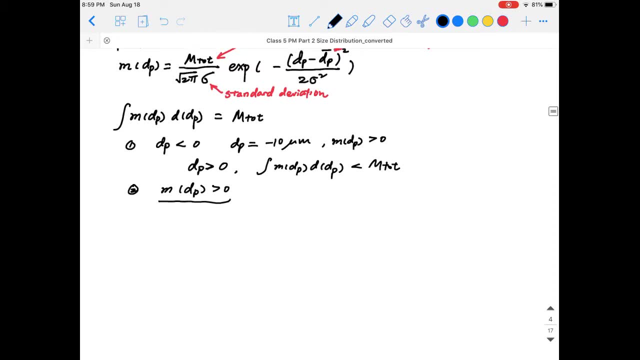 So basically the two problems are: first, the particle size can be smaller than zero, And also, when particle size is smaller than zero, the mass concentration can be larger than zero, Or we can combine that. Basically, it didn't put a clear constraint. 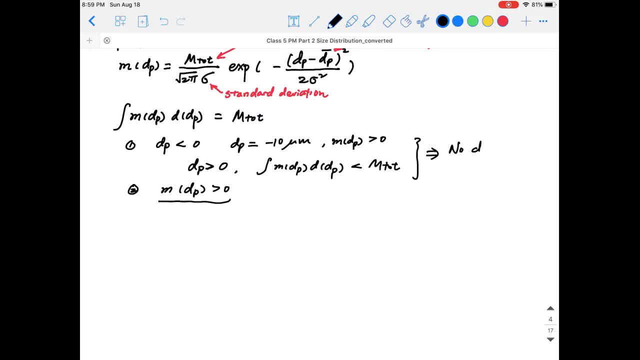 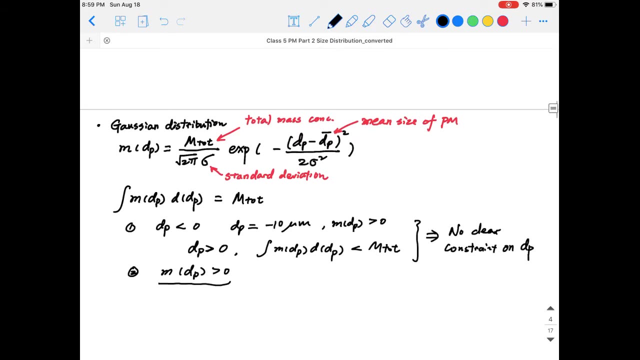 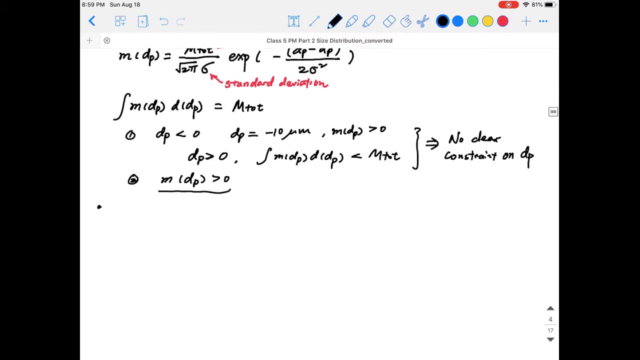 on the particle size. Okay, So this is the reason why people created another type of size distribution or another type of distribution to describe the particle size distribution, And this is the log-normal distribution. Okay, So, in a log-normal distribution, I'm just going to write down: 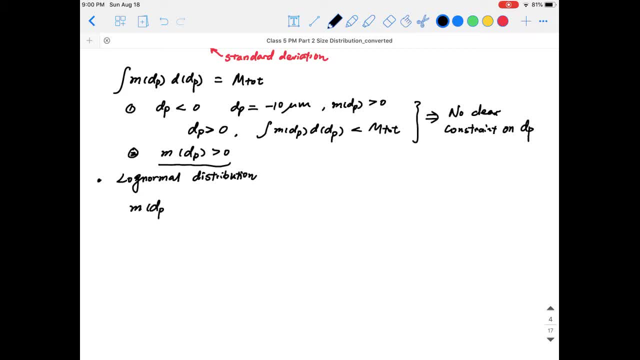 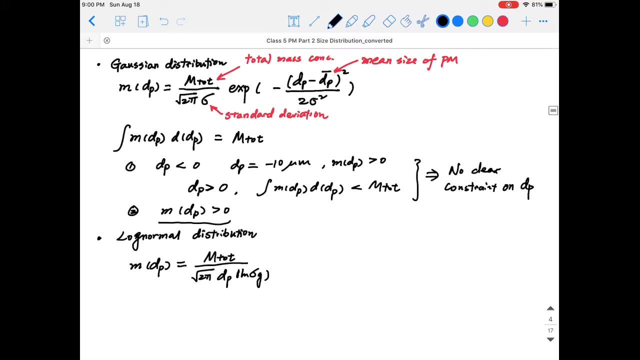 the mathematical expression here. So it's going to be still M total at the denominator, And now it's divided by 2 pi, dp log, sigma g. Okay, Please notice the difference between these two equations. So you see that now we have an extra dp term here. 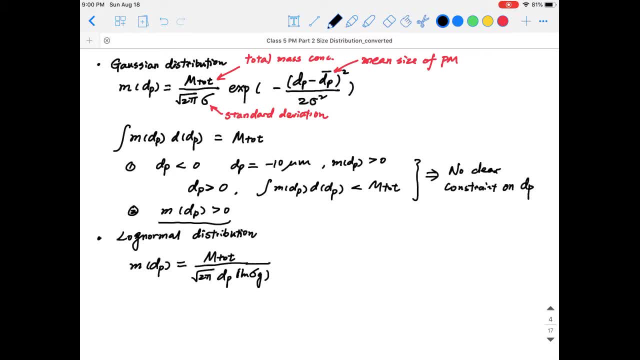 And also the sigma is changed to the log of sigma g And in the exponential term we have log dp minus log dp g, still squared, divided by 2 log squared sigma g. Okay, So now we have to define a few more terms. 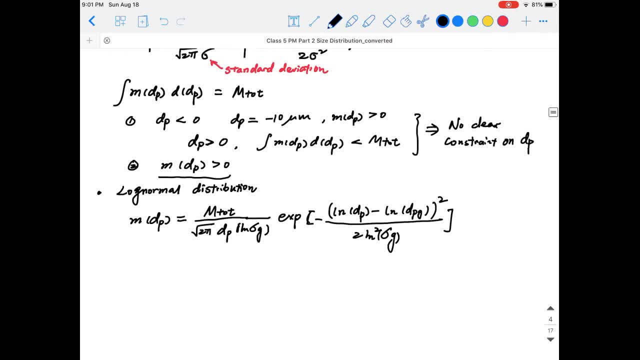 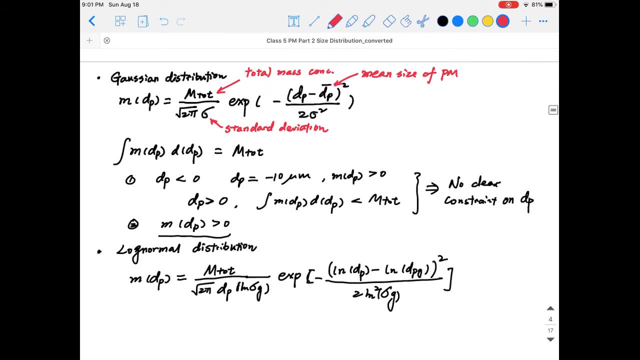 Okay, So the M total is still the same. That is the total mass concentration. So we know this one. And then dp is the particle size which is basically showing the function as a function of dp, And the sigma g here is a new term. 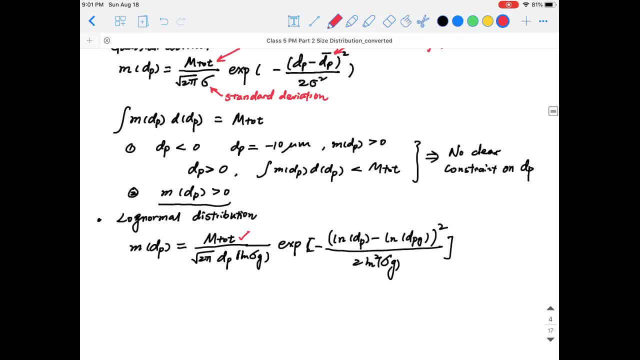 And this is called the geometric standard dp and the sigma g here is a new term And this is called the geometric standard dp And this is called the geometric standard dp And this is called the geometric standard deviation of the particle size And the dp g here. 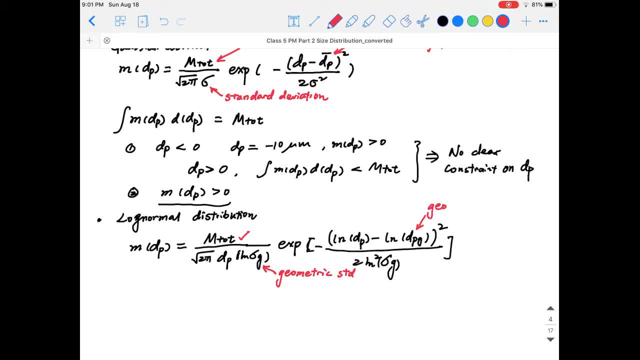 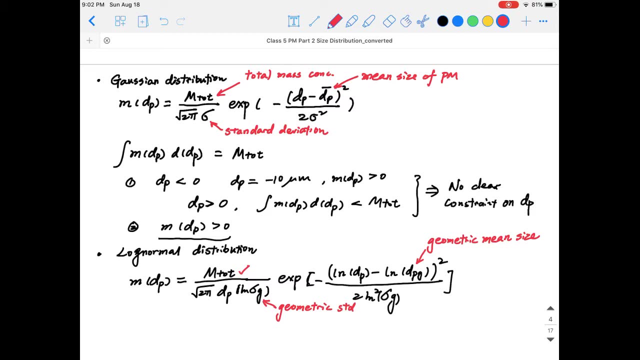 is the geometric mean size. So the difference between the mean size and the geometric mean size, calculation of these two terms. the mean size is directly the. it's also the by directly averaging all the different sizes. but the geometric mean size is based on the product of all the sizes and then take the corresponding root of. 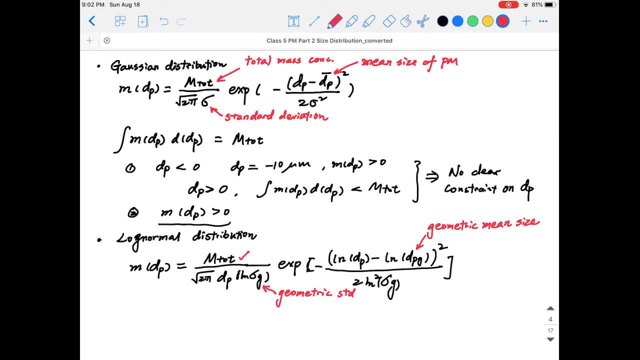 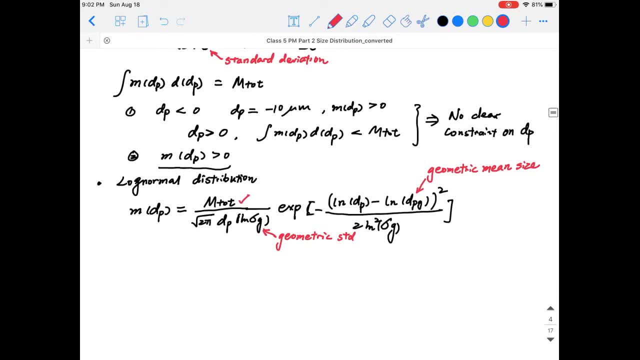 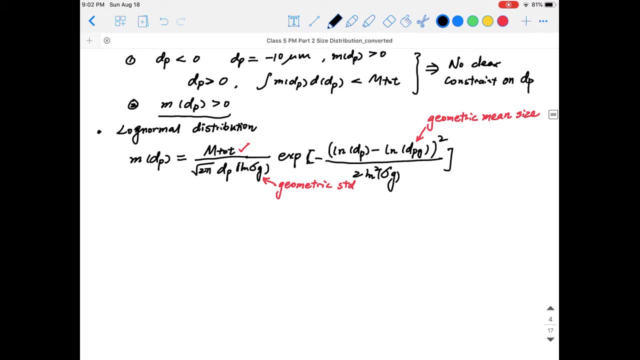 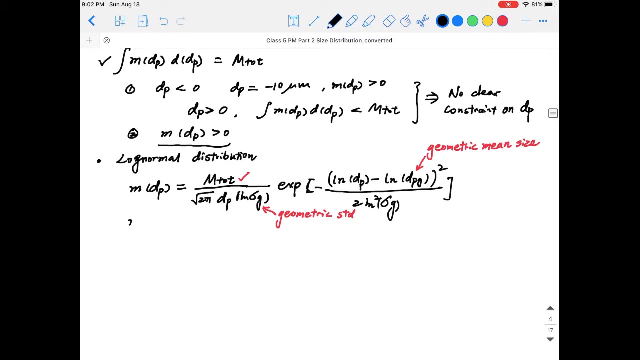 all the side of the product so that we can get this geometric mean. so one is directly algebraic and the other one is by multiplication. okay so, but interestingly, for the log normal distribution that also satisfies this condition. okay, we can easily prove that, because now if we use MDP, DDP, we're 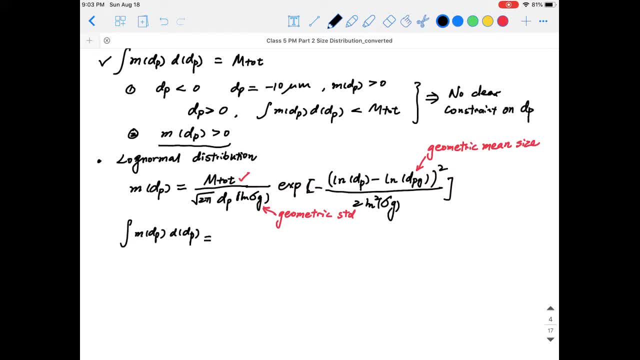 going to still carry all these terms, but one thing that we need to do is we need to do, is we need to do, is we need to do. a thing we need to notice is that- let me just write it out here: square root of 2 pi log Sigma G: exponential okay. log DP. minus log DPG: 2 square Sigma G: okay. 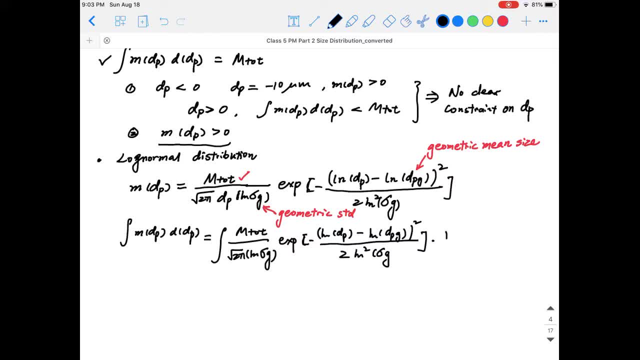 so now we can make some substitutions. I'm actually missing one term here, that is 1 over DP, DDP. okay, now we can make few substitution, so what we can do is: let's set, let's set and just finish this bracket here. let's set log Sigma G as: 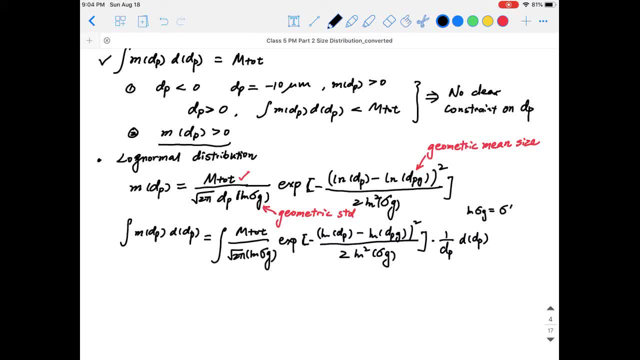 Sigma prime. okay, and log DPG as DP G prime. okay. so we can substitute these two terms in, because they are just constants. they are not relevant to the particle size here, right? so let's see what happens. it's going to be M total square root of 2 pi Sigma Prime. 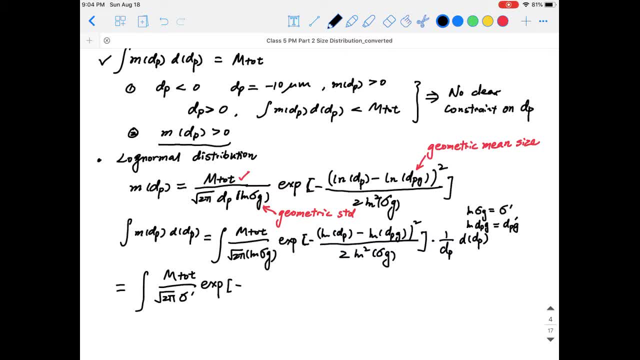 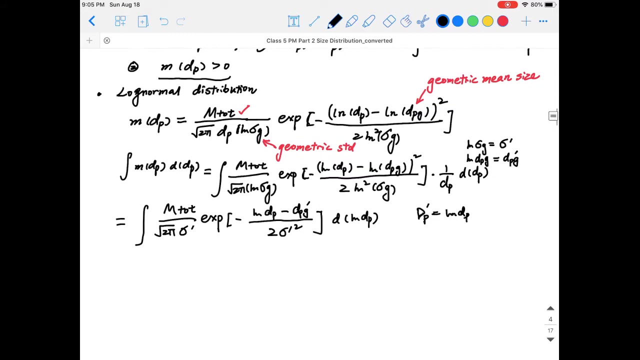 exponential minus log dp, minus dp g prime: okay. 2 sigma prime square, Actually 1 over dp multiplied by ddp is d log dp. okay. So we can make another substitution. Let's use dp or the capitalized dp equal to log dp, or capitalized dp prime, okay. 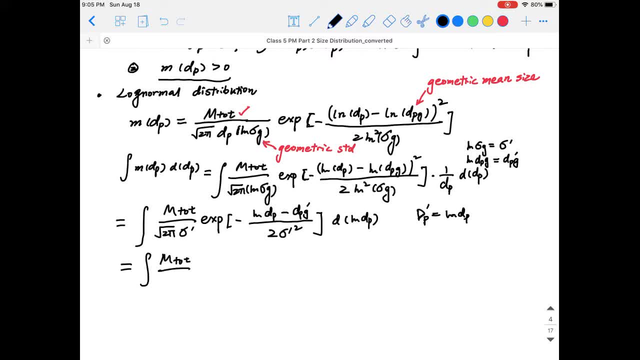 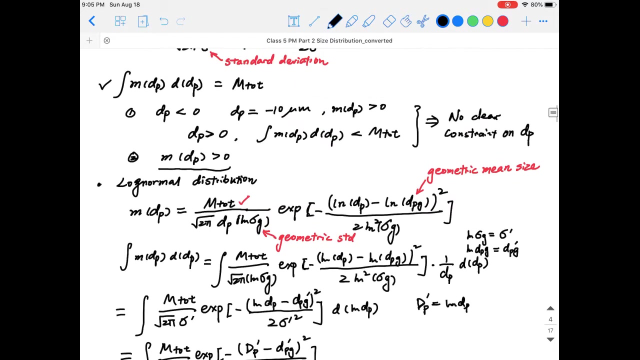 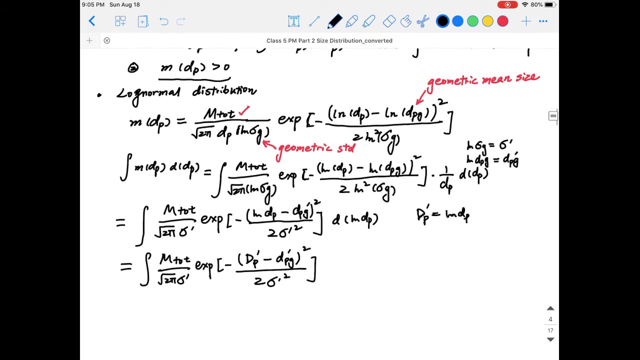 So what we're going to have is m total square root, 2 pi sigma prime exponential minus dp prime. okay, I forgot a square term here. okay, dp prime minus dp g prime square divided by 2 sigma prime square. So let's compare these two terms, or the Gaussian distribution, and this substituted: 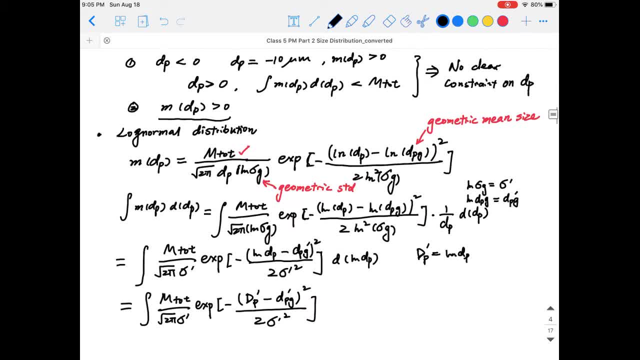 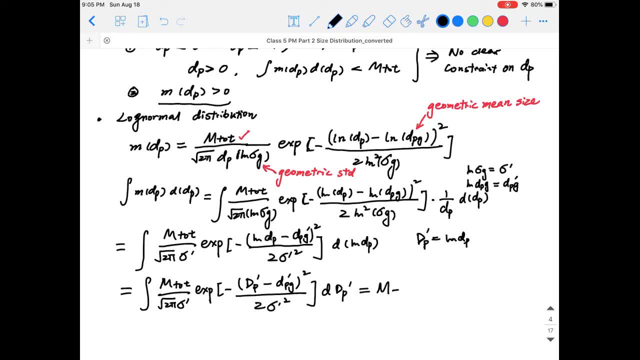 log norm distribution. You can see that they're the same right, And what this means is that this will still be equal to m total. Okay, So you can see that they're the same right. So you can see that for the log norm distribution, if we integrate the size distribution, it's. 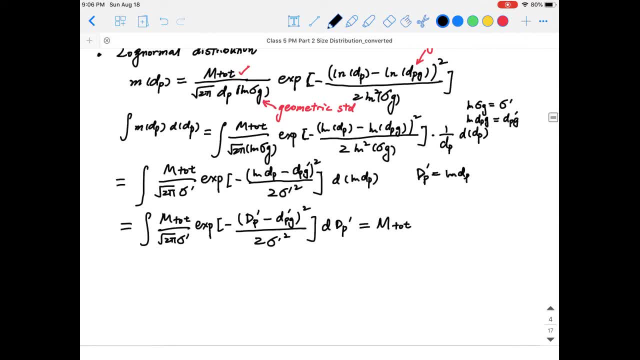 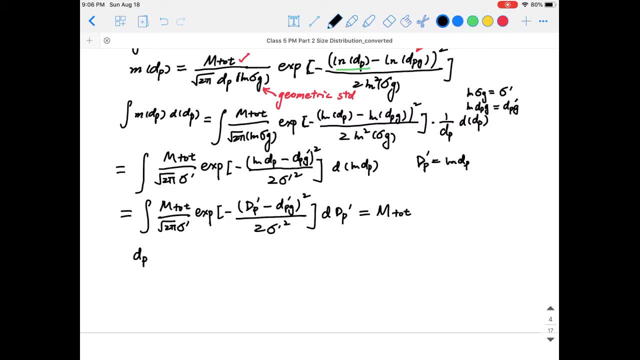 still going to give us the same total mass. And the difference now is that the dp in this term here, the dp in this term here, has to be larger than zero, because we're using log dp as a term within this log norm distribution right. 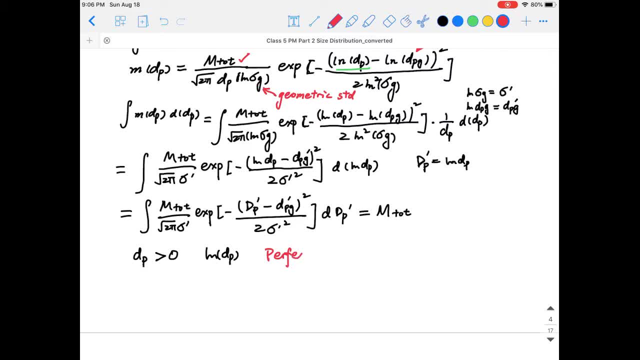 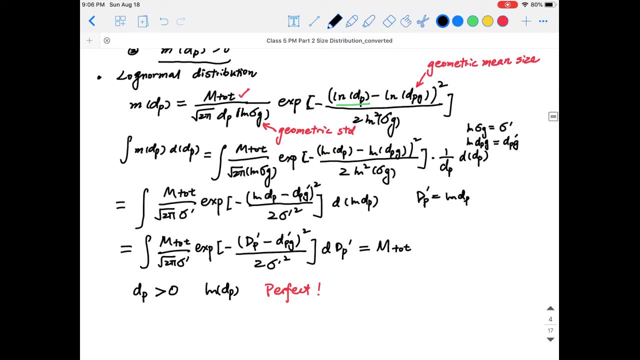 So now let's say it's perfect And actually if we use any instrument and just measure the size distribution outside for the ambient and for a lot of the situations, they are indeed going to follow the log normal distribution, okay, And the major difference for log normal distribution and the or the or the Gaussian distribution. 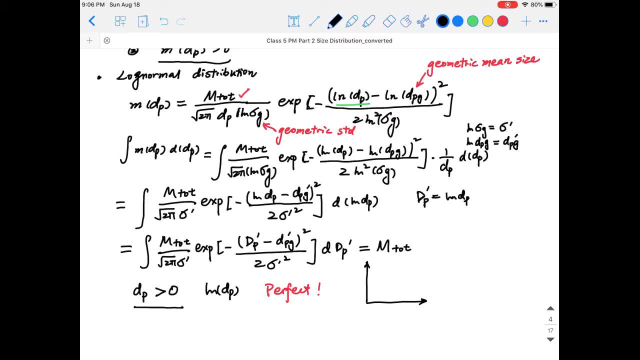 apart from the definition of the dp here or the constraint of the dp here is actually, if you draw these two terms, you can see that the log normal distribution is going to be the same. So let's say we have these size distributions out. 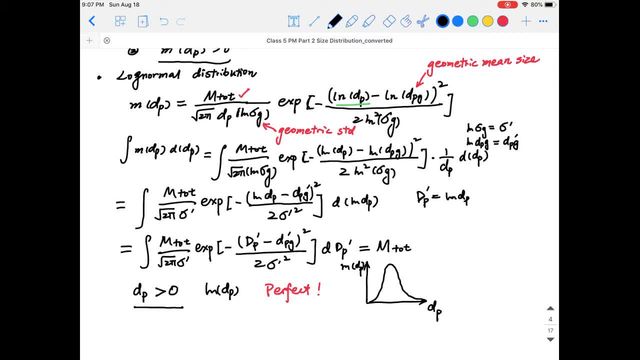 For Gaussian distribution. if we have these symmetric, symmetric size distribution, then the dp has to be in the linear term. What it means is that a 10 micrometer is at the peak, and this then this is 9,. this is 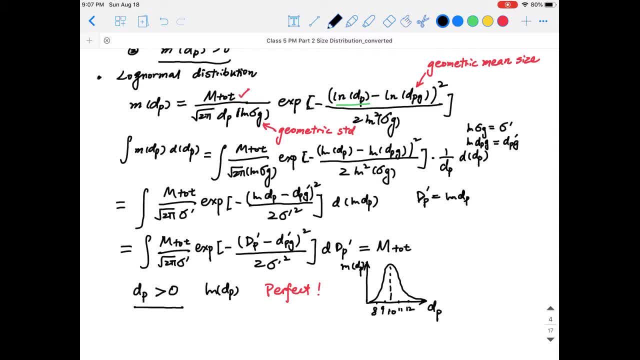 11,, this is 8,, this is 12.. But for a log, normal distribution, what's going to happen is that it's still symmetric, But this only happens when the dp is shown in the log, in the log scale. So, basically, if this is still 10, and here it's 1,, and here is 100,, okay, 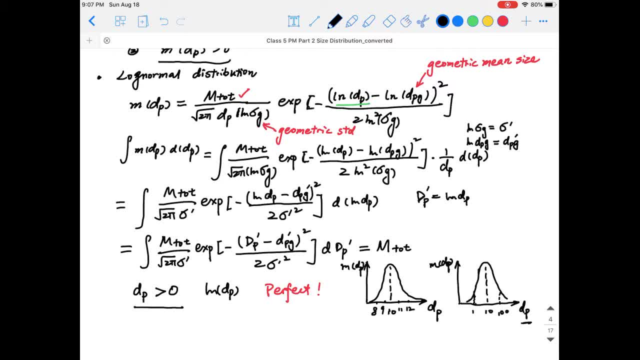 Because we're taking the log of the particle, So basically we have to convert it. If we're taking, for example, if we're taking log 10 of dp, this means that this is 1,, this is 0, and this is 2.. 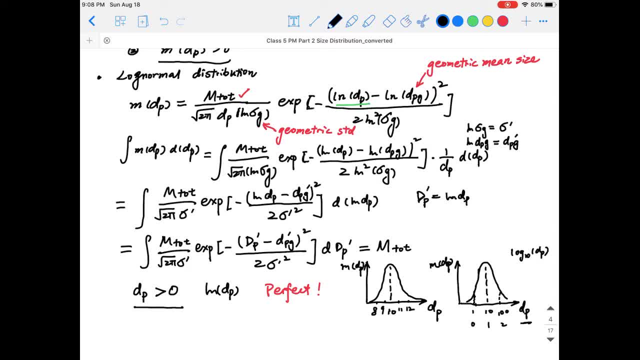 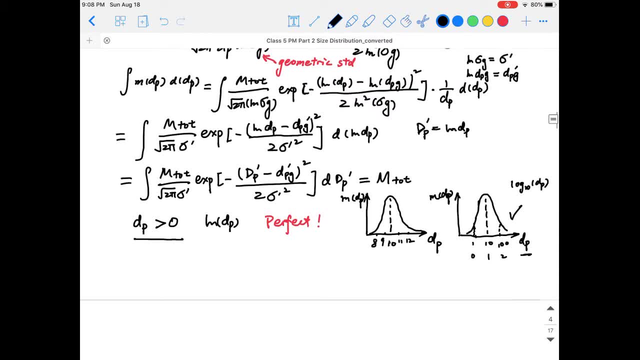 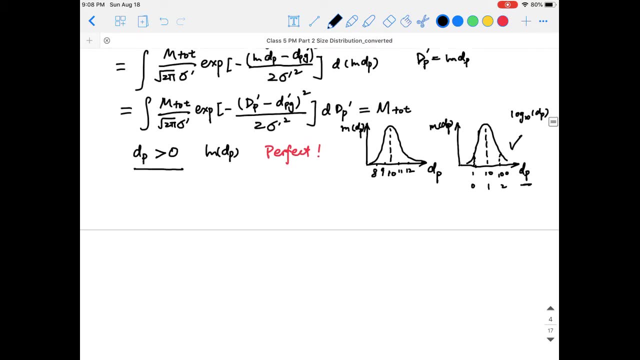 So these are the two major difference between the log normal distribution and the Gaussian distribution, And we prefer the log normal distribution to describe the size of the particles. okay, And now let's look at the some properties of the of the log normal distribution, because 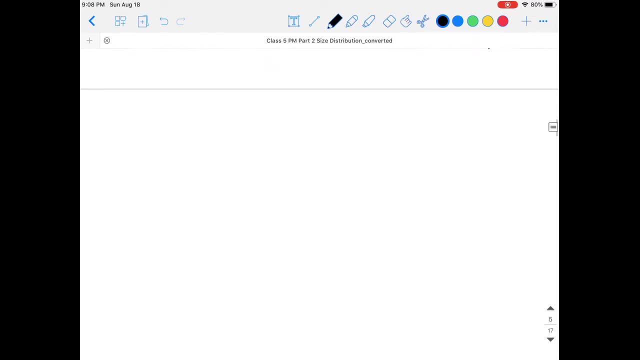 it's very important And we can use it to actually solve a log. So let's look at a lot of the problems, a lot of problems. So now we can look at the properties of log: normal size distribution. okay, So the first one is the cumulative mass fraction. 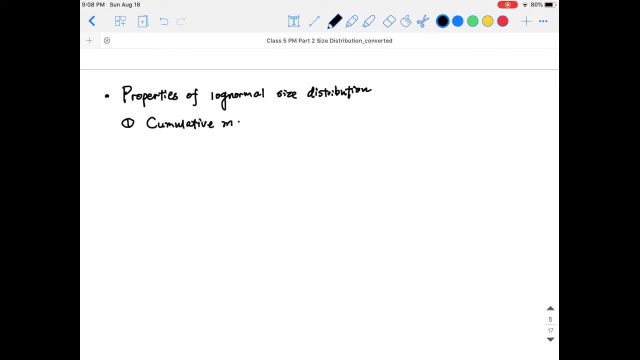 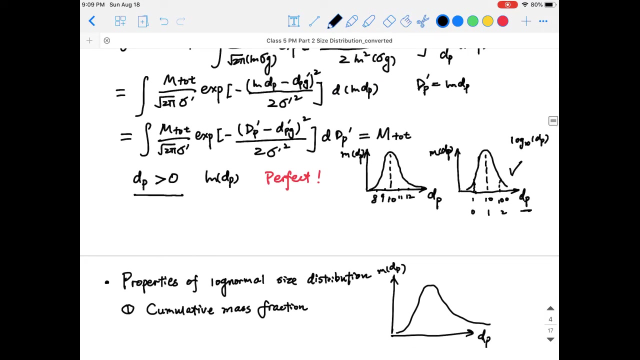 So let's say, we're still drawing the size distribution out and this is the log: normal size distribution. It has a form like this. So one thing that I forgot to mention is that. so here, basically, it's showing the 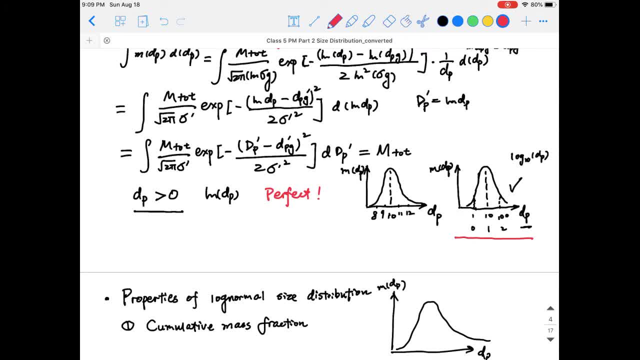 size distribution In the log scale. So what happens if we convert it to linear scale? So what's going to happen is it's quite clear, right? So originally the gap between 1 and 10, and 10 and 100 is the same. 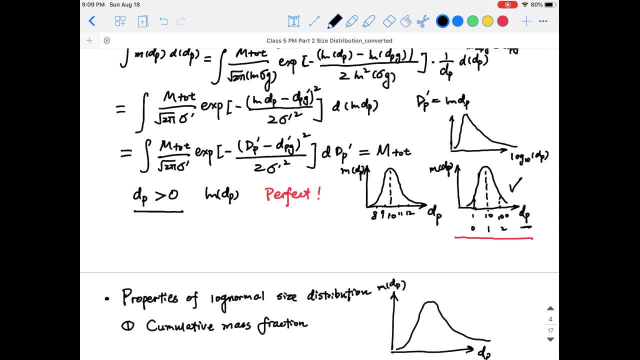 But if we change it to linear scale, it's going to be something like this: right, It's going to have a long tail And actually this is a more appropriate, appropriate way for describing the particles, because there's always going to be a gap. 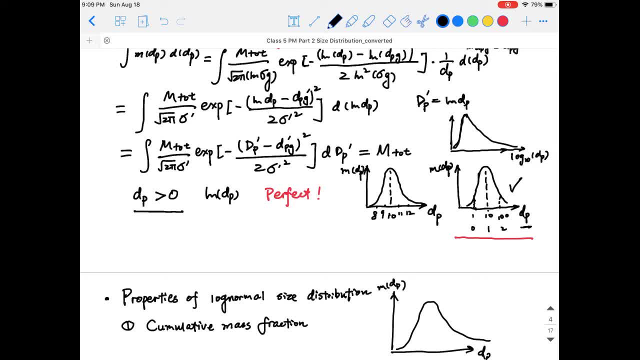 There's always going to be some particles at larger sizes. For example, if we throw a bunch of some sand into the air, there's always going to be some larger rocks existing in this bunch of sand. okay, So the concentration at infinitely large is not. it's non-zero under most scenarios. 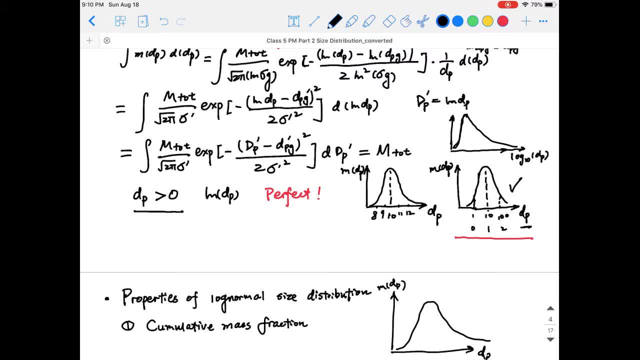 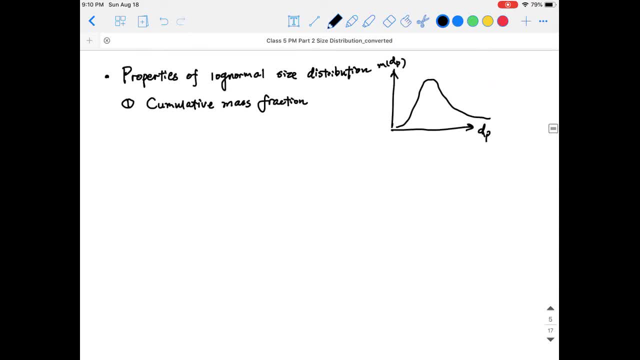 So that's why the log normal size distribution is more is a more commonly accepted way to describe the size of the particles. Okay, So now let's draw it again and let's say that we set the dp in the log scale. so it's. 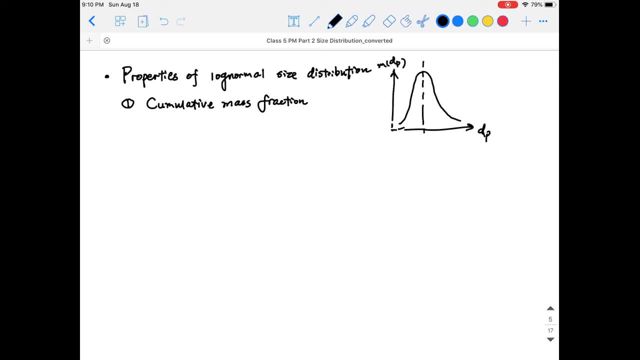 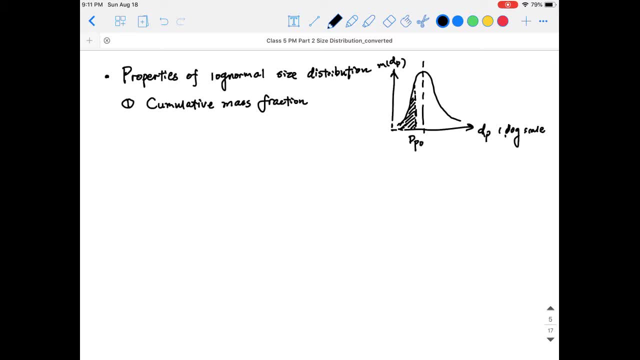 size. Let's say dp is 0, below certain size over the entire mass concentration. So in a more mathematical way we can define that as Fm. So Fm is the cumulative mass fraction And that's going to be a function of, let's say, the capitalized dp, because we're still using the smaller dp, lowercase dp, to describe the size distribution. 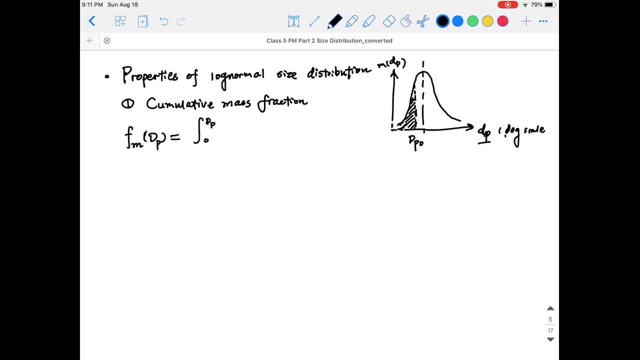 And that is going to be integration of zero to capital dp, m dp, d dp divided by m total. Okay, So this is the definition of the cumulative mass fraction, And actually we can plug in the form of the log-normal distribution and then do the integration. 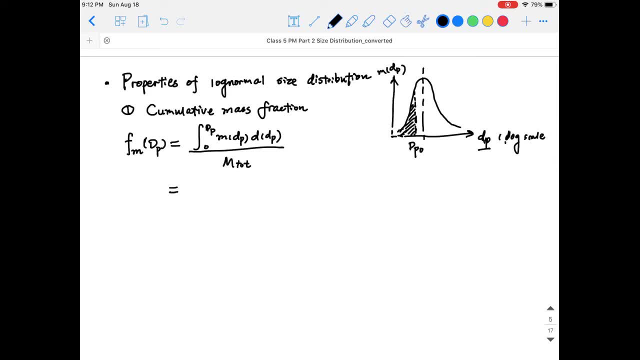 And luckily, some others have already done the integration in the analytical way for us And if you're interested, you can feel free to have a check on how we can do this integration. But the result for this integration is actually 1 over 2, is actually in a quite elegant and simple way. 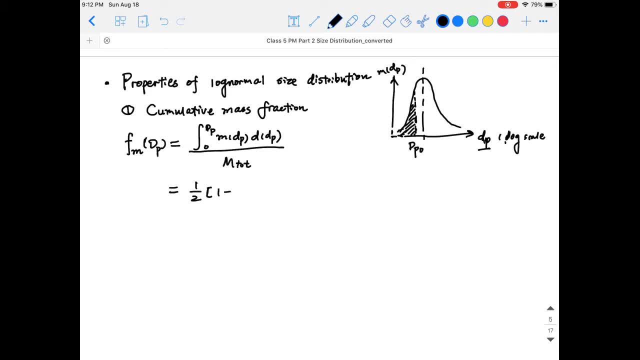 1 over 2 multiplied by 1 plus e or f, and this is called error function. And inside the error function is log dp divided by dpg over square root of log sigma g. Okay, And again, we still remember the definition for these two terms, right. 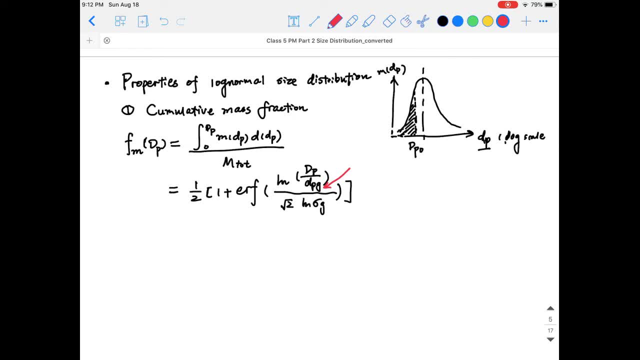 So the dp is actually arbitrary size that we are interested in. It can be 1 micrometer, it can be 100 micrometer and so on and so forth. But the dpg is associated with the log-normal size distribution And this is the geometric mean of the particles. 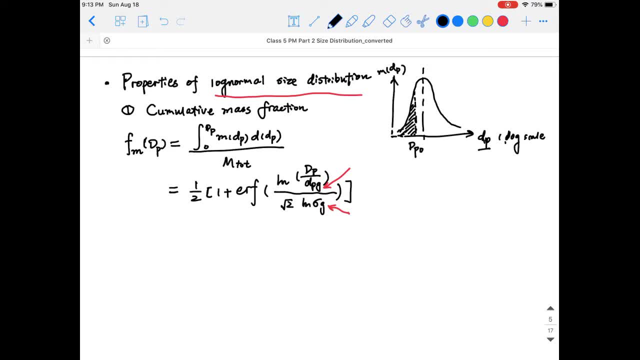 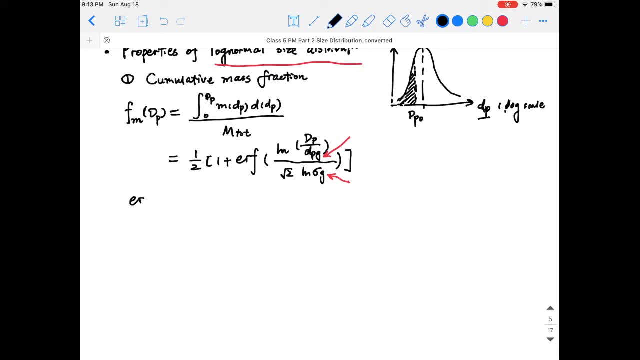 And the sigma g is the geometric standard deviation of the log-normal size distribution. And here we saw this error function. So actually the error function has its analytical expression of 2 over pi multiplied by integration from 0 to z exponential minus x squared dx. 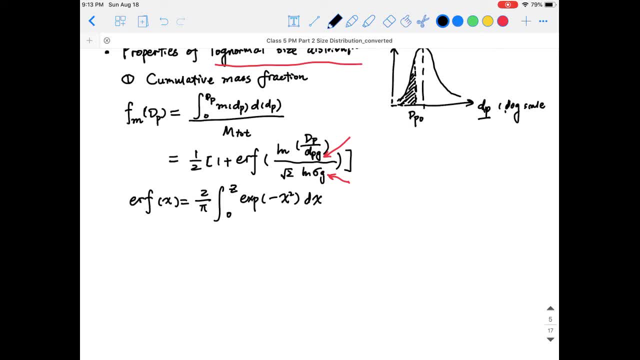 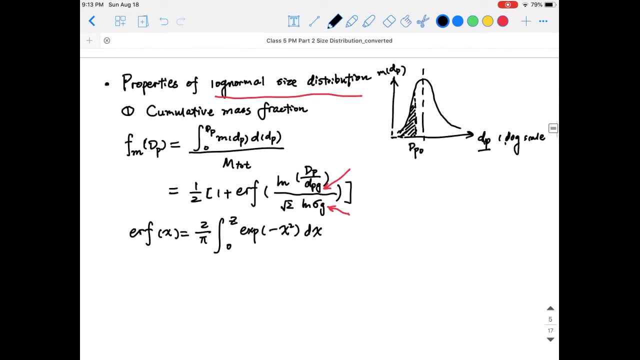 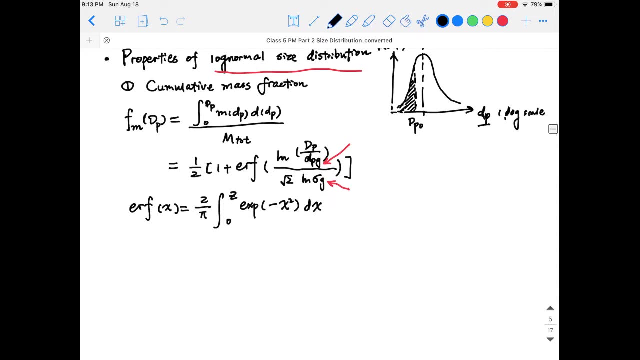 Okay, So this seems to be very complex And I know that in this class we have gone through quite many equations here, But you can see that you can later find out what simple results we can obtain by going through these derivations. Okay, 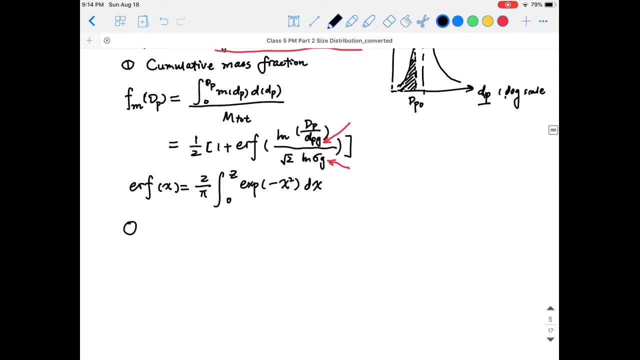 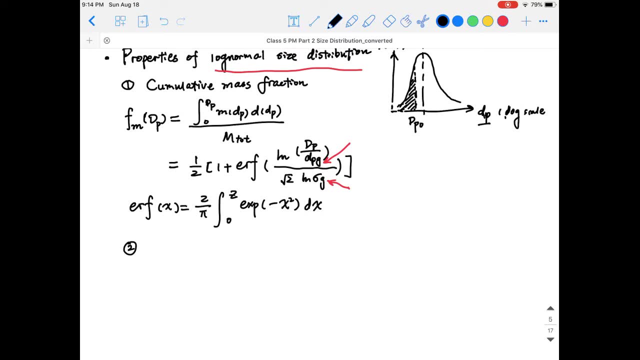 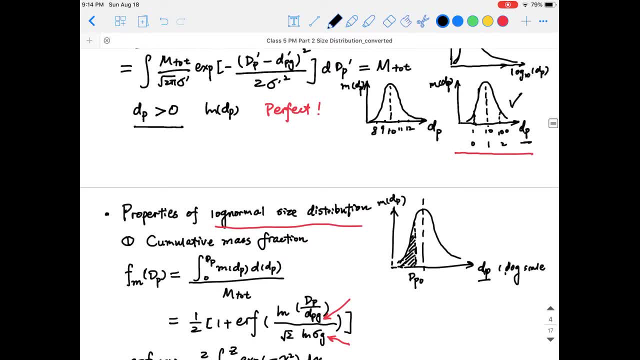 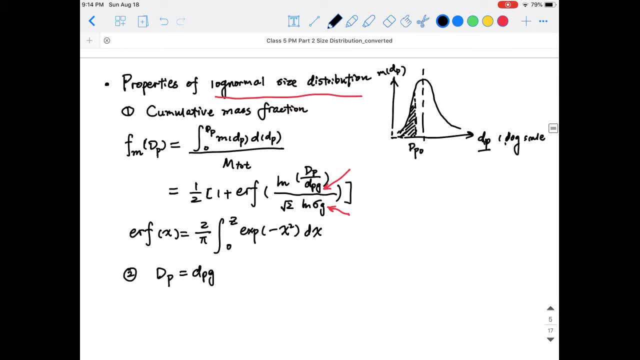 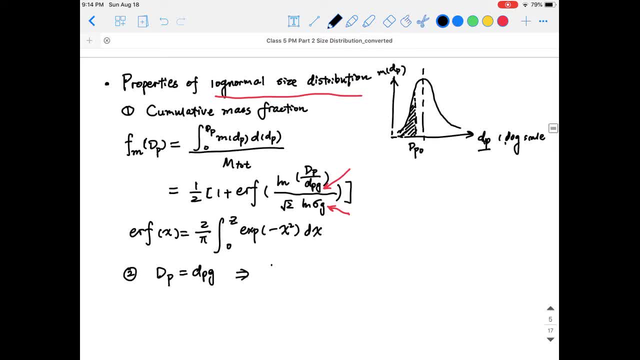 But since we already have this term, this form here, so we can directly plug in, So it's going to be dpg And this is going to be dpg, So it's going to be dpg, plug in. That's going to log. 1 is equal to 0.. 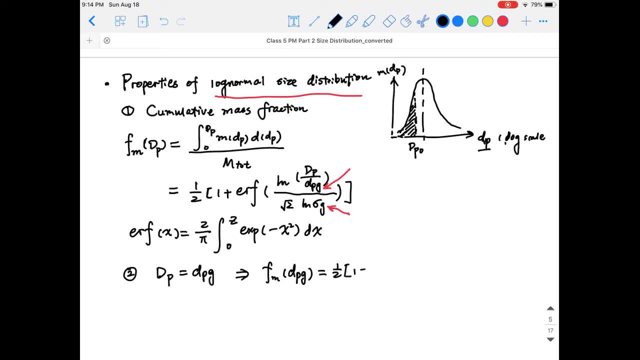 Right, So it's going to be 1 over 2, 1 plus error function of 0.. Now you may wonder: what is error function of 0?? So the error function of 0, basically, let's see I made a mistake here. 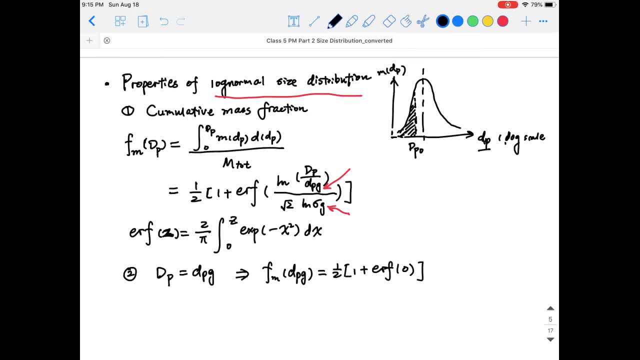 So this should be error. function of z is equal to. So basically, if I plug in z equal to 0,, then the integral here it will be 0.. Right, So the result will be 1 over 2, which is 50%. 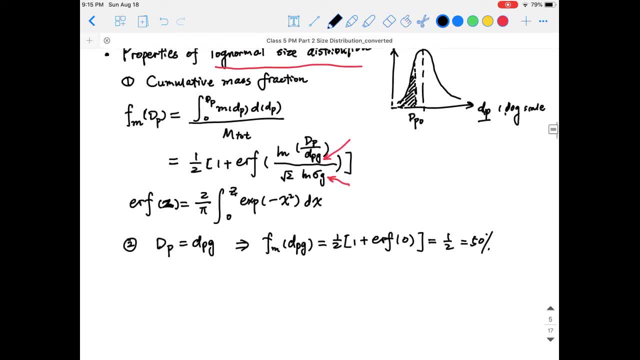 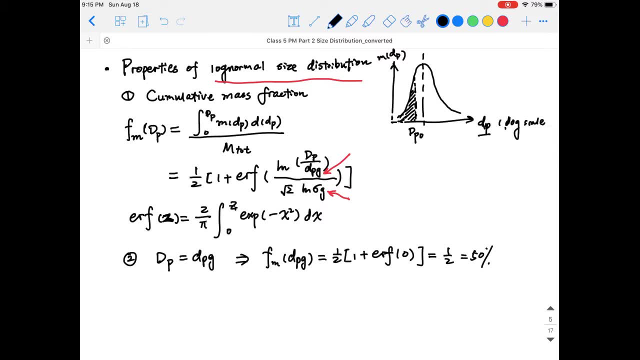 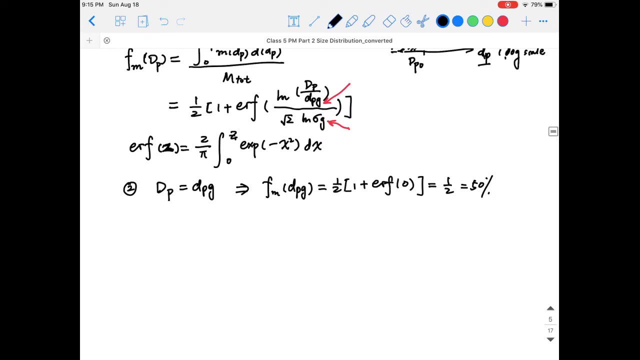 So what this means is that when the particle size is equal to the geometric mean size of the log normal size distribution, then the cumulative mass fraction will be exactly 50%. Okay, Okay, Okay, Okay. And we can also try some other interesting things. 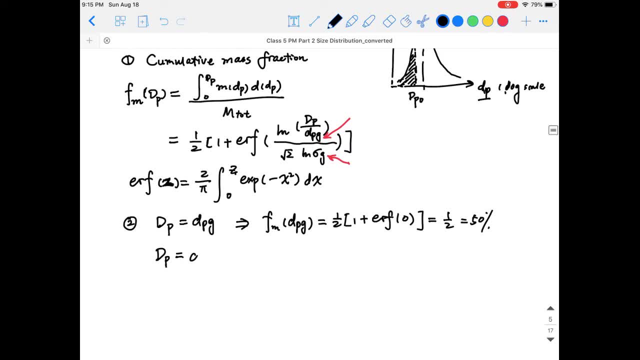 So if we plug in the dpg- dp equal to dpg multiplied by sigma g- and then what we can get is going to be equal to. we just plug in everything here And then inside this term here, we're going to cancel out the dpg. 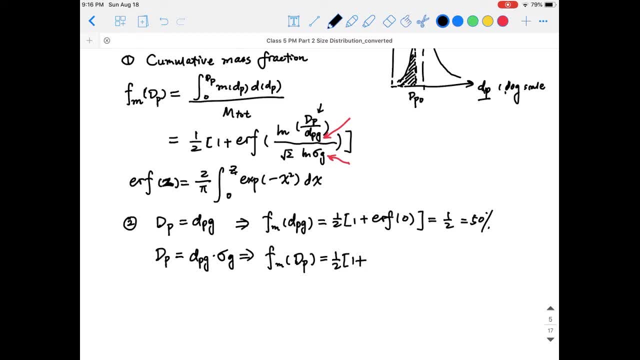 And just inside this term here we're going to just cancel out the dpg and have the sigma g here. Okay, And log sigma g, and log sigma g will get canceled out. So this will be error function of square root 1 over square root of 2.. 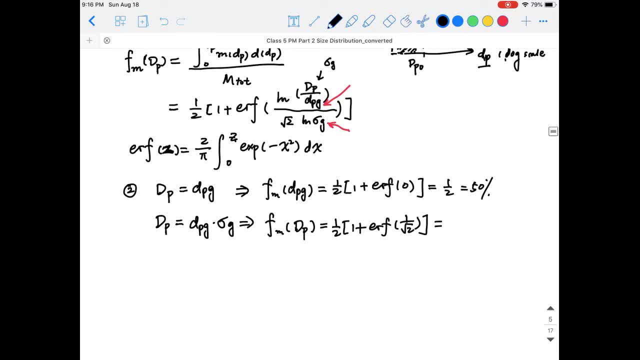 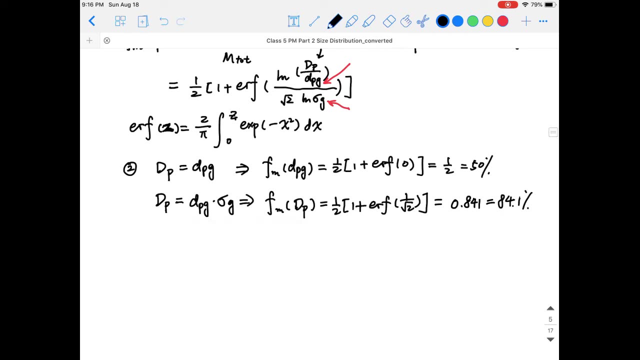 Okay, So everything is constant, It's just the numbers we can plug in, And this is going to be 0.841, which is 84.1%. So what this means is that when the particle size is equal to the geometric standard deviation multiplied by the geometric mean size, 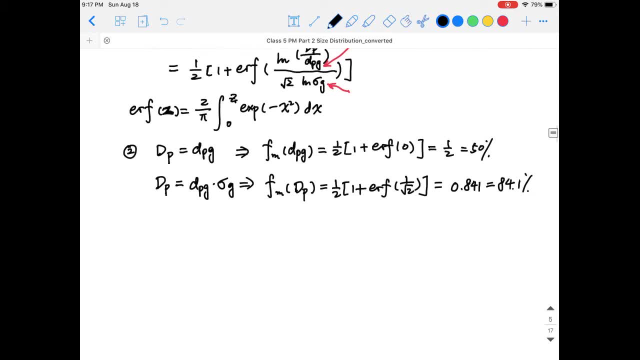 then the cumulative mass fraction will be 84.1%. Okay, And we can also try dpg divided by sigma g. Okay, And we can get. let's check what we can get. Okay, So if we plug in this term here, 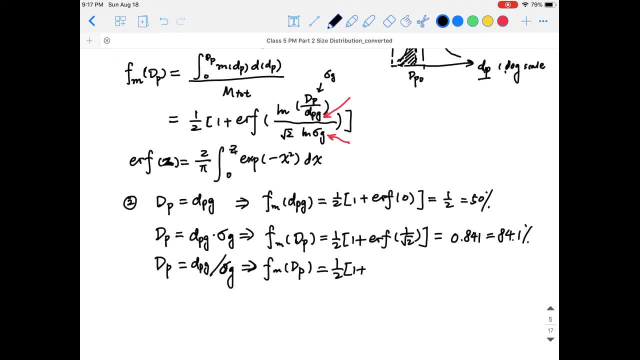 then it's going to give us log of 1 over sigma g, And log of 1 over sigma g is basically minus log sigma g. Okay, So that's going to give us minus 1 over square root of 2. And we can also calculate it. 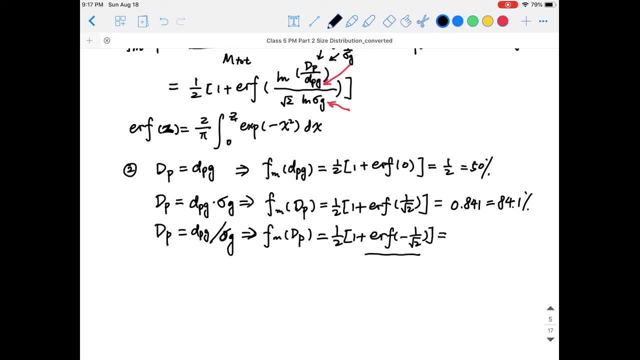 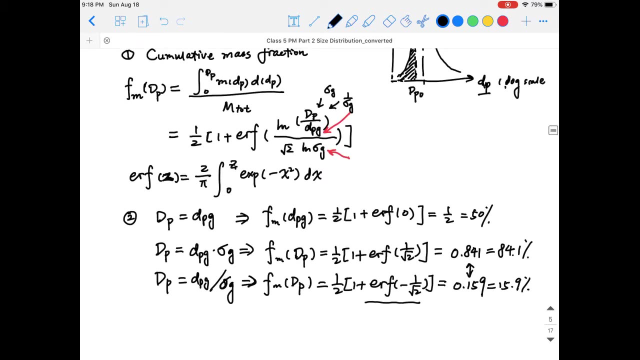 So these are all numbers now, Okay, And we can calculate the number. So this is going to be 0.159.. Okay, Which is 15.9%, And you can see that these two numbers are actually symmetric And this makes sense. 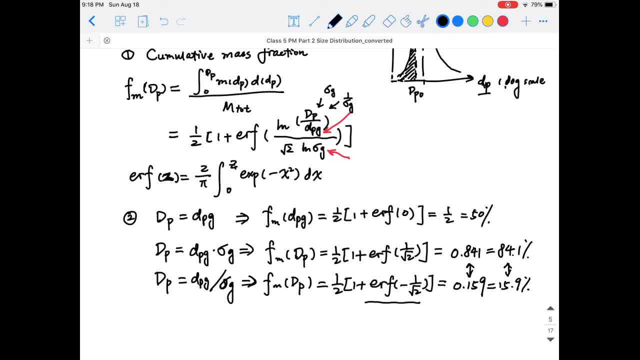 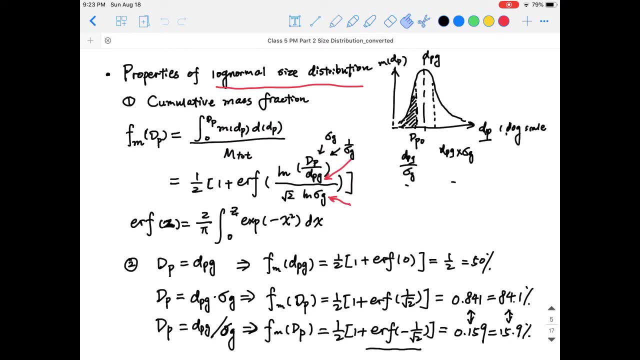 Right, It's symmetric. By symmetric I mean the sum or the addition of. by adding these numbers up, we're going to get 1.. And actually this makes sense Because for a logarithm, for a log-normal size distribution, 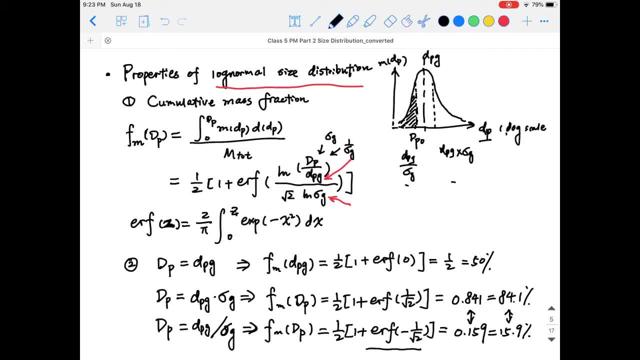 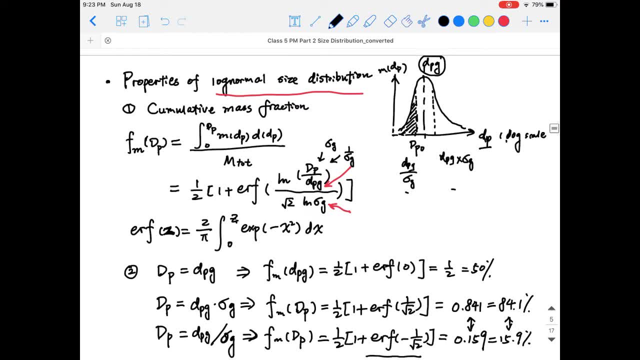 what happens at the peak actually corresponds to the size of the geometric mean. Okay, And since the x-scale or x-axis is in the log-scale, so the dpg divided by sigma g will be somewhere below, let's say, at this location. 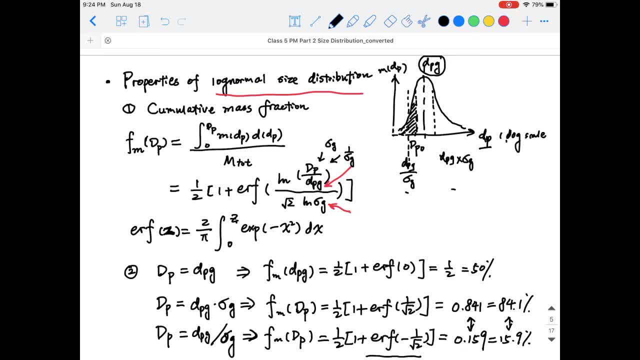 Okay, In this location And the dpg multiplied by sigma g, because it's in log-scale, then the ratio here, or the multiplication here, will be converted into linear scale, So it's going to be symmetric to the center axis. And now, if we talk about the area of the size distribution below the dpg divided by sigma g or dpg multiplied by sigma g, 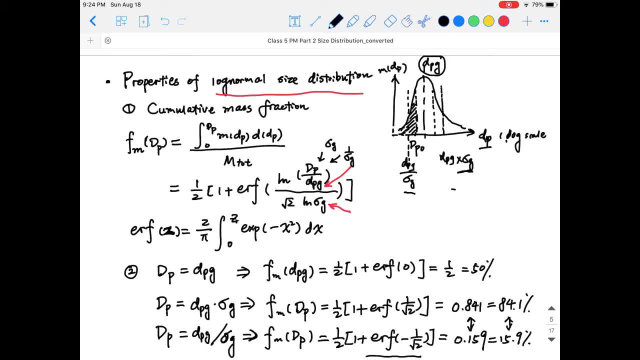 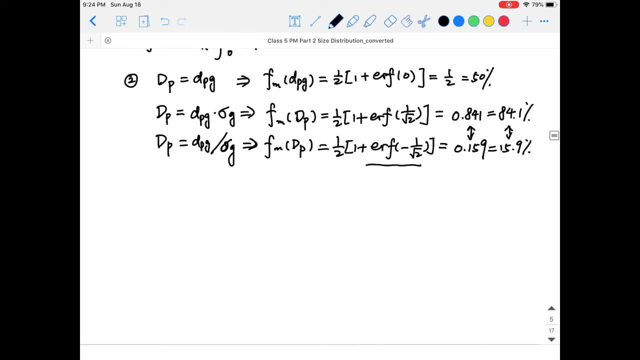 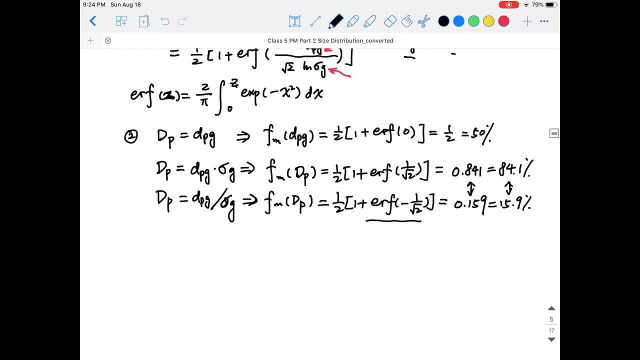 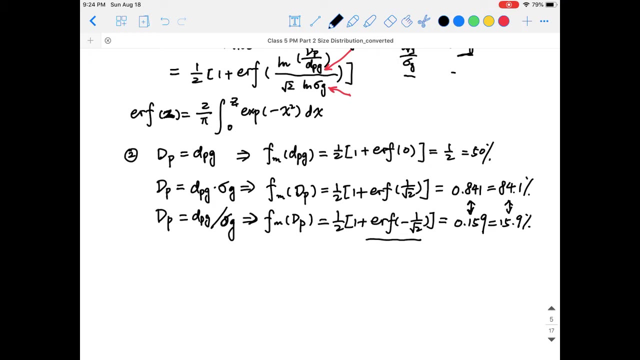 they're going to be reciprocal, Reciprocal. Okay, So the summation will be 1.. All right, So this actually helps us explain why these two mass fractions, or cumulative mass fractions, have these types of symmetric properties. Okay, So I'm pretty sure that, by going through all of these mathematic equations, 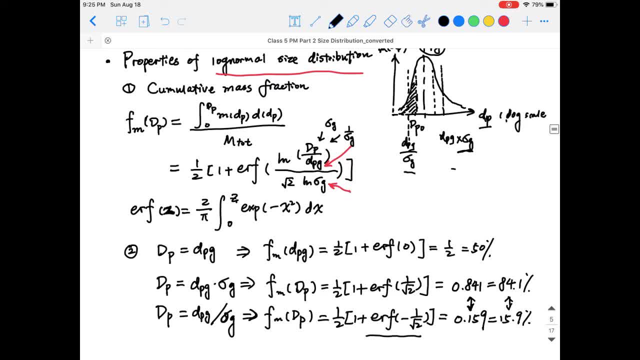 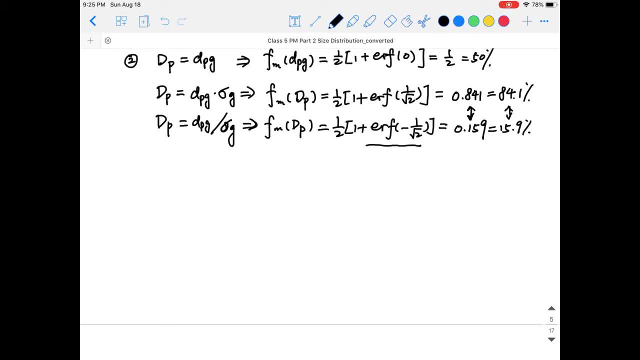 you are now a little bit puzzled Because these are not shown in the textbook, And you may wonder why we are going through this. Okay, Well, actually the textbook. what the textbook showed us is a very simple way of telling whether the size distribution is log-normal. 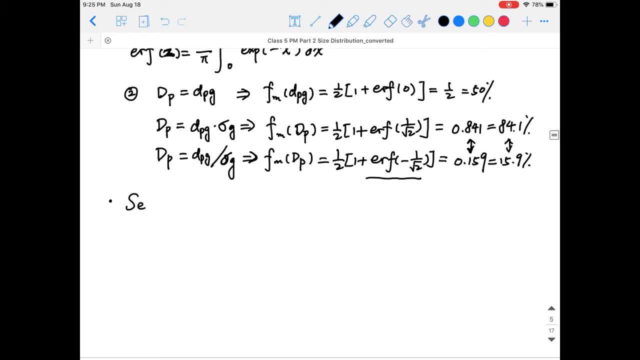 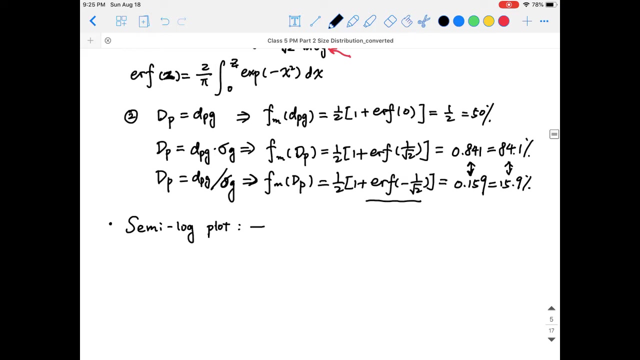 So it created a plot called a semi-log plot, But it really didn't explain the reason or the mechanism on why we can use such a semi-log plot to tell whether the size distribution follow the log-normal distribution. Okay, So this is also a more engineering way to tell whether the size distribution follows the log-normal distribution. 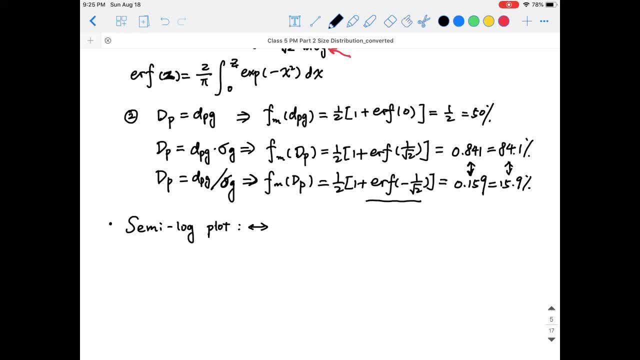 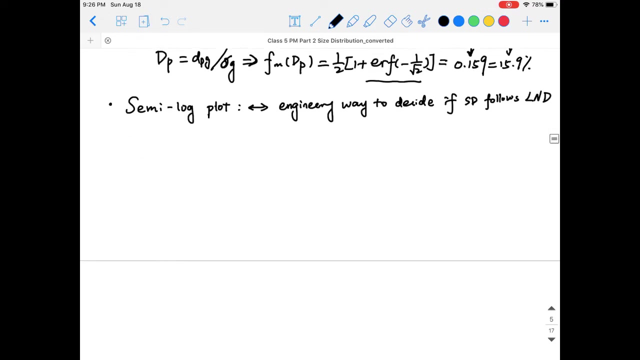 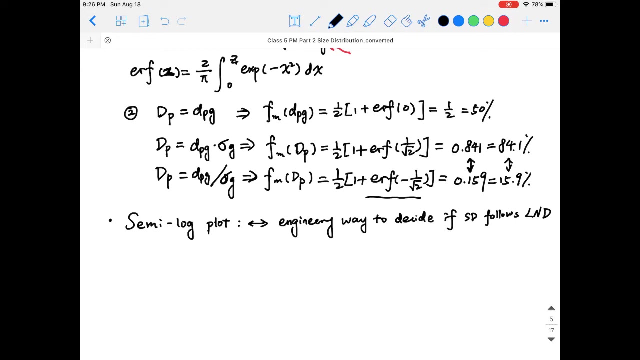 Okay, So engineering way to distinguish or to decide whether the size distribution, Let's say decide if size distribution follows the log-normal distribution- follows log normal distribution. okay, I'll just start to use these abbreviations. okay, so basically the background information or the mechanism. 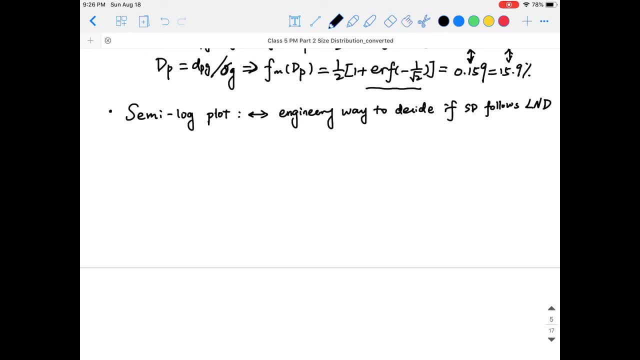 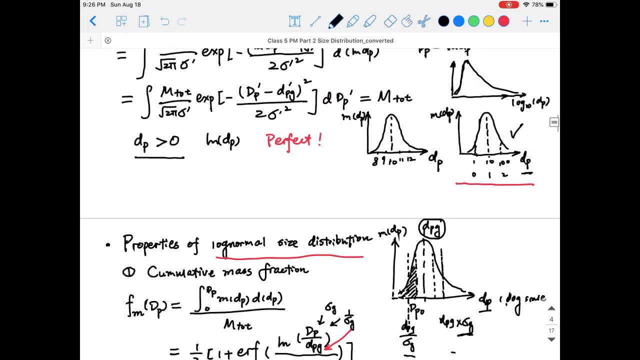 behind this semi log plot that's actually in this way. so let's see. so we can probably write on this section here. so let's say, if we want to plot the cumulative mass fraction as a function of particle size, okay, so what we're going to do is basically calculate this equation here as a function of particle. 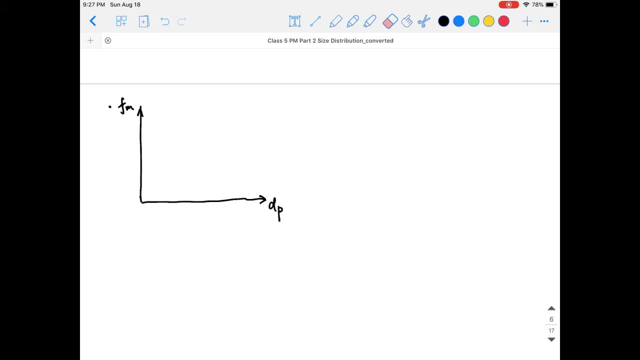 size. now let's start to use the capital DP here, to just be inconsistent with the. I don't know why this is not working, but let's just use large DP here. okay, so, and also, let's try to write this down: point one ten one hundred one. 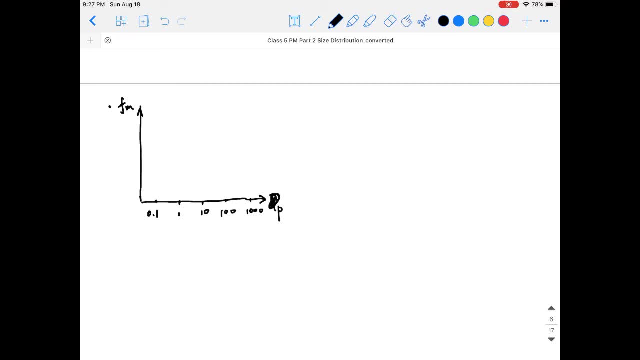 thousand. still, the x-axis is in the log term. so by plugging in these capitalized DP into the equation, what we're normally going to get is a function like this: so let's also assume that the particle size or the size distribution have a geometric mean DPG equal to 10 micrometer. so what's going? 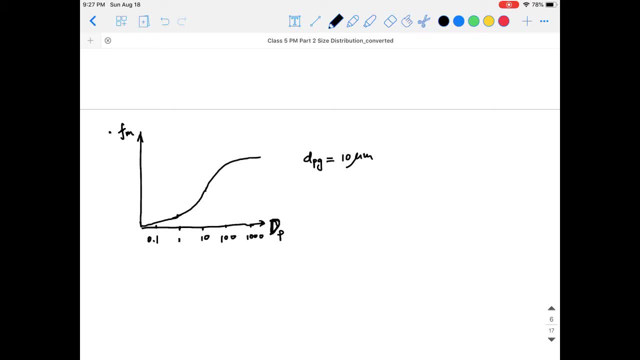 to happen is it's going to have this type of shape. okay, so let's say this is corresponding to one thousand and here, if the DP G is equal to ten micrometer, then at 10 micrometer this is going to be 50%, right, and this is going to be 100%. and let's say: if the DP G, DP G divide by Sigma G. 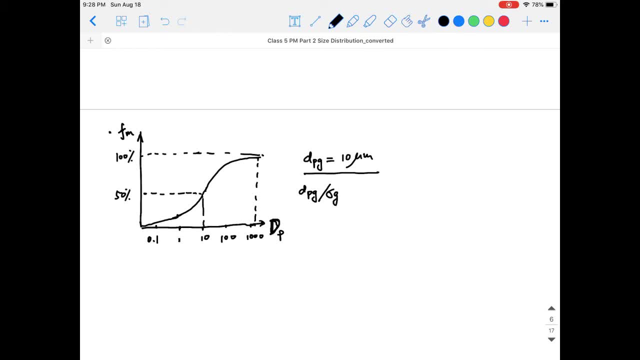 equal to. so basically, from this cumulative mass fraction we can also find what is the sigma G. okay, so now we can easily find the cumulative mass fraction of 15.9 percent. that is going to be around or below 1 third of the 50 percent. so it's going to be something like this: okay, and 85 percent, that is. 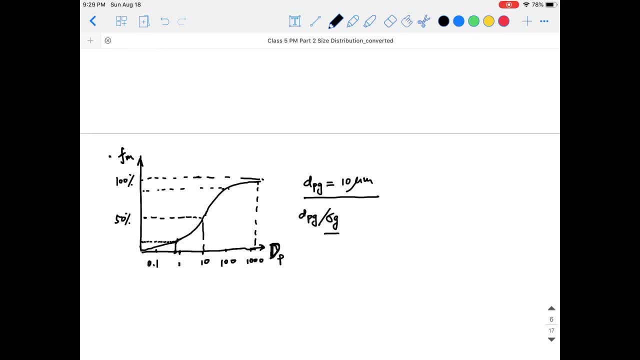 going to be somewhere here. okay, so we can find these locations. and then, and then we, by using these values- let's assume that here it's around- say what point nine? let's say, assume that it's point nine here: 0.9 micrometer. So by using this value here, you can know that sigma G is equal. 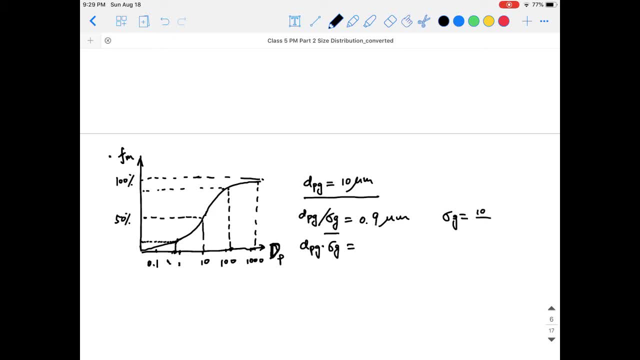 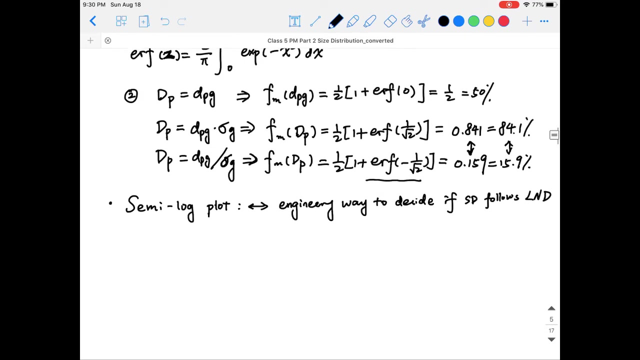 to 10 divided by 0.9, okay, Or by using this value here we can also calculate another sigma G and basically we can further average these sigma G values and then get the real sigma G. okay, But this is still not convenient enough. so we: 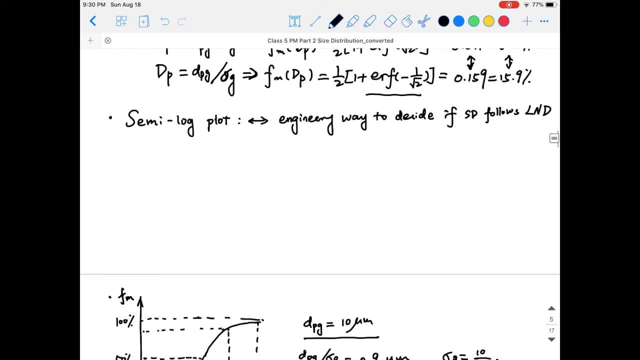 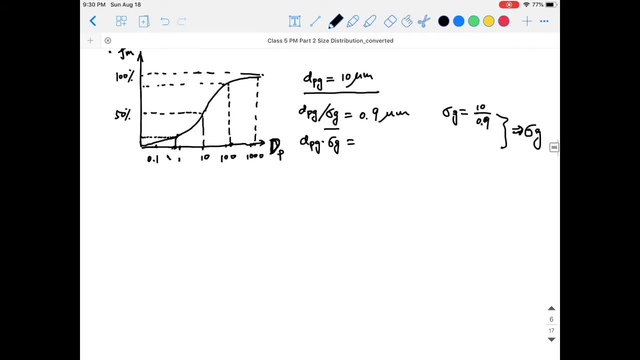 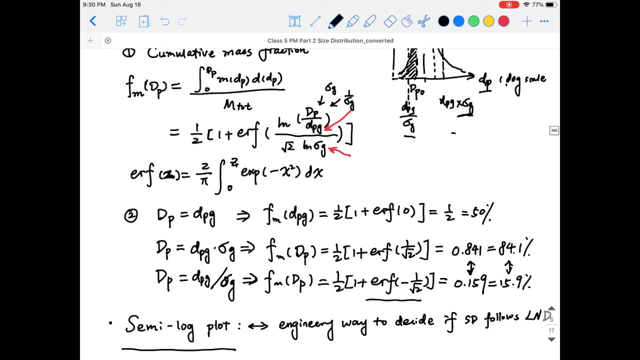 can try to borrow this similar idea and then create this such a semilog, a semilog plot that shows this relationship in a linear scale. So now let's have another look at the cumulative mass fraction equation here. So what we're doing here is we're going to do a simulation of this. So this is the 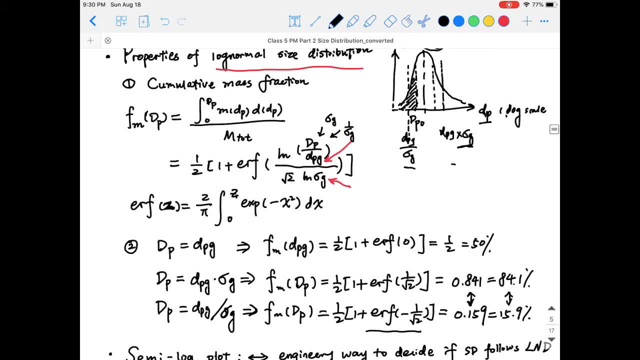 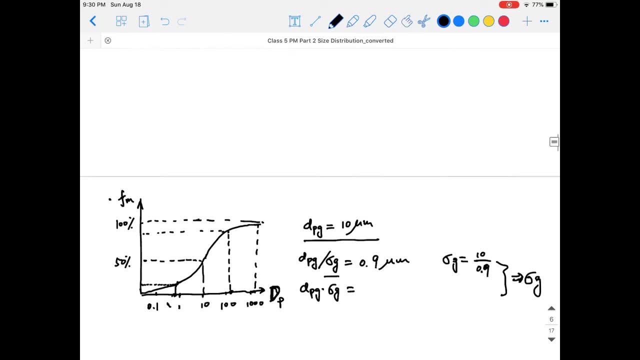 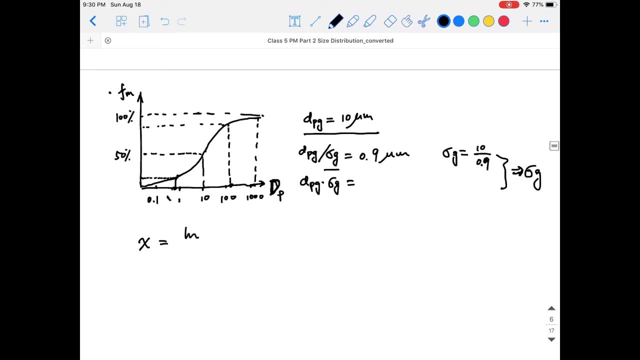 now we can do is we're going to assume this term here to be x. So what we're trying to do is that to set x equal to log dp divided by dpg, and this is divided by square root of 2 log sigma g. And what we can do is we're going to make another plot that shows fm as a function of x. and this is going to be quite similar to dp. So what we're going to do is we're going to assume this term here to be x. So what we're going to do is we're going to make another plot that shows fm as a function of x, and this is: 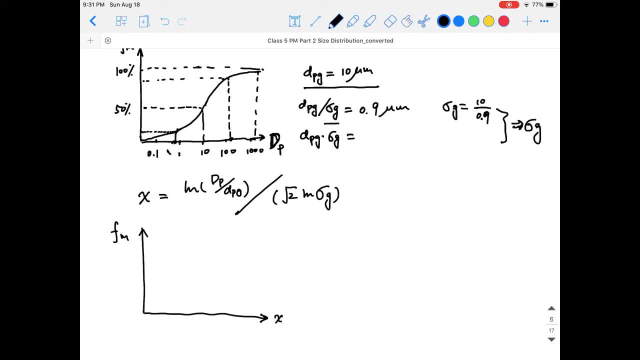 going to be quite similar to dp, because you can see that clearly, right now we're showing the dp in the log normal, in the log scale, and the x is actually the log of dp. So in terms of the x, then the x will be in the linear scale, right, And this is what we're going to show in here. 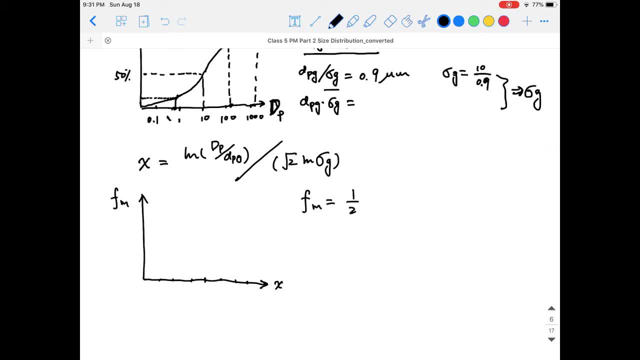 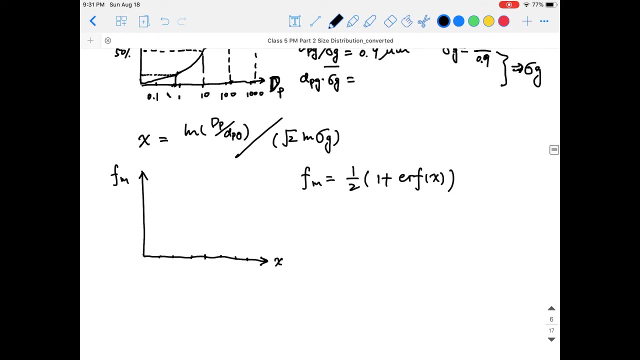 So basically, if we plug in, that's going to be 1 over 2 multiplied by 1, plus error function of x. okay, and this is what we have plot. by using the MATLAB or any Excel we can create such a plot. okay, so when the X is equal to 0, which means that DP is equal to, 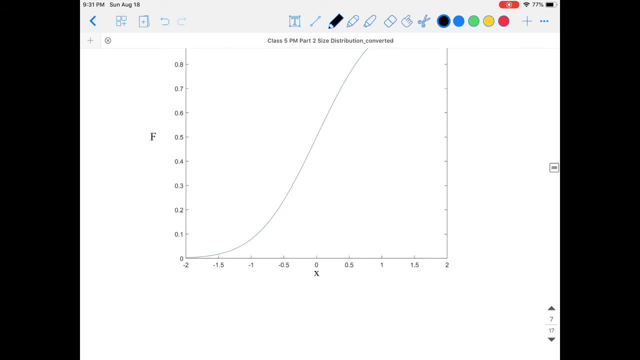 DPG here, then it's going to have the value of 0.5. okay, so this still makes sense, all right, okay, so now what we can do is let's start to make some marks. okay, so I think the the format is definitely format is definitely creating. 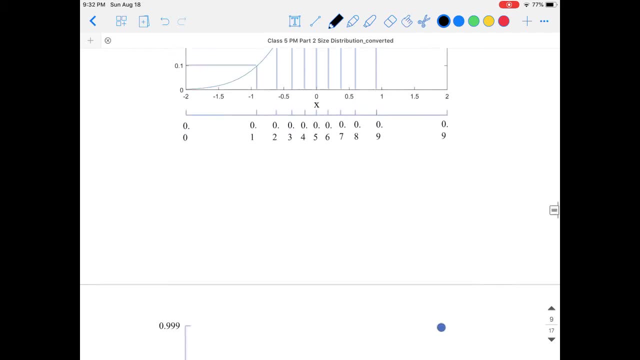 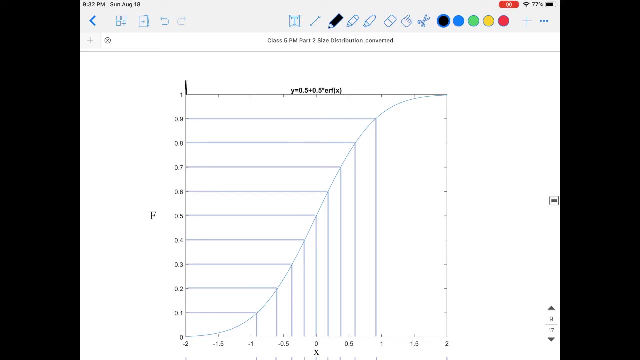 a little trouble here, but we can try to distinguish the marks by this plot. so on the white line here we can see that we have a little bit of a problem with the white line here. we can try to distinguish the marks by this plot. so on, axis is actually showing the cumulative mass fraction. right, it's from 0 to 100. 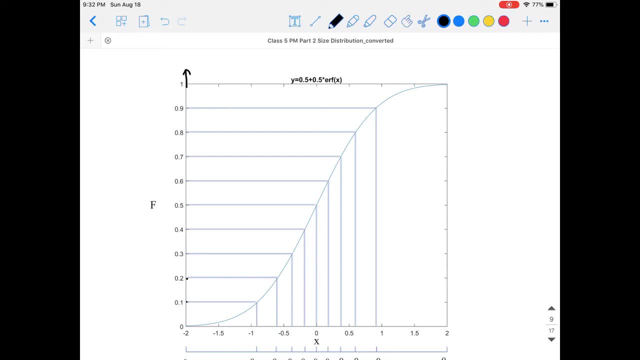 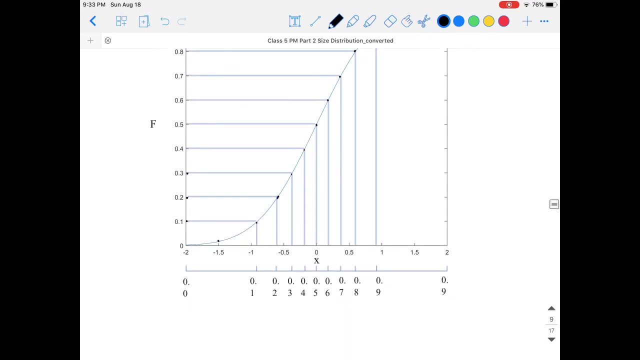 percent, and what we can do is that we can mark out the location from in, basically in a linear scale from point 1 point 2 and 2, point 9, and we can then make corresponding marks onto this log, normal or this cumulative mass fraction value here. okay, we can mark these, we can mark these values out and then first, 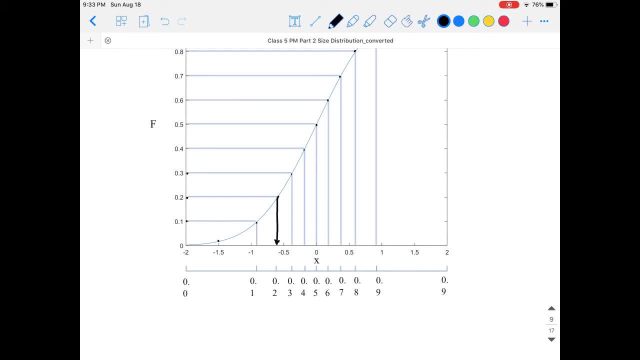 further impose them or draw these corresponding cumulative mass fractions onto the x-axis. okay, and now it's going to show the value of point 1, point 2 and 2, point 9, and then we can probably also try to plot some other values, because the value for X equal to minus 2 is not exactly 0, right, when the X is equal to. 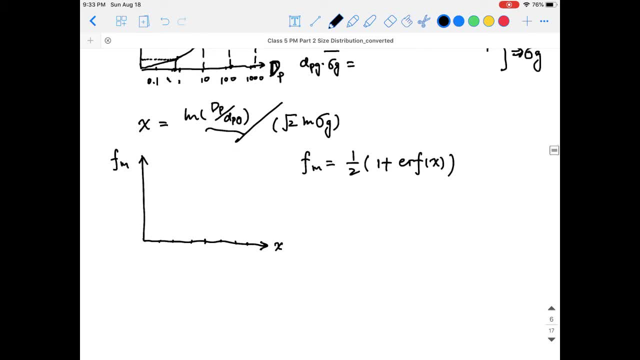 minus 2 is equal to minus 2. the cumulative mass fraction is still going to have some values, and this value is actually point 0 0, 1, which is not point 0 here, and this is point 99: 0, 0, 0, 0, 1, 999. okay, so now, what we did is that we 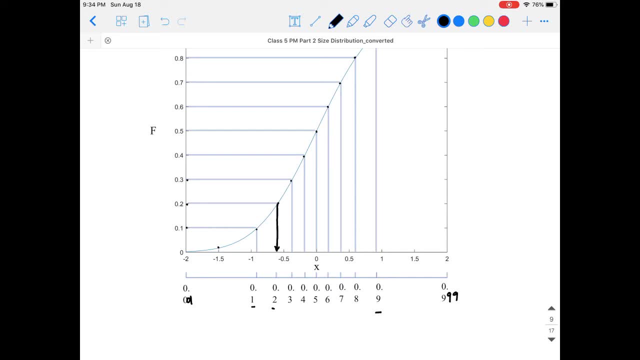 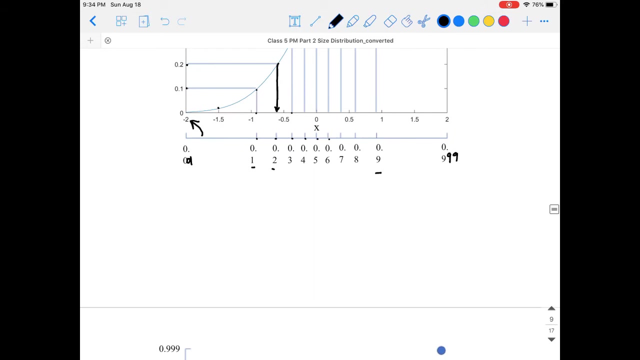 basically convert or made another axis that shows the cumulative mass fraction at the corresponding x values correct, and then let's use this new axis- X, C, Y axis- and let's see what happens. okay, so you can see that, for this new X is here. it's actually quite crowded at the X location of 0, right? so this is what. 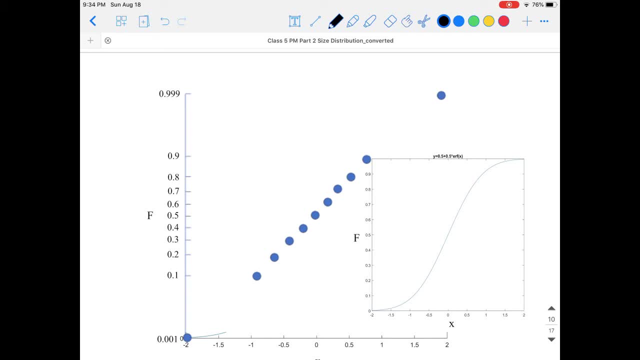 I have done. You can see that here is actually quite crowded and this is quite here is quite crowded and here is quite open in terms of these values. okay, So this is new axis, And now let's plot this new cumulative mass. 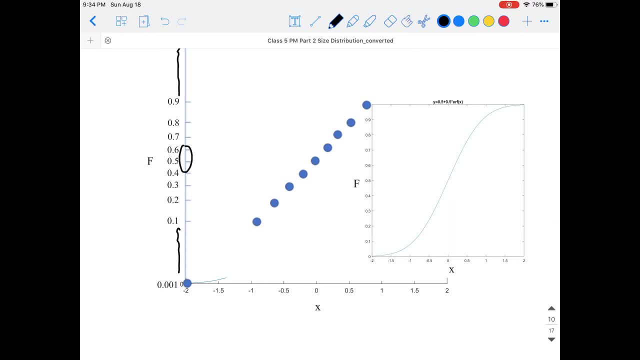 fraction onto this picture here, onto this figure here, okay, So let's see first at point 1, it's going to have a value of, let's say, 0.9,. okay, Which is exactly this point here, okay. 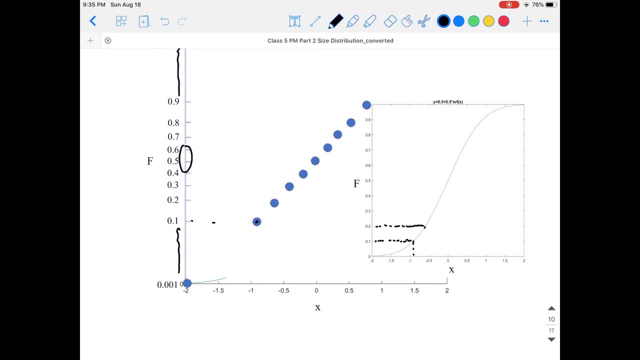 Point 2 of the y-axis is going to have a value of minus 0.6, that is this point here. okay, Point 3 is going to have a value of minus 0.3, minus 0.3 is going to have this value. 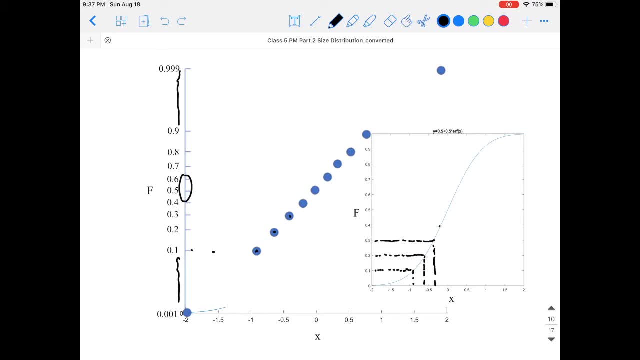 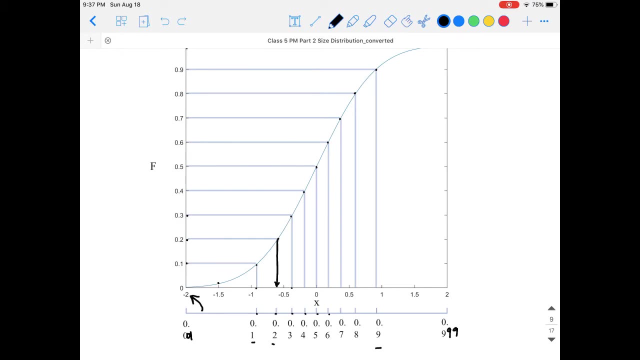 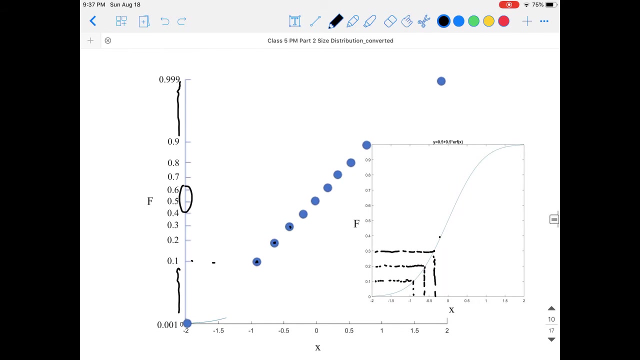 So what happens in this new plot is that actually these existing data points on these, on this complex curve here, is actually going to be converted into. it's going to be converted into a straight line data points onto a straight line by using this new axis here. So, instead of using the 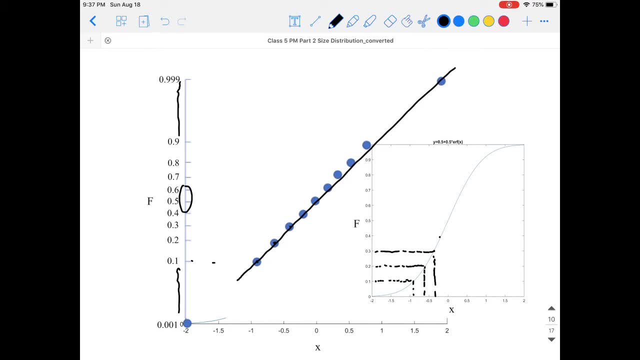 linear axis that's showing the cumulative mass fraction. we did a little bit trick So that if a size distribution satisfies a lognormal distribution, it's going to show a straight line onto this new graph. and we call this new graph as the semi-log graph. 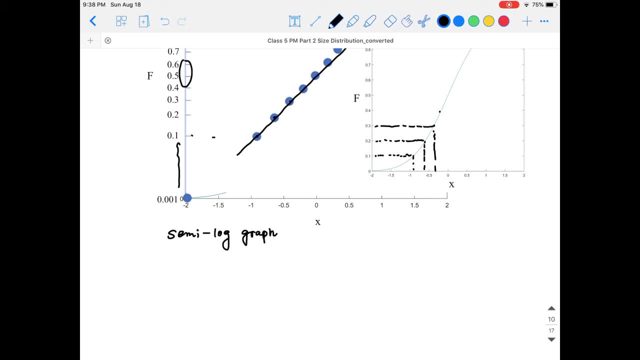 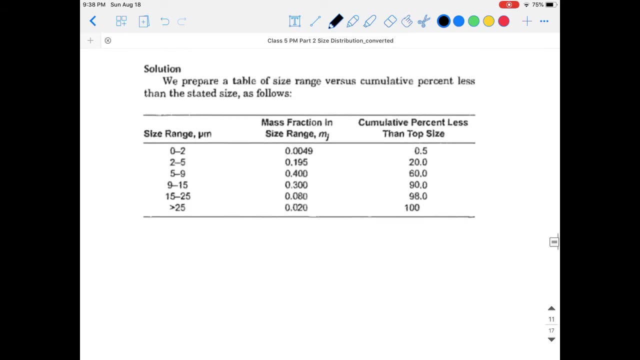 And actually online you can download quite many different types of semi log graphs, but this is actually a quite special one, So let me show you. Okay. so with this I'm doing a very little bit of какую. directly jump into the graph or the final graph. here The final graph. 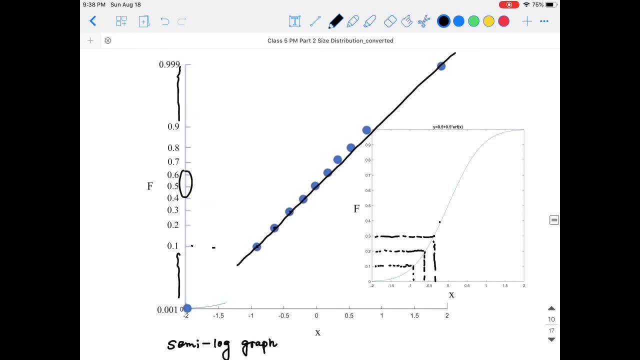 is actually a little bit different from this graph either, because on the y-axis we're showing the cumulative mass fraction, On the x-axis we're showing the x. We know that the x is actually the log of the particle size And in real situation, in the engineering plot. 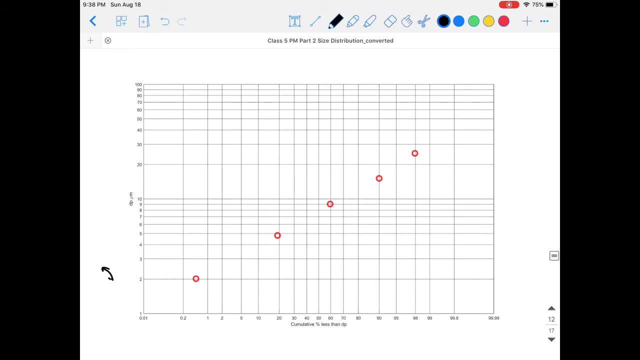 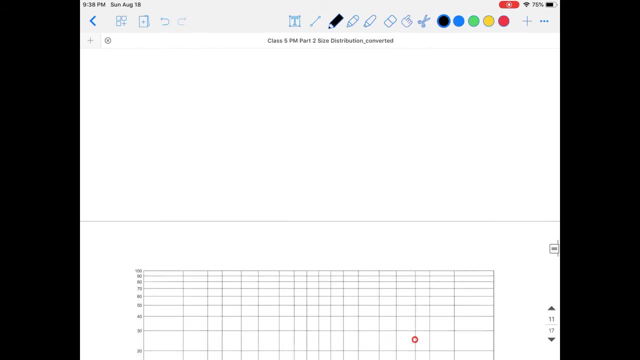 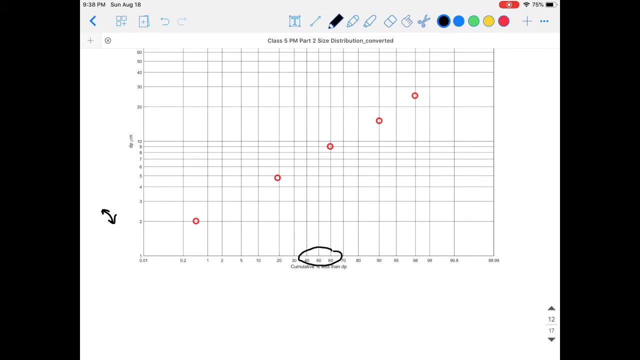 we actually switch that y-axis and x-axis again, because here the y-axis is the mass fraction And now we convert that into here. You see, it's quite crowded at 50% and it's quite open at both ends, And on the y-axis we're not using the x. 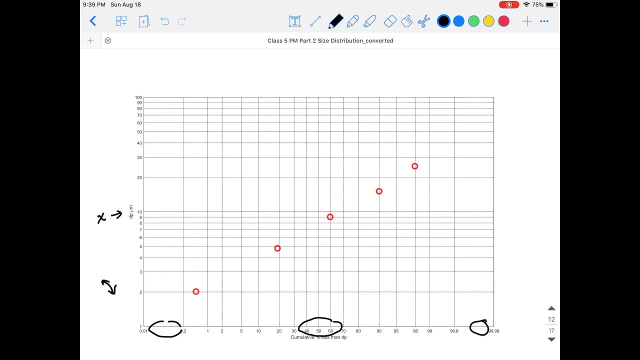 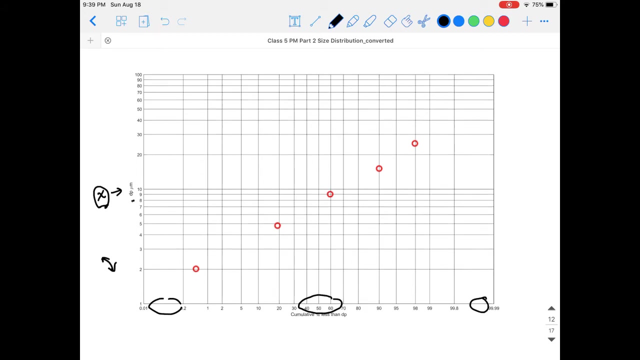 We're actually using the particle size, But there's no difference, because the x is the log of dp, which is in linear, which is actually in linear scale for the x. Okay, So I hope that by doing this type of derivation here, we can try to understand why we're doing. 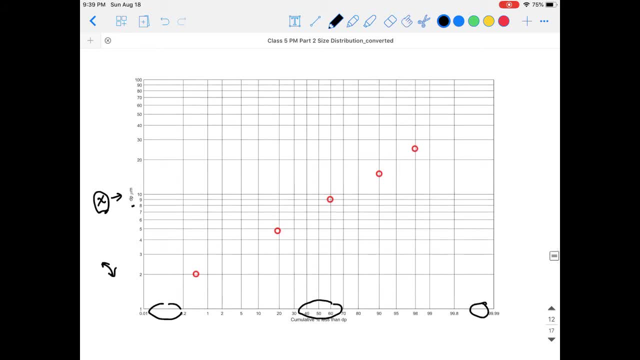 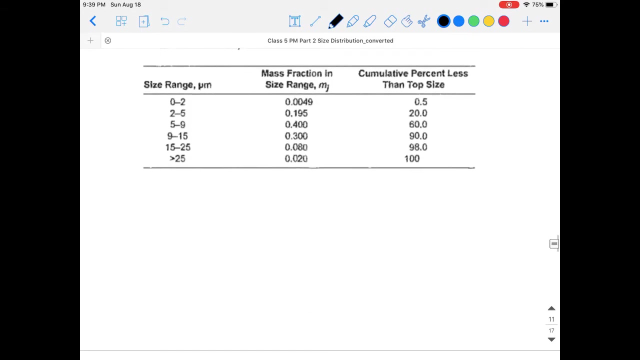 why we can use such a semi-log plot to create or to study the, to study the size distribution of particles, And also, as I mentioned, although we call this as a semi-log graph, actually if you just google it online, there are actually different types of semi-log. 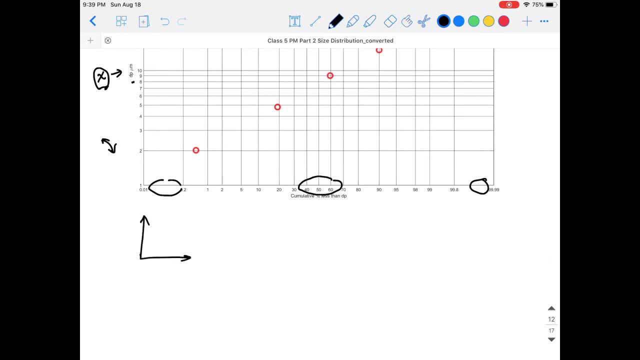 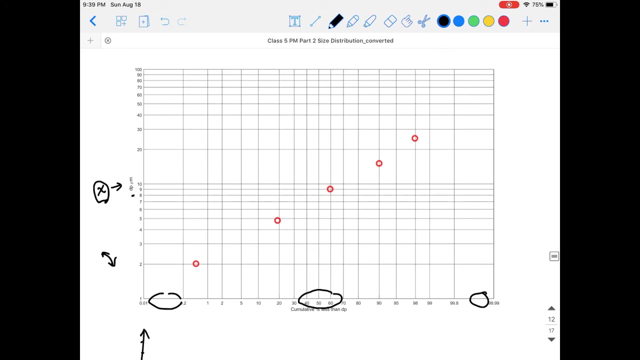 Some of them are actually showing the log in the x-axis, log scale in the x-axis, but the y-axis is still linear. Some of them are showing the y-axis as log, but the x-axis is linear. But for this semi-log plot we can see that on the y-axis. 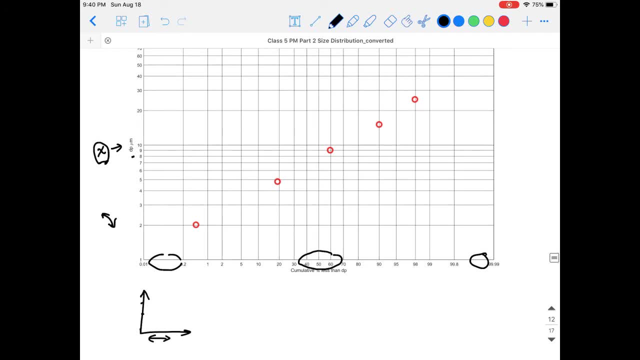 it's in log scale, but x-axis is not linear, right? So this is a. I would have to say that this is a very special type of the semi-log graph that's used for distribution of particles, That's used for determining the log-normal distributions. 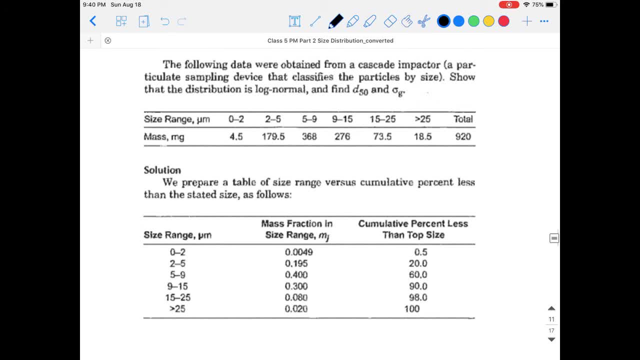 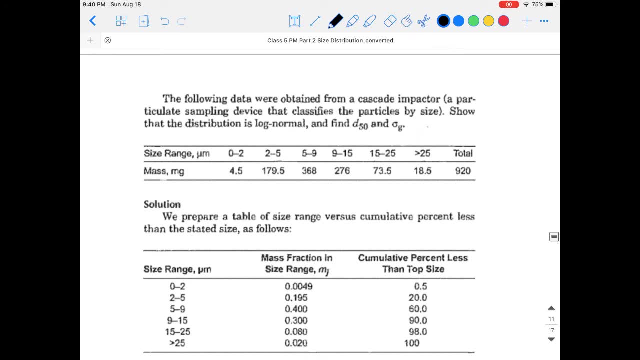 And actually we can go through an example to see why that is the case. Okay, So let's look at this example here. I think this should be the example of 3.1 on the textbook, but I may be wrong, So let's say the following data were obtained from a cascade impactor. 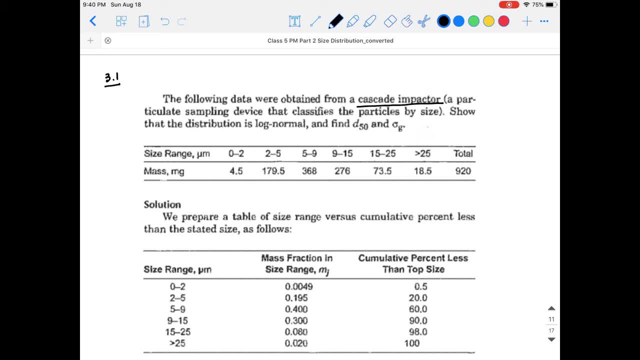 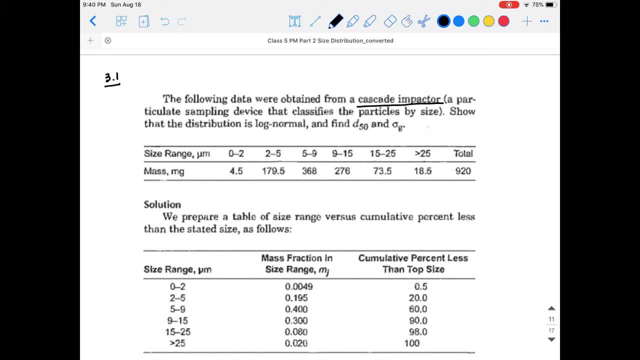 Or the mass of the particles in different size ranges, And show that the size. it wants you to show that the size distribution is log-normal and wants you to find the dp50 in sigma g. Okay, So the given data is shown in this way. 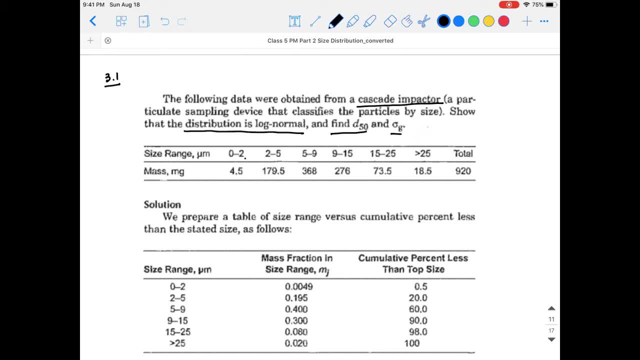 It gives you the mass size range: 0 to 2,, 2 to 5,, 5 to 9.. So basically, it's the different, it's in different stages And we know that for the 0 to 2, it's actually measured by the mass. 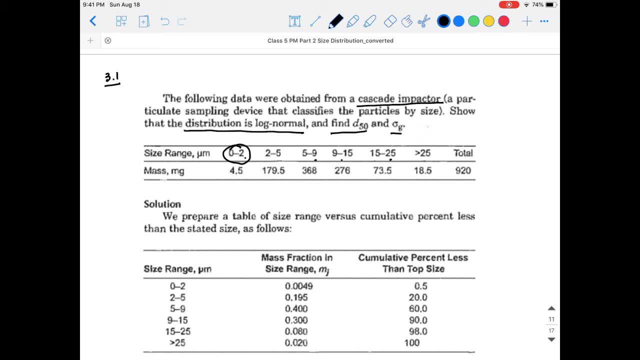 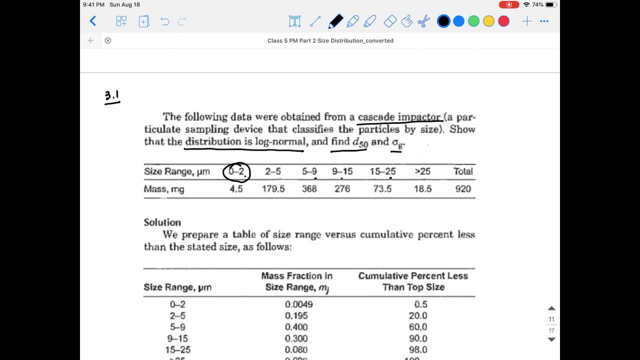 It's measured by a filter, right, It's not measured by the impactor stage, Because for the particles of infinitely small size, it's not going to be able to get collected by an impactor anymore, And the particles larger than 25 micrometer is the first stage. 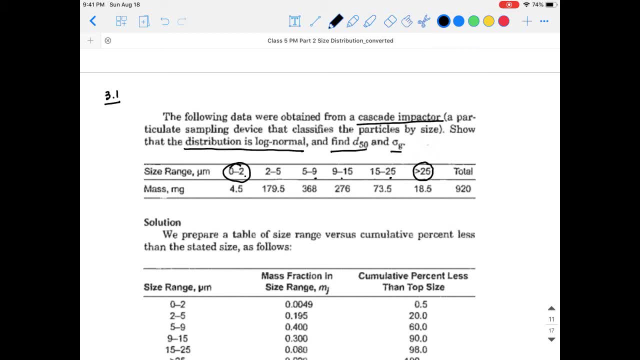 So let's say, if I ask you, how many stages are there in the cascade impactor? we know that there are one, two, three, four, five, Five, Five stages. Right Now, let's go back to the topic. It wants you to calculate, it wants you to prove that the size distribution is log-normal. 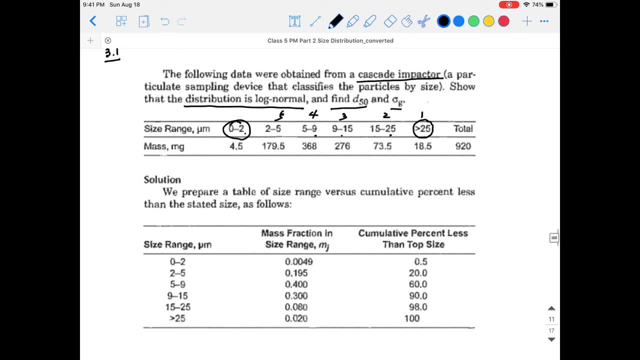 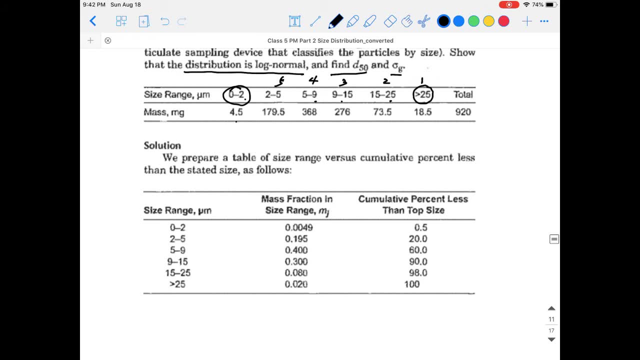 So what we do first is we measure or we calculate the mass fraction in different size ranges- Let's say it's 0 to 2,, 2 to 5, and 2 to 25.- And calculate the corresponding mass fraction in each state. 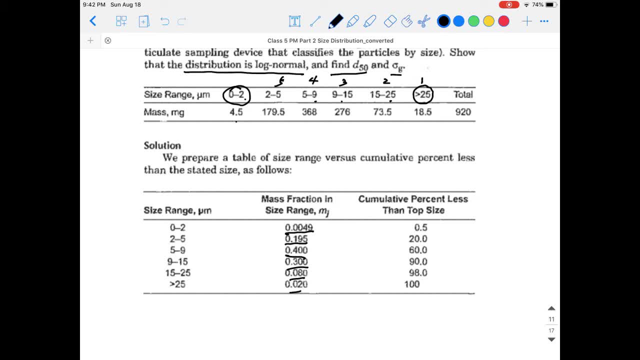 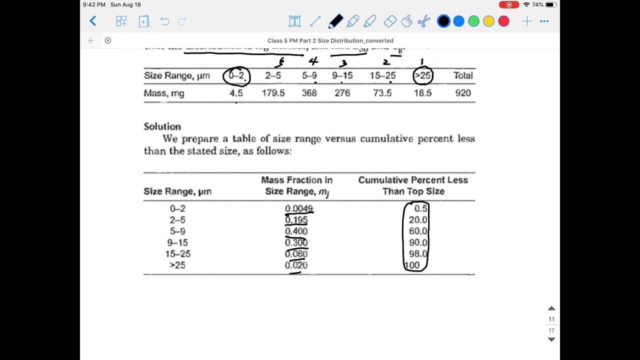 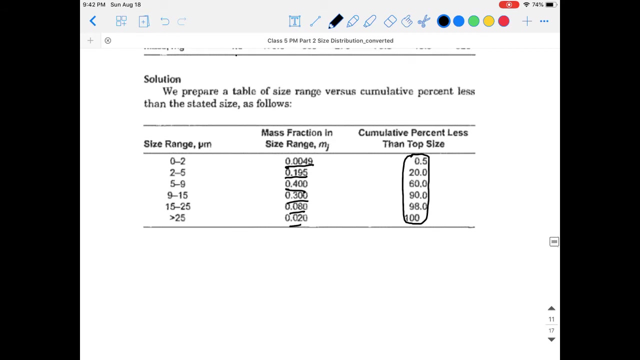 And then calculate the cumulative percent or cumulative mass fraction at each stage. And now we can use that semi-log graph to prove whether it is, or to prove or disprove the size distribution is a log-normal, follows log-normal distribution. So now let's look at the first data point. 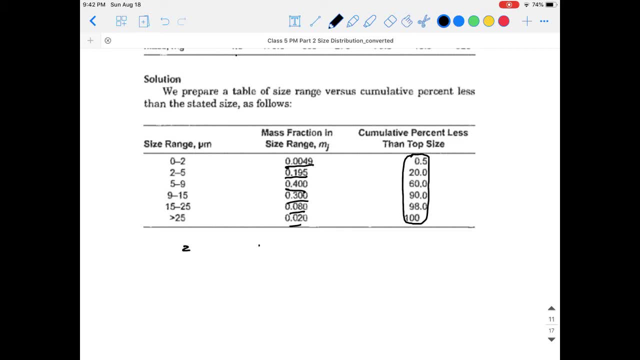 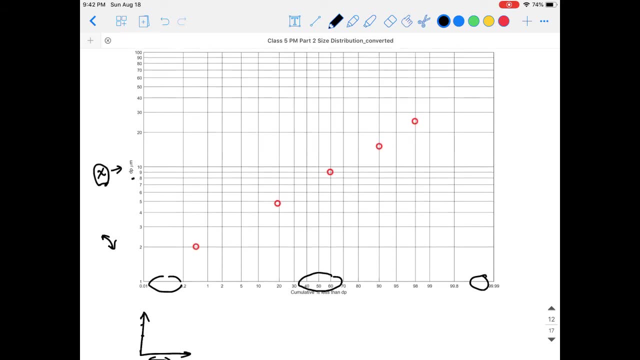 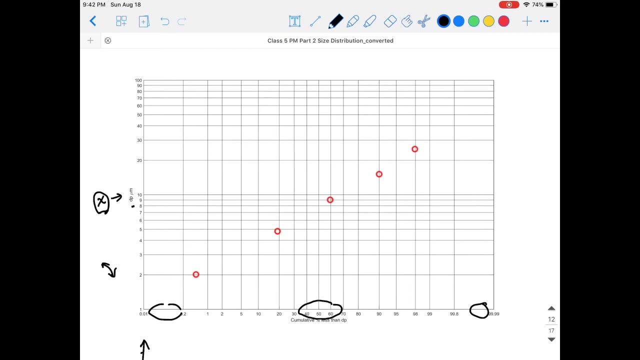 That's going to be at 2 micrometer And the mass fraction is 0.5, right? So if we come here- and luckily the PDF is not showing a clean graph here, So these are pre-embedded here, But let's just go through this process again. 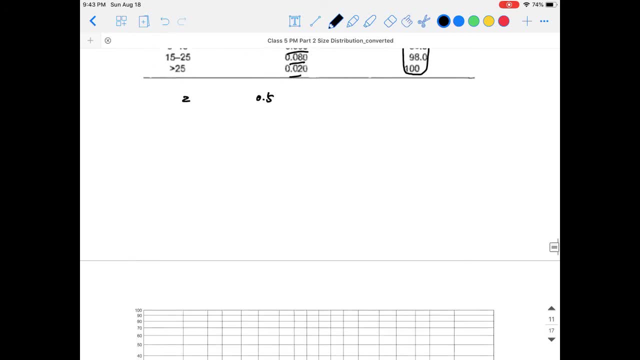 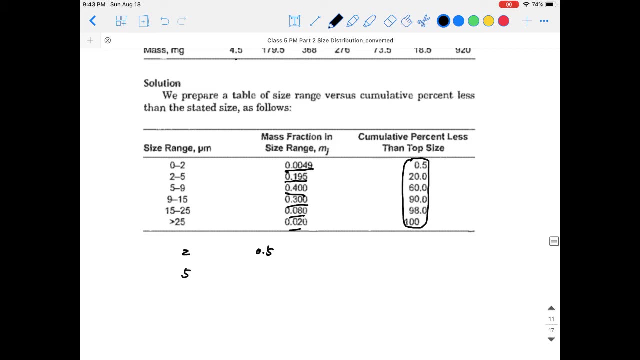 So 2 micrometer is 0.5%. We can find this third point. It's here, Okay. And the second data point is 5 micrometer, 0.5.. It's 20% And we can find the 5.. 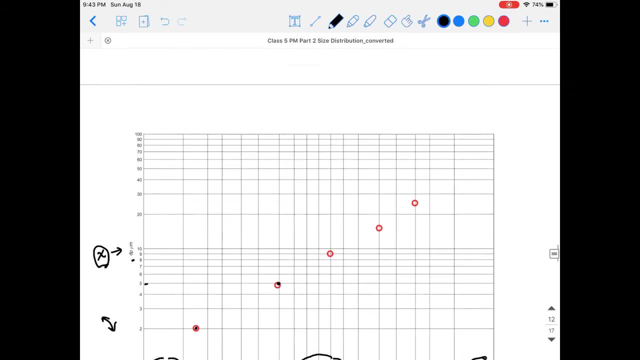 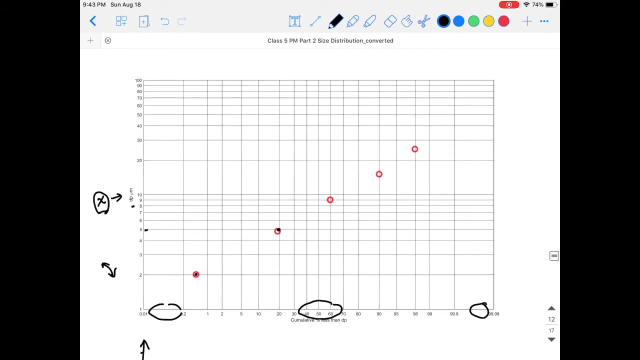 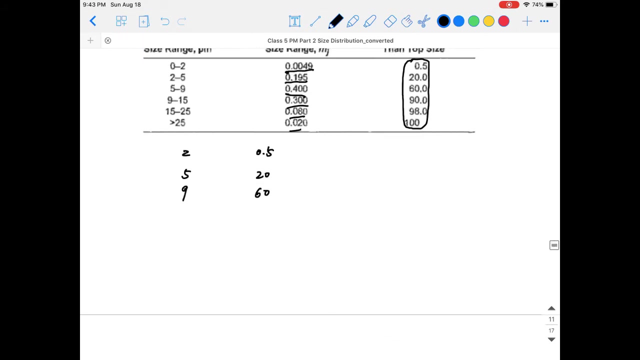 And 20 is here. It's a little bit off here, but I can still draw it out. At 9 micrometer, it's 60%. I should find 9 and 60.. That's here. And 15 micrometer, that's 90%. 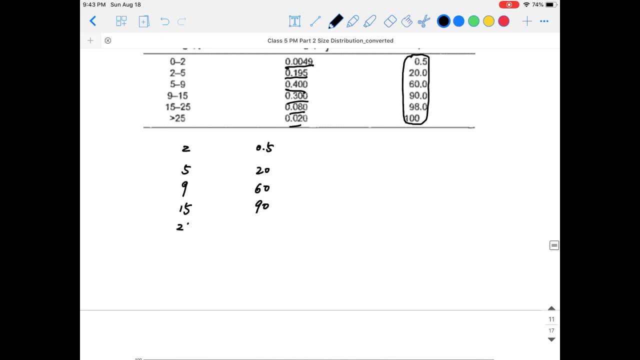 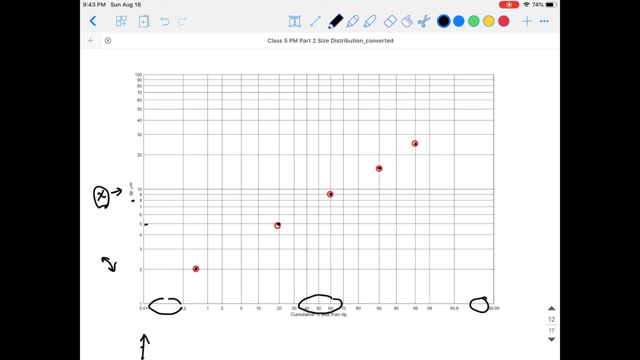 That is going to be the data point here, And finally 25.. That is 98.. 25 is somewhere here. 98 is here, So let's see if it's a straight line. It is a straight line, right. 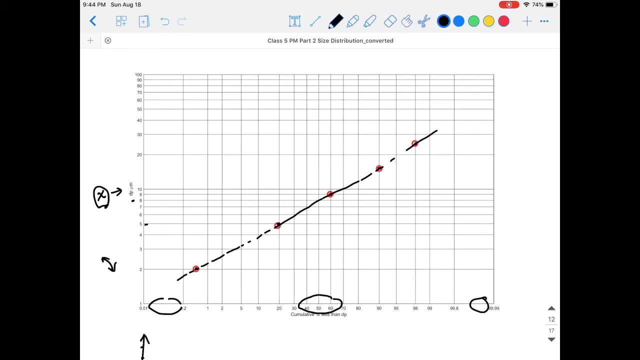 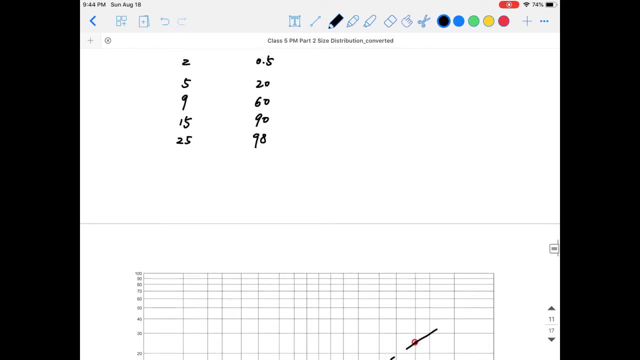 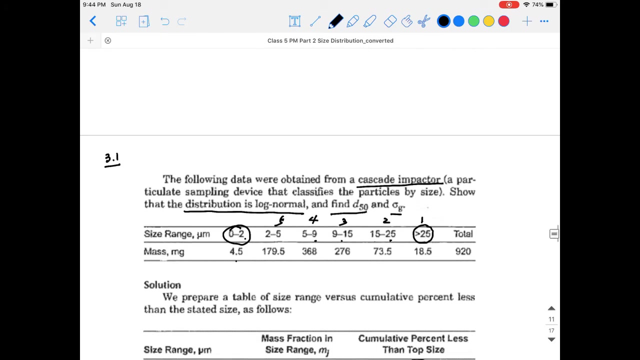 Although it's not perfect, but it's actually showing that the size distribution follows the log-normal distribution. Okay, So I hope this makes sense And actually, by using this semi-log plot we can get more information. Let's say what it also asks for. 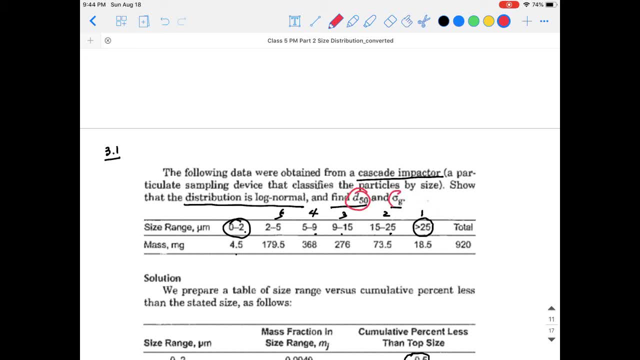 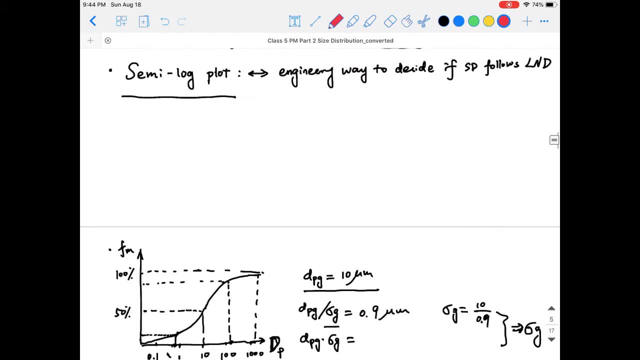 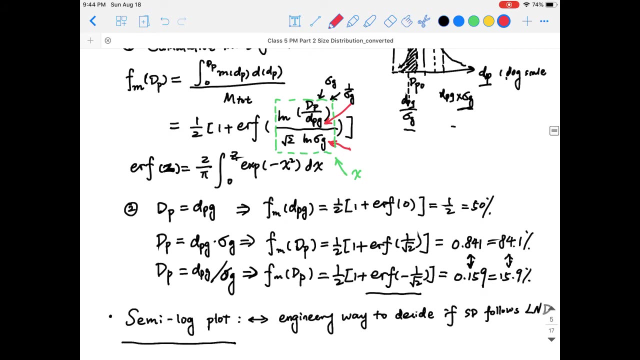 Okay, So it also asks for the DP50 and sigma G. How we can find that Now we can use the properties of the log-normal distributions right, If we recall here the first proper Or the second property. When the DP is equal to DPG, the cumulative mass fraction is 50%. 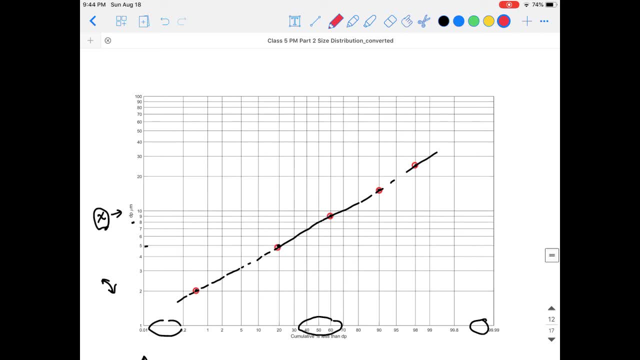 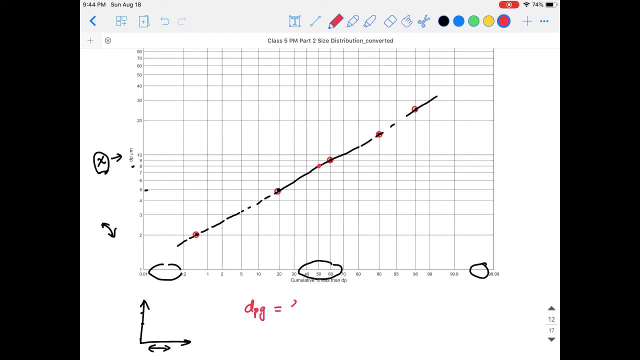 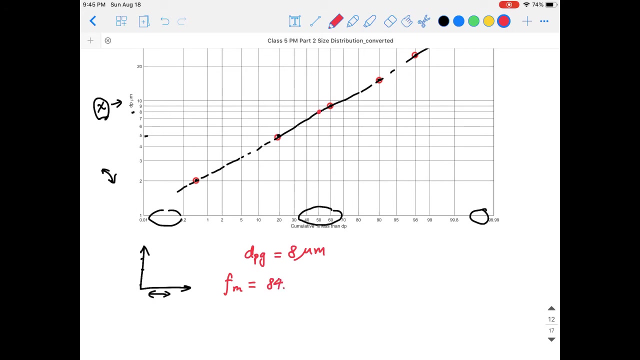 Okay, Let's just look at 50%. It's going to be here, Okay, Which means that the DPG is equal to 8 micrometer. Okay. So what about sigma G? We know that, at When the cumulative mass fraction is 84.1%, the DPG multiplied by sigma G, it's a size 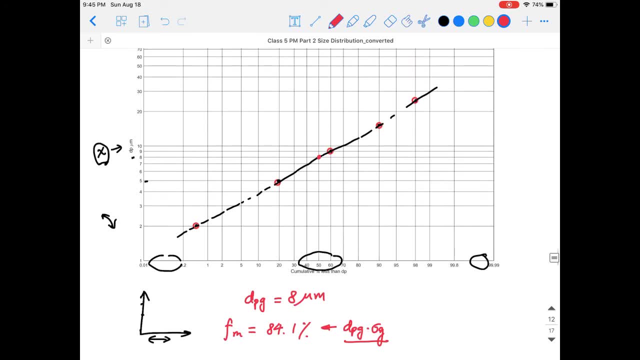 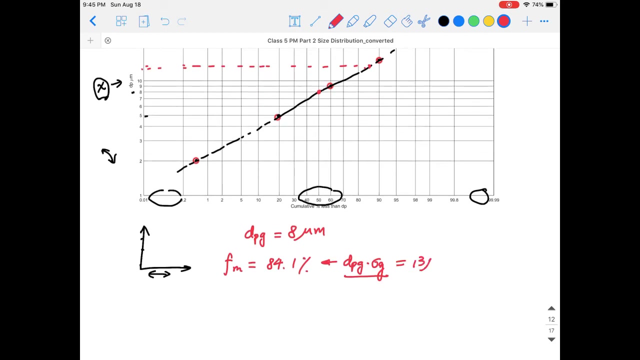 that corresponds to this mass fraction. So let's just look at the 84%. okay, That is somewhere here Which is around 84%, Let's say Which is around 13.. I would say 13 micrometer, Okay. 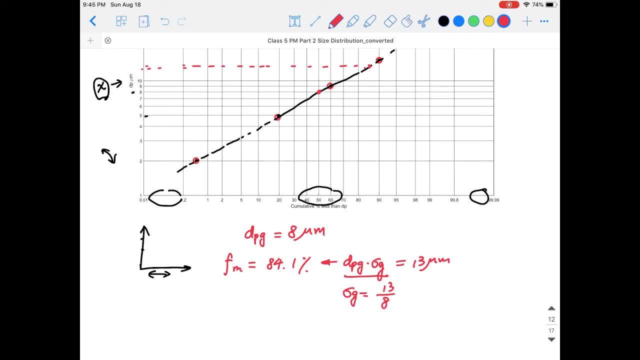 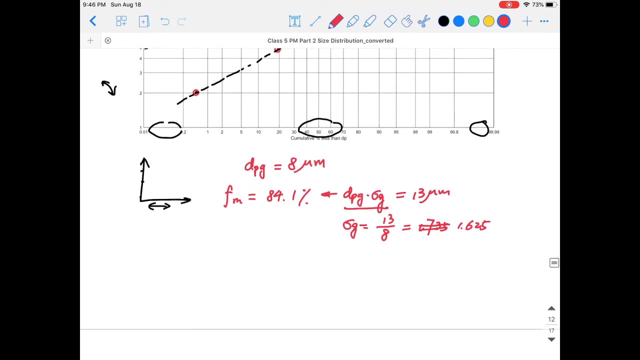 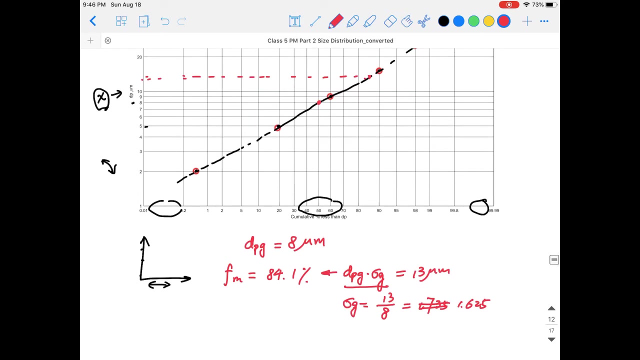 So the sigma G will be equal to 13 divided by 8. And that is 1.735.. Okay, No, no, it's 1.625,. okay, And if you're still not happy with this answer here, you can also do use the lower end. 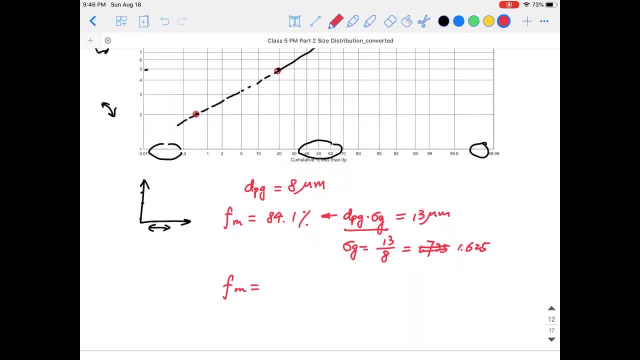 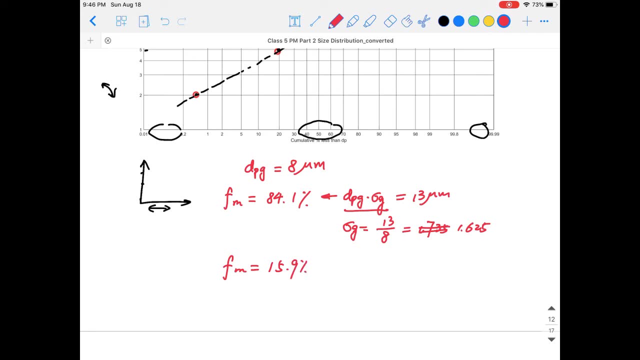 We know that when the FM is equal to What's that? 19.7 divided by 4.5,? okay, That's one 6.25.. Okay, 15.9%. okay, it's always reciprocal, right? it's 1 minus 84.1, that's 15.9%, and that. 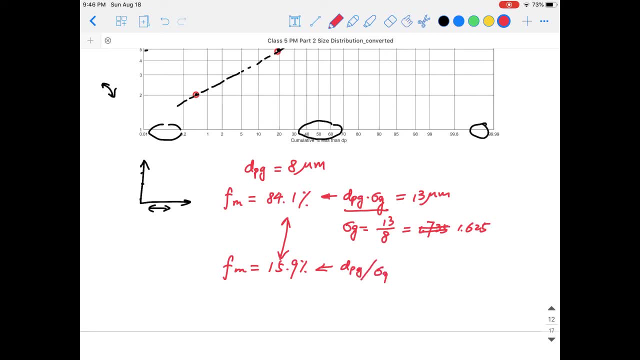 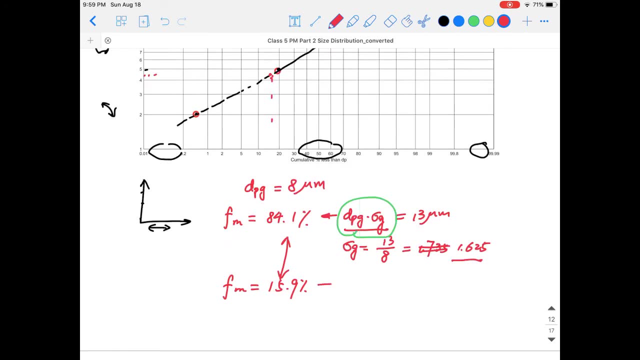 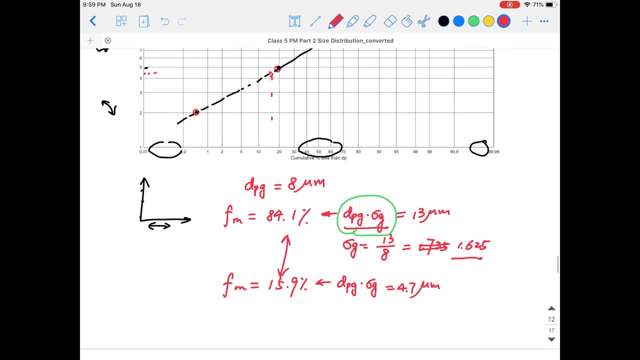 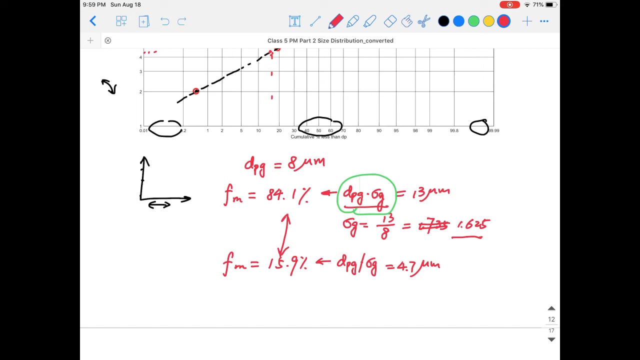 is corresponding to the size dpg divided by Sigma G. okay, so this is going to be around 4.7, 4.7 micrometer. okay, so we can. we can actually calculate the Sigma G from this value. that is going to be 8 divided by 4.7 micrometer, and this is: 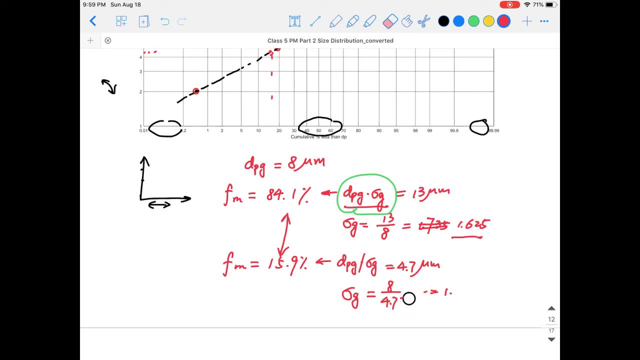 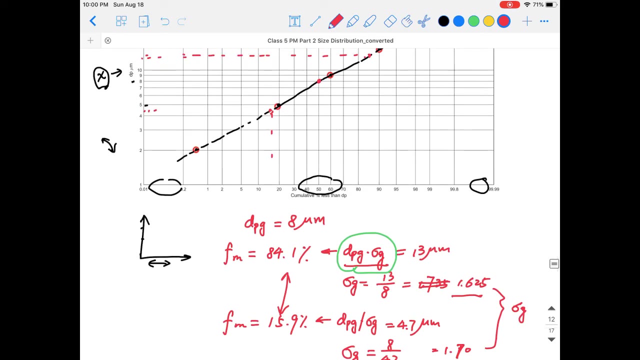 4.7. we actually don't need a unit here, because for the geometric standard deviation it is unit less and that is around 1.70. okay, you can see that there are some difference between the Sigma G values and actually a more proper way, or more. 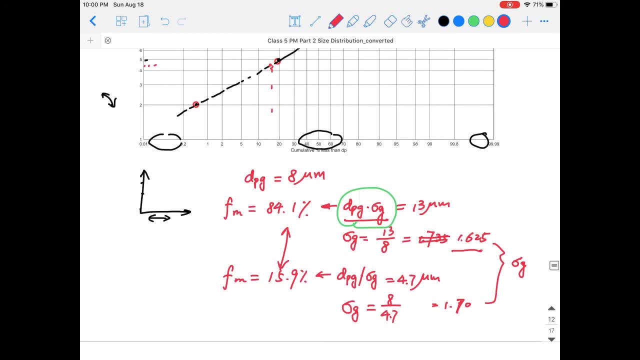 accurate way to do this is actually, since we already have these two equations, let's say equation 1, equation 2. so if we multiply equation 1 by equation 2, what we're going to have is dpg Sigma equal to 13 x 14.7. okay, if we use equation 1 divided by equation 2, that is, 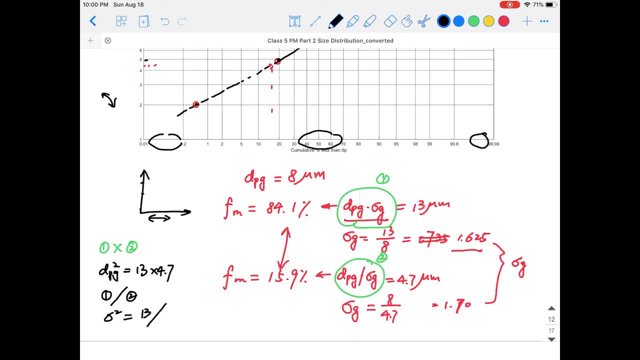 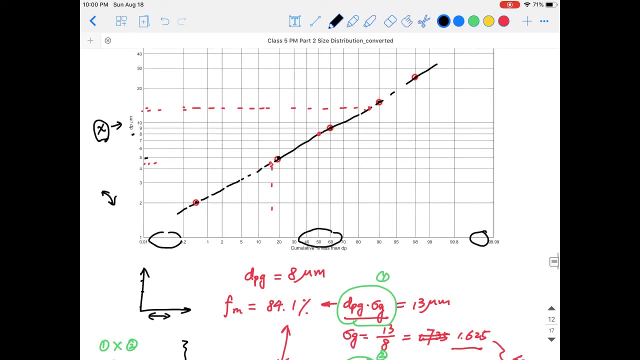 going to be Sigma G, squared equal to 13 x 4.7. okay, so in this way it's a more accurate way and, of course, in the real situation we need to solve the homework or solve the exam problem. we definitely need to use a ruler, right, because this is a lot of. 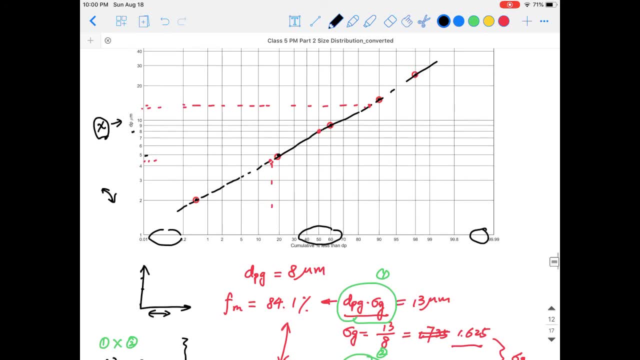 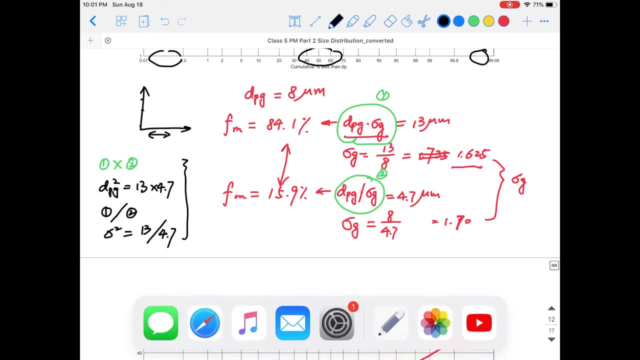 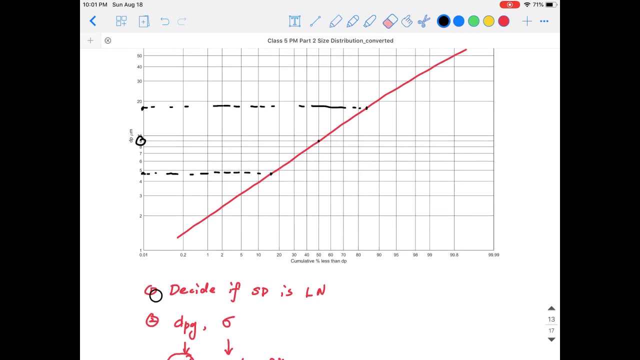 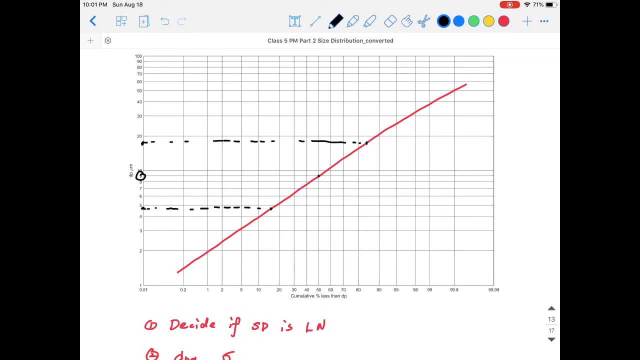 So this is quite objective, depending on where we draw this line here. So basically, what this section tells you is that we can use the semi-log plot to tell us a lot of information regarding the particle size distribution. So first we derive all of those equations to show that we can actually create such a plot to simplify the process of telling whether the size distribution follows the log-normal distribution. 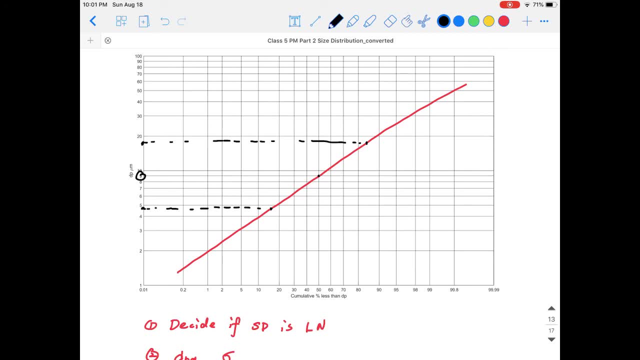 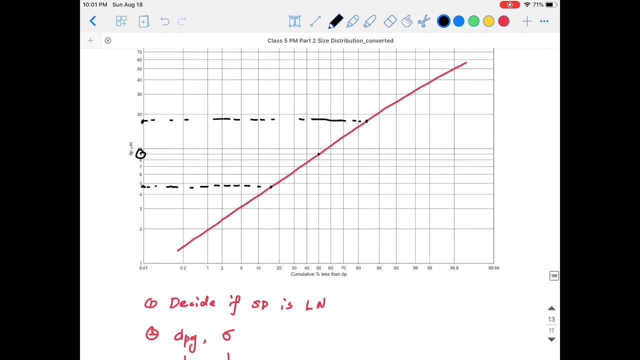 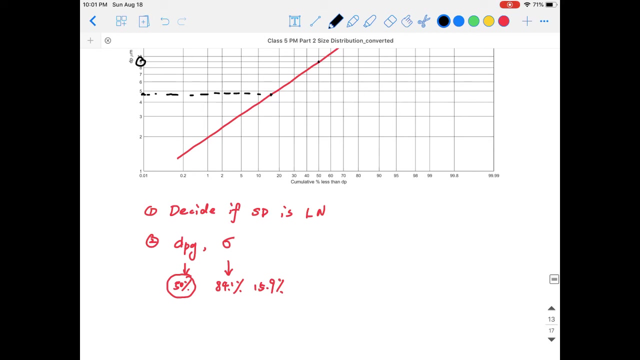 And actually by showing that all the data points follow a straight line and further confirm it follows log-normal distribution, we can further tell more information about the particle sizes. We can easily tell what is the, What is the geometric mean size and what is the sigma g, the standard deviation. 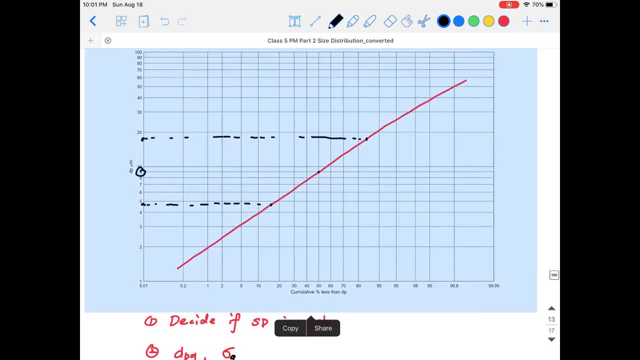 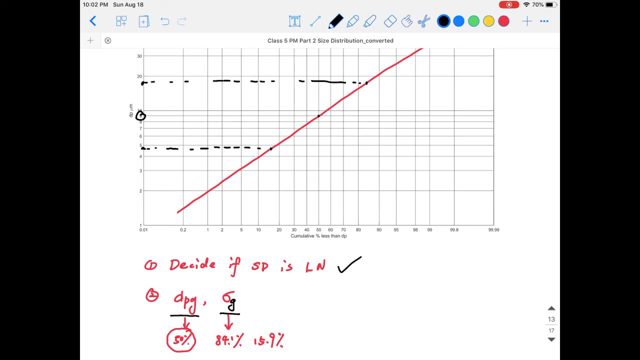 Let's say here I randomly draw another straight line. here, Of course, by using the straight line, it tells us that the size distribution is log-normal distribution. And then let's say: now we want to know where is the DPG? 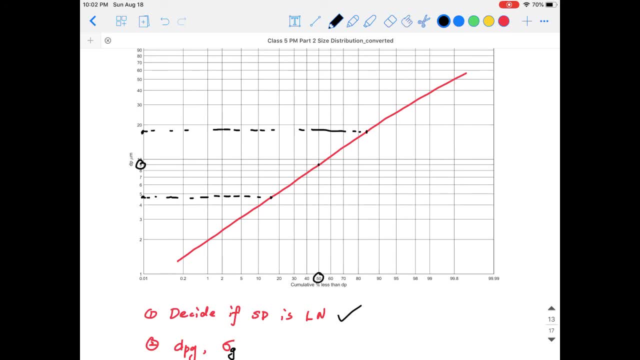 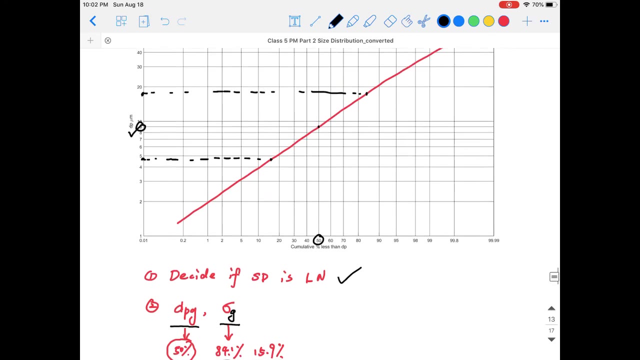 So we first look at the 50% And then We can tell that's 9 micrometer. And then let's say we want to know what is the sigma g. Then we'll find these two data points, That's corresponding to 84.1 and 15.9.. 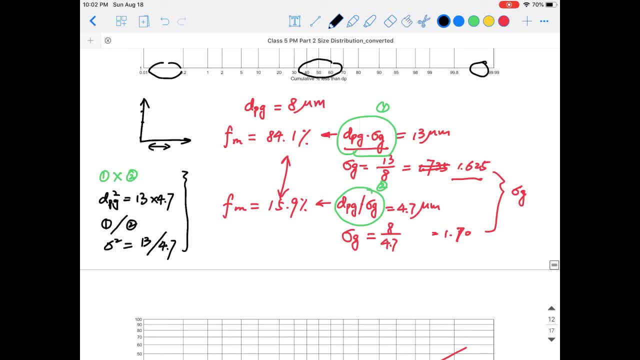 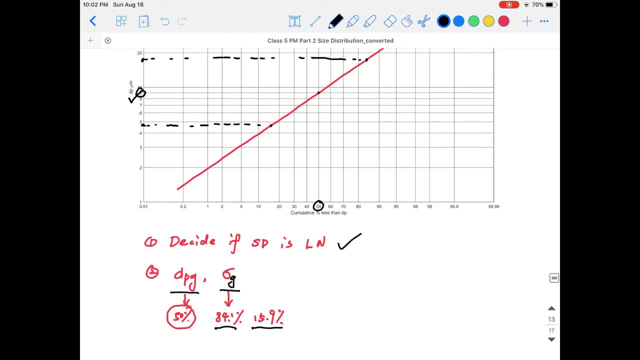 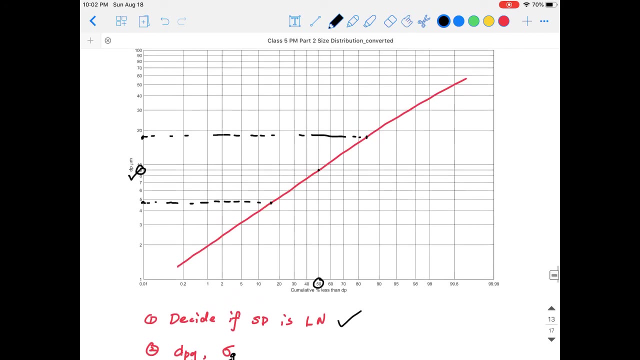 And then we can do this trick to calculate the DPG and sigma g again, And maybe we can compare whether the DPG is the same as the value that we choose from 50%, And what this also means is that We don't really need the straight line. 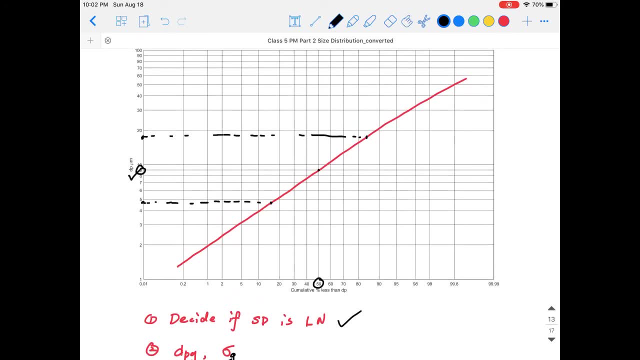 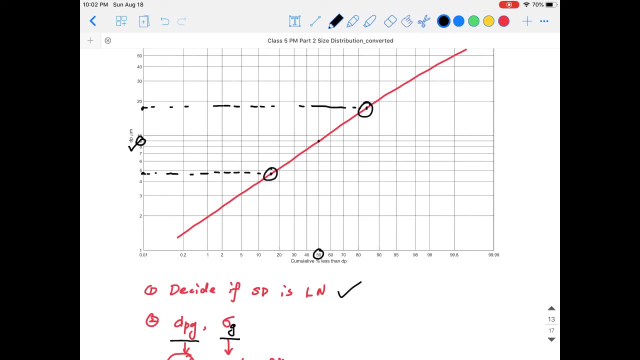 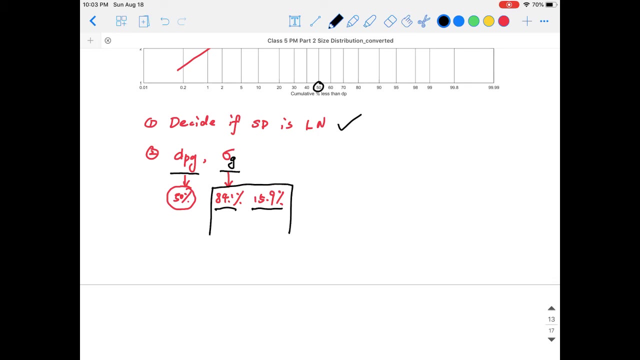 We don't need this graph to tell us what is the geometric mean size. We actually just need these two data points. Let's say, for another example, I just give you the particle size, Or the particle size that has the cumulative mass fraction of 100 micrometer, that has 84.1.. 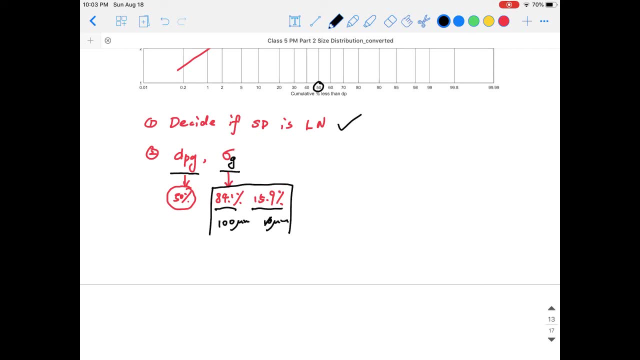 And 10 micrometer. 10 micrometer, Or let's say 1 micrometer, corresponds to the cumulative mass fraction of 15.9 here. So let's calculate what is the DPG. So the DPG will be equal to the square root of these two right. 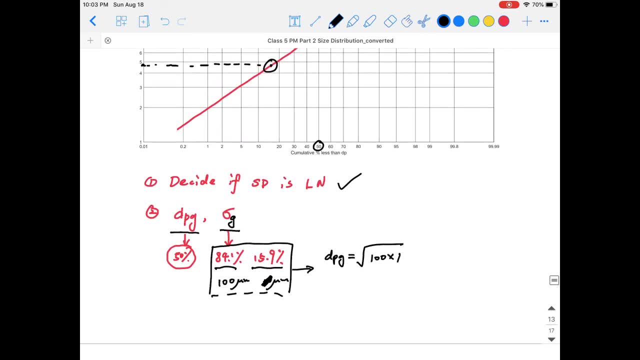 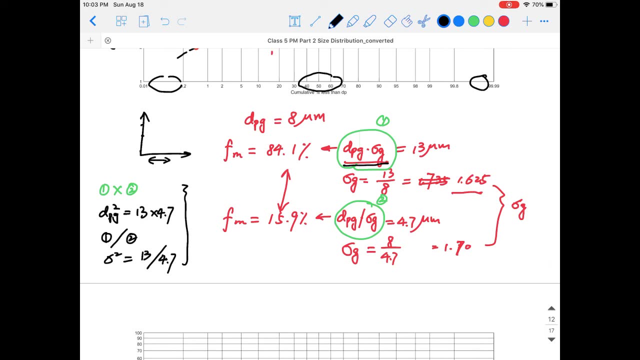 100 multiplied by 1.. Because at 100 micrometer, that is this value here, And at 1 micrometer, that is this value here, And at 1 micrometer, that is this value here, And at 1 micrometer, that is this value here. 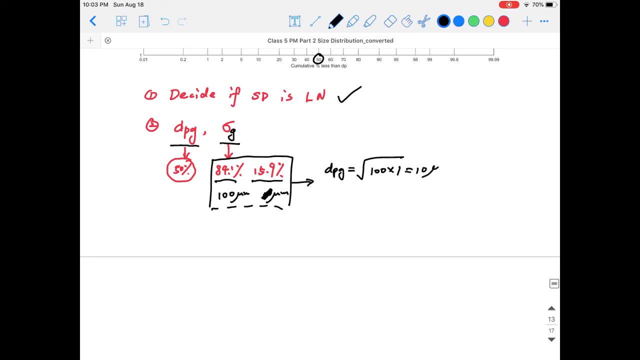 Okay, So this is going to be 10 micrometer And the sigma g is going to be the ratio of these two And unfortunately the ratio of these two is also 100. That is 10.. So this is actually showing a quite broad size distribution. 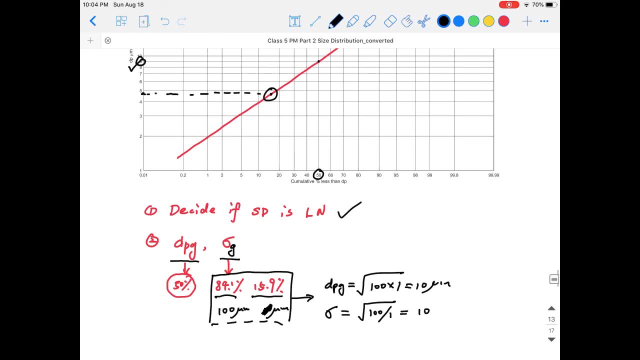 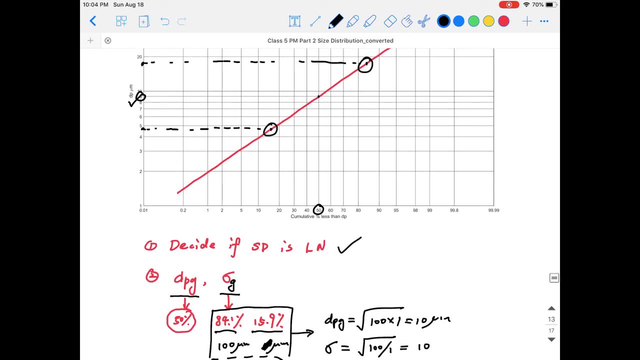 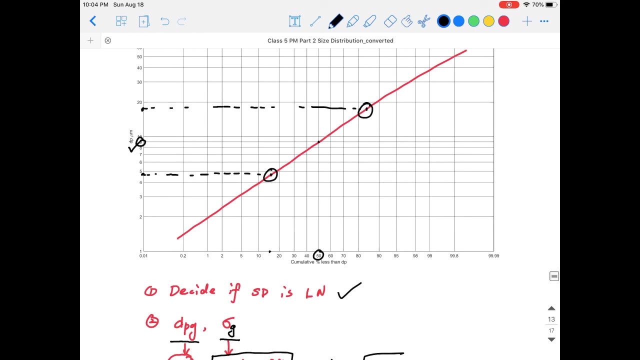 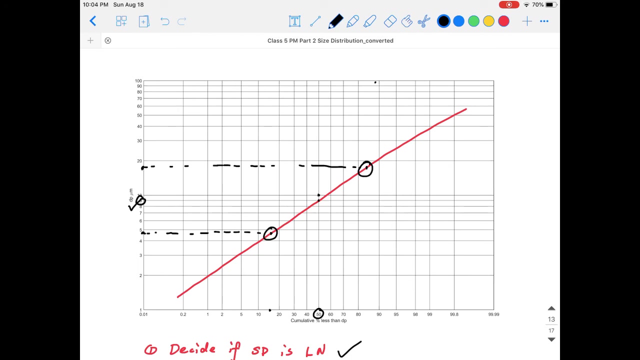 Okay, So if we draw that out, that's going to be somewhere like At 1, it's going to be 15 point, something like this, And here I guess the other point is here: Okay, 100, 84.. 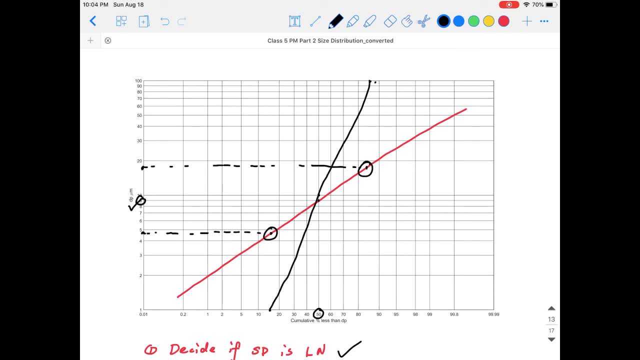 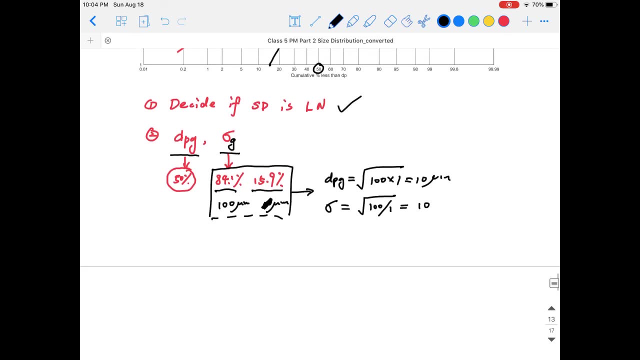 So that's going to be a straight line like this. Of course, in homework you have to use a ruler to do this, And it's not quite easy for me to do this on a computer. Okay, So that's it for this class. 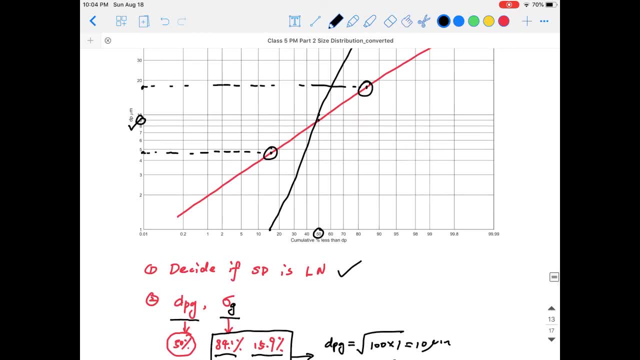 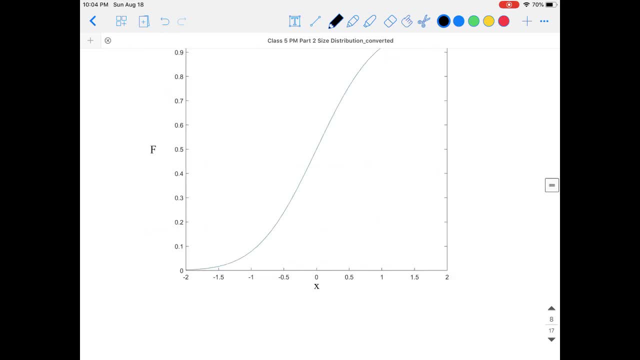 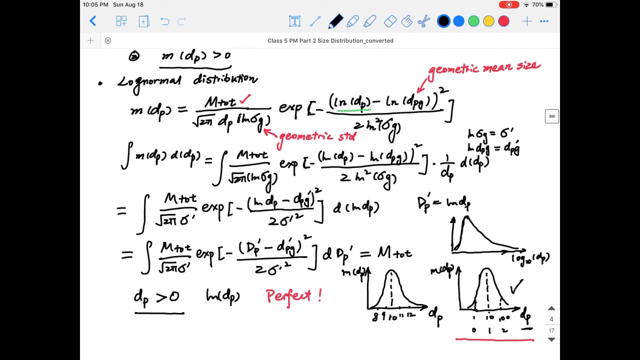 And I know that during the first part we show a lot of equations, But I'm just trying to show that there are many ways we can show the size distribution And what we find out is that we have to use log-norm distribution to describe the size distributions. 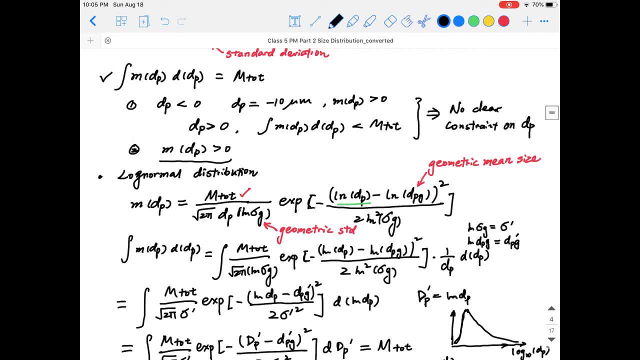 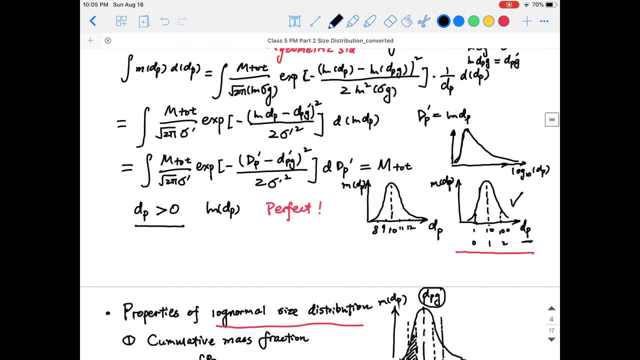 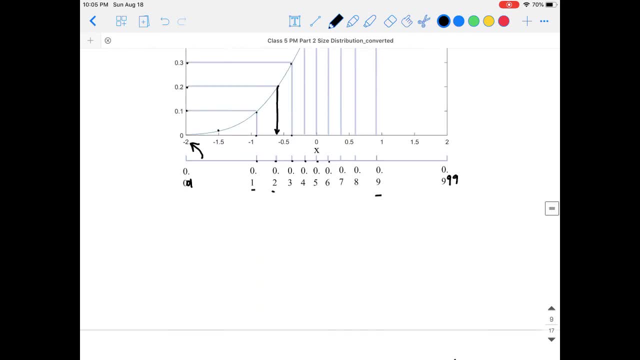 Because the Gaussian actually do not work because of the lack of constraint on the size. And then, by using the definition of the log-norm distribution or the derivation, we show that we can plot the cumulative mass fraction in a more easier way, actually in a linear. 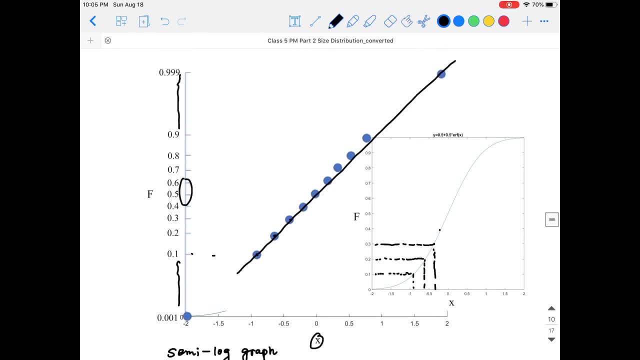 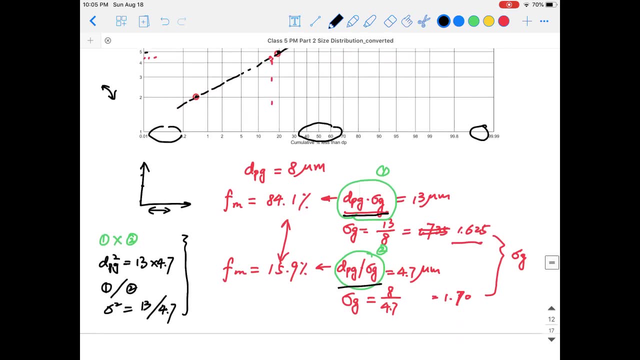 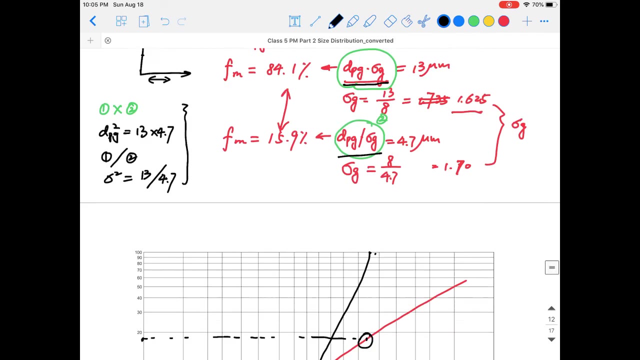 scale so that all the log-norm distributions will be a straight line. here And further, we show that by using this straight line we can tell more information regarding the size distribution by finding out the geometric mean and the geometric standard deviation. Okay, 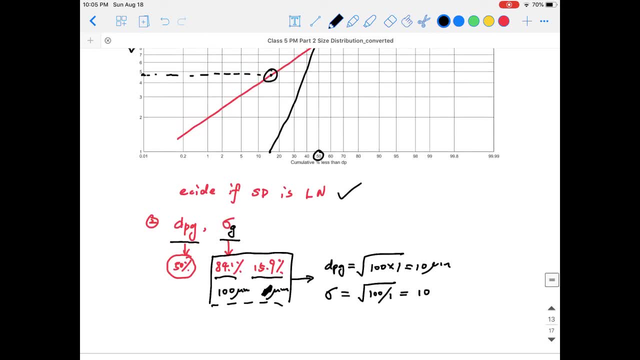 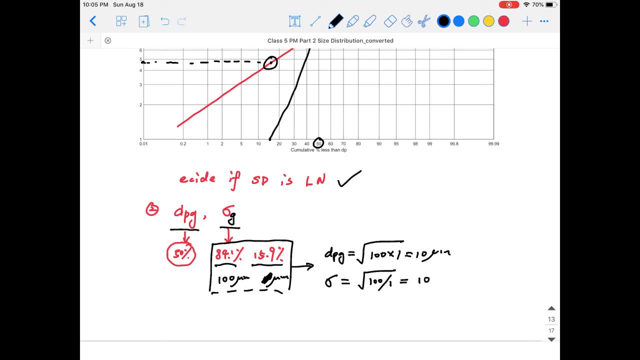 So I'll further post the homework on the canvas And feel free to let me know if you have any questions, Because unfortunately I won't be in my office for this week and the two more weeks. So if you have any questions regarding homework, I can answer them by email or I can even 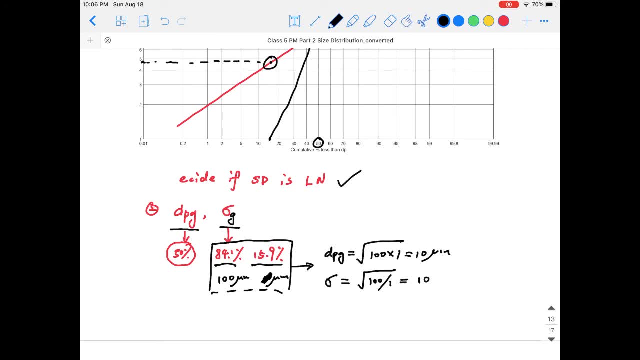 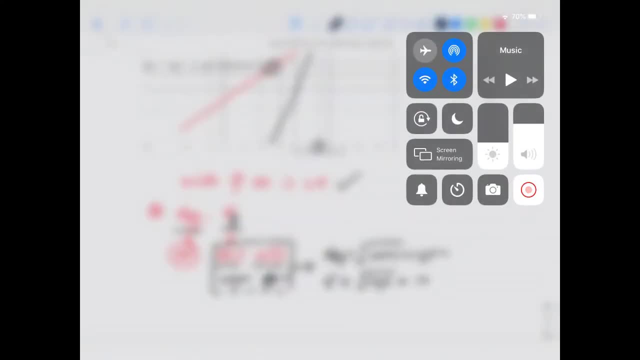 post another video regarding homework problems. Okay, Sorry about that And hope you enjoy the rest of the class. Thank you, Bye, Bye.